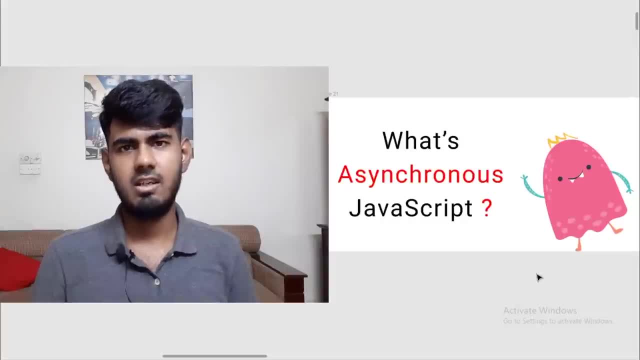 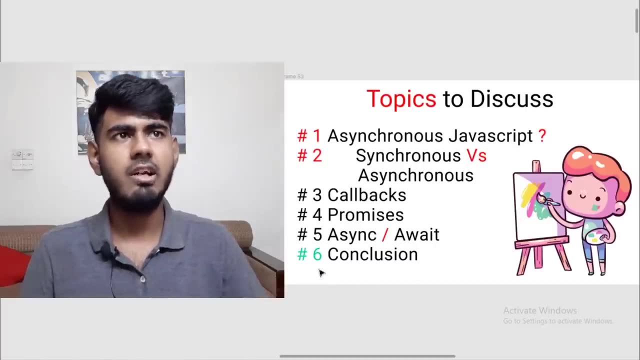 than this is for you. What asynchronous JavaScript does is it allows you to break down bigger projects into smaller tasks And then, using any of these three methods over here, either callbacks, promises or async await- await, along with examples. callbacks- promises- async- await, along with. 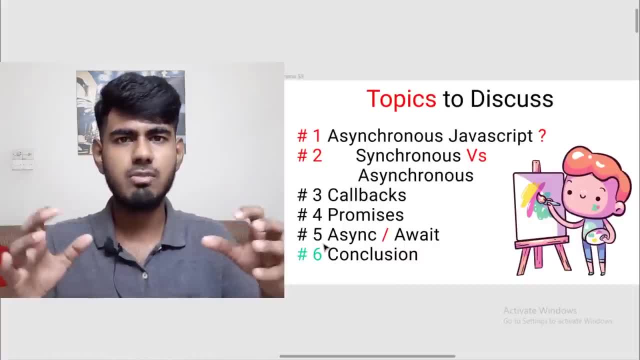 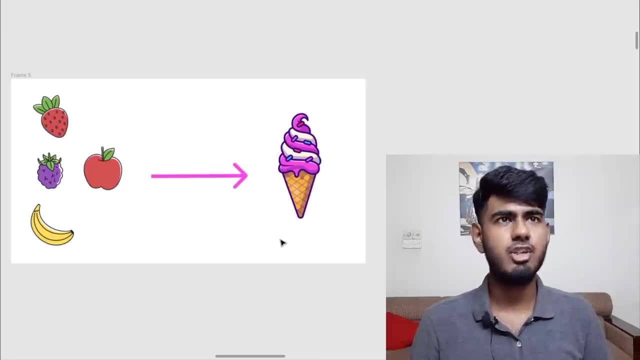 sync await. what you can do is you can form a connection between these small steps in a way that you can get the final result. so here's an example of what I mean. so this is the ice cream that we're gonna make today. here is the ice cream. okay, so using asynchronous JavaScript, we can break it down into. 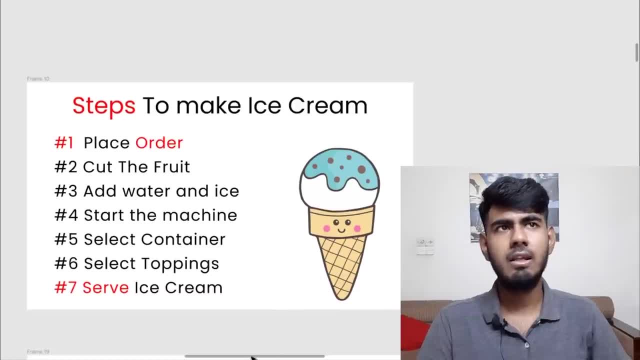 smaller steps. if we do that, it looks something like this: you can see that these are the seven steps to make ice cream. first, starting with the place order, then we're gonna cut the fruits, then we're gonna add water and ice, so on and so forth, and at the very last we're gonna serve ice cream to make you. 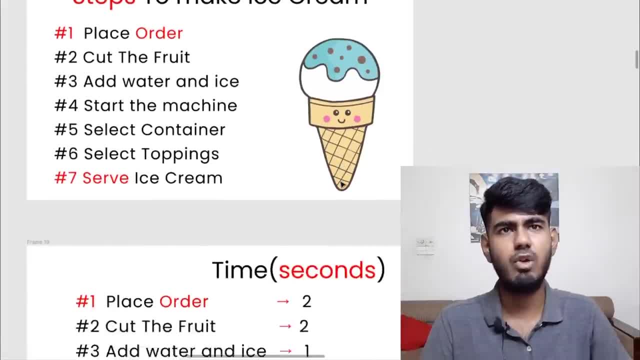 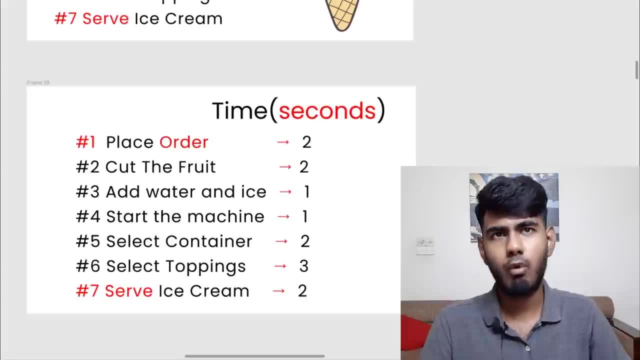 understand this topic even better. I have added some time function as well. you can see this over here: it takes 2 seconds to place the order, 2 seconds to cut the fruit, 1 second to add water and ice, so on and so forth, and at the very last we 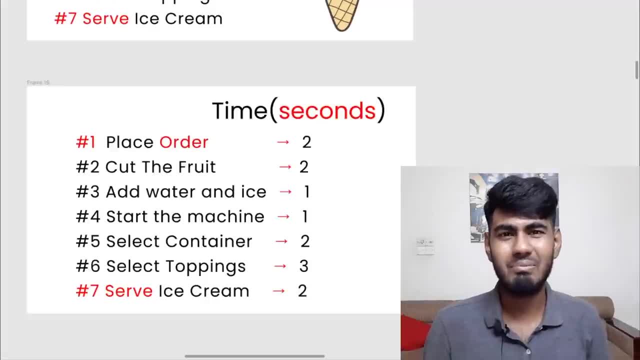 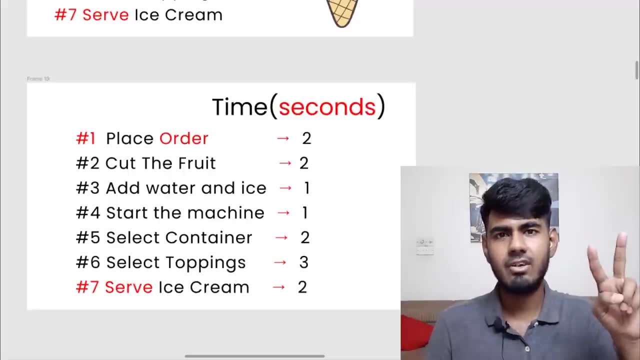 can serve ice cream, take the money and buy ourselves a Lambo- because why not? if you want to learn asynchronous JavaScript better, you need to know the difference between two things: synchronous and asynchronous system. let's start this discussing with the synchronous system. let me explain this to you in clear. 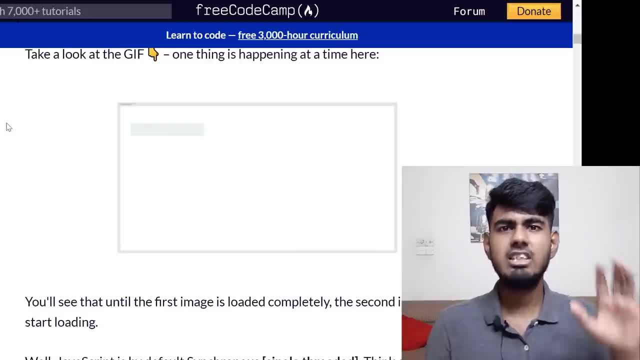 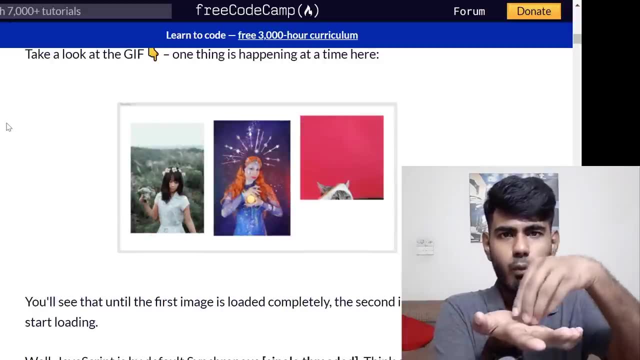 words. let's say that I have given you ten tasks and just one hand. ten tasks, one hand. so how will you do the task? you're gonna do one by one, right, like this: look, one, two, three. so we are in tax number three. right, you cannot jump to the tax. 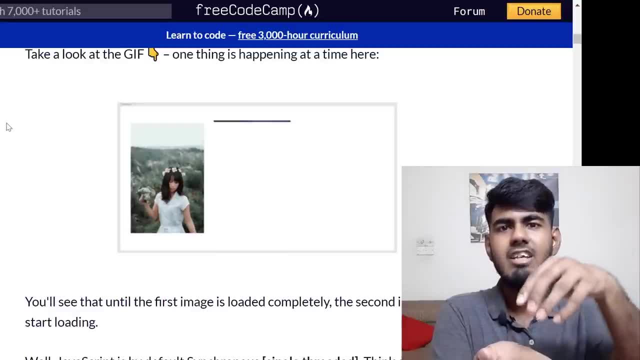 number seven, unless you do four, five, six and then seven, right? so what are you doing? you're doing one by one, right? but you know one by one is Archives and see what exactly does it takes. how are you doing? if it is to the first person is given one task, then remain the same. 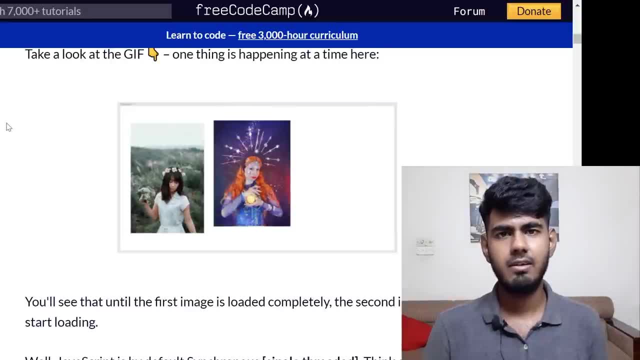 hand. now let's see this one too far apart, because people are working for 10 hands so that we can work any part and 30 tasks in the calendar system. for 10 tasks. you will be given 10 hands, so there you can work independently without. 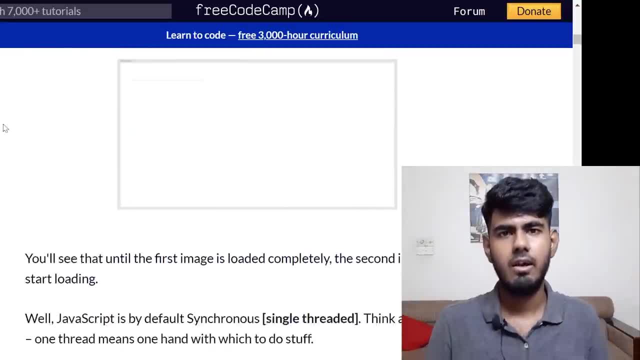 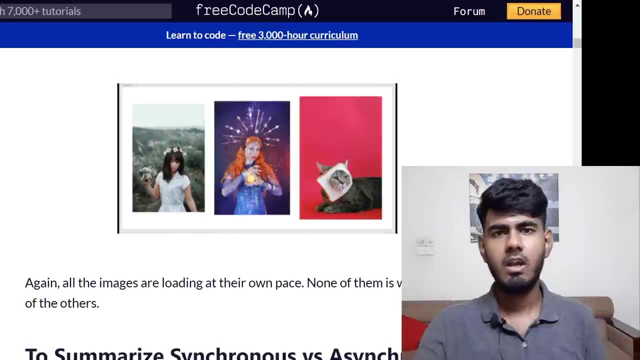 depending on anyone. look at this image. you are here. this is a synchronous system. they are loading one by one. They are loading on their own pace, independently. By the way, I wrote an entire article on the topic that we are gonna discuss today, so that you can understand it better. 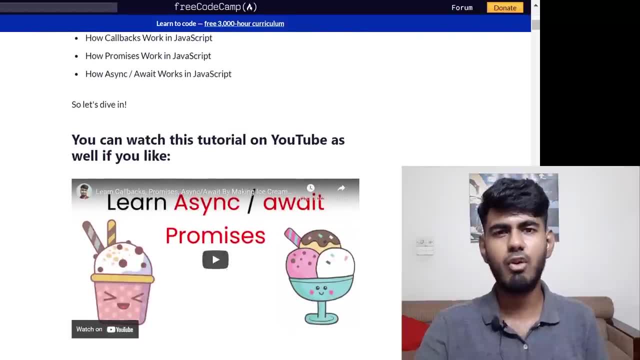 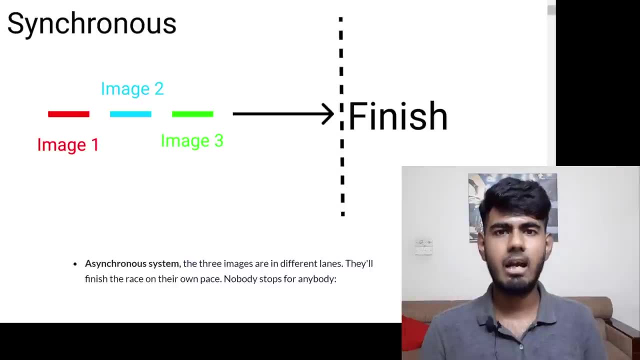 At the same time, you can revise it from here more easily, efficiently and quickly. Link of this article will be given in the description down below. Go and check it out. To summarize, let's say that we are setting up a marathon for three persons. 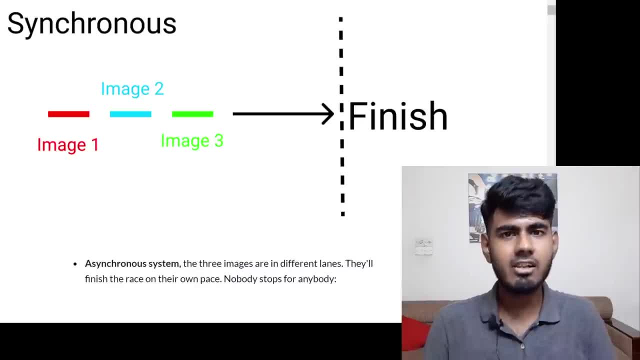 How many persons? Three persons. If you are doing it in the synchronous way, what will happen is you just have one single lane and you have to place those three persons on this single lane in the serial of 1,2,3, and the rule is: nobody can overtake the other. 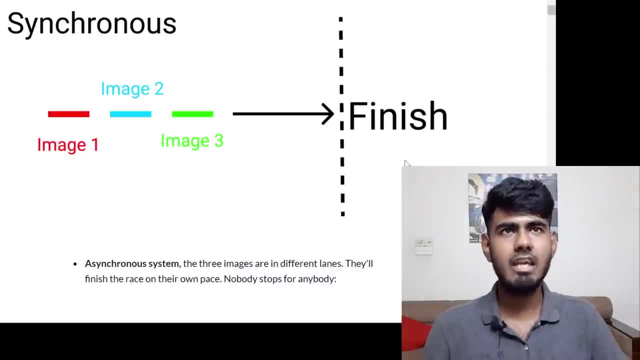 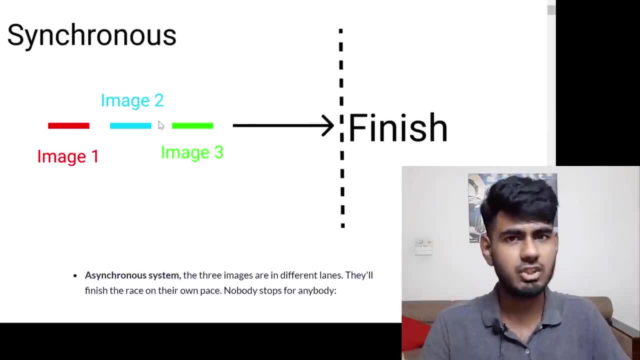 Everyone has to finish the race one by one. Look at this image over here. This is the synchronous system. This is the finish line over here and the images, which is the persons 1,2,3 are standing on the same lane. Which lane? 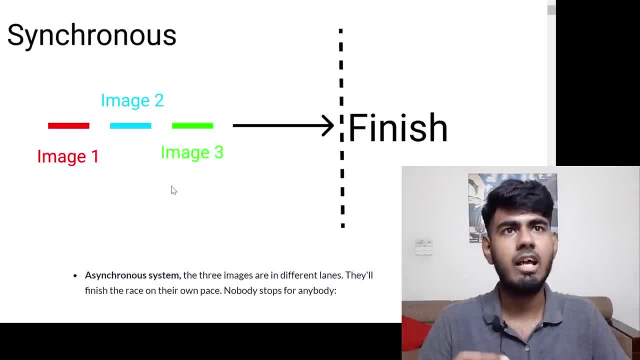 Same lane And nobody can overtake the other. Everyone has to finish the race one by one. So the person 3 or the image 3 will finish the race first, then the second one and the first one. Like this, The single lane. 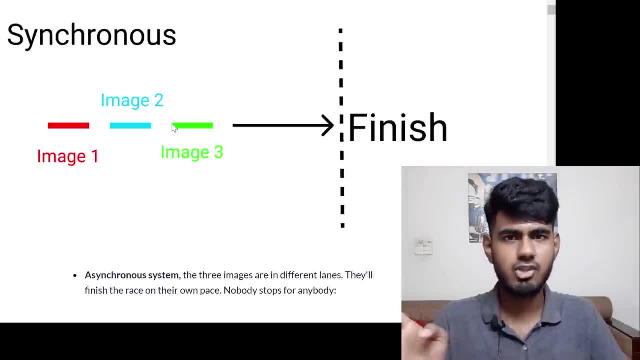 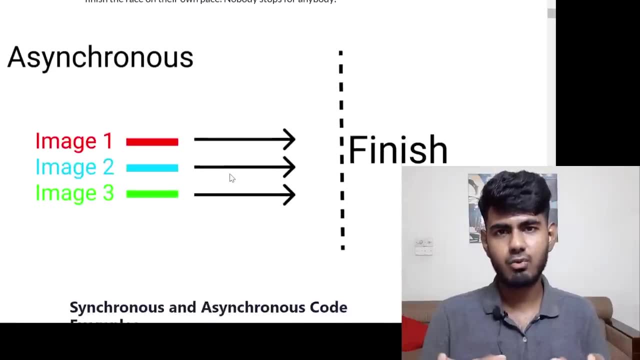 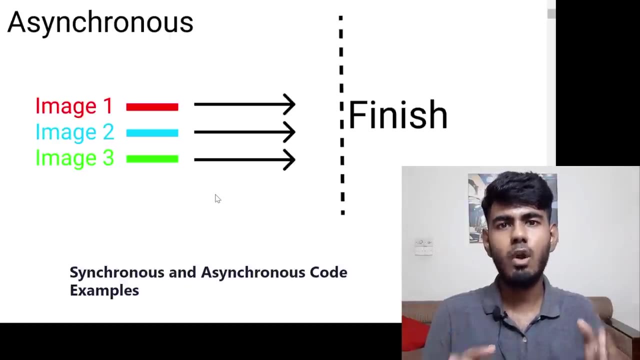 The synchronous system. If anyone stops, the entire process stops. If the image 3 stops over here, then everyone has to stop, And if we are setting the marathon in an asynchronous way for three persons, we will have three lanes. If we have more participants, then the number of lanes will increase. 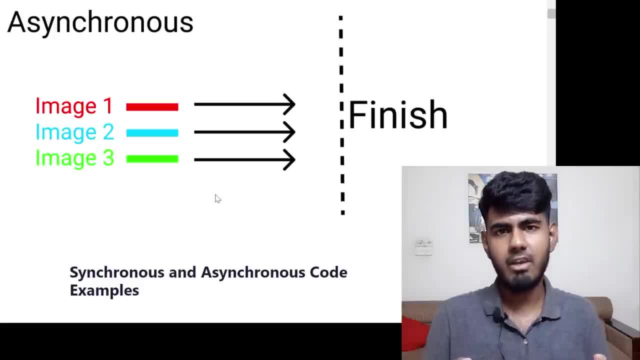 Which means that nobody stops for anyone. They can finish the race independently on their own pace. If anyone stops, then the system still continues to run. Look at this image over here: This is the finish line and this is the participants over here and these are the lanes. 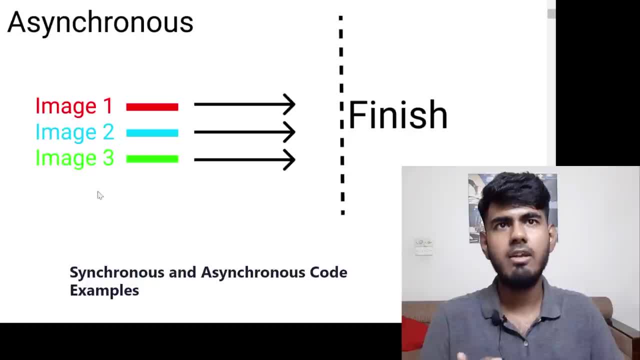 Lane number 1, 2 and 3.. The image 1, 2 and 3.. They are gonna finish the race on their own pace. I hope you understand the difference between the synchronous and asynchronous system. Let's look at some examples right now. 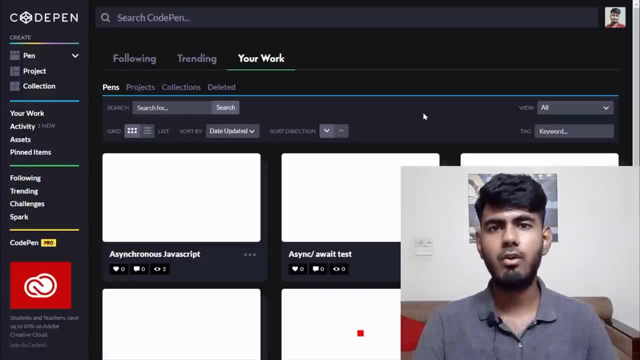 You can use any code editor you want, but for this tutorial I'm gonna write it on CodePen because it has a simple interface, So you can follow along with me if you want. So open codepenio and then you click this pen over here. 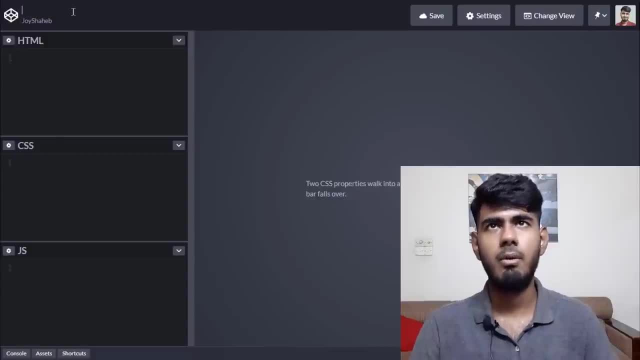 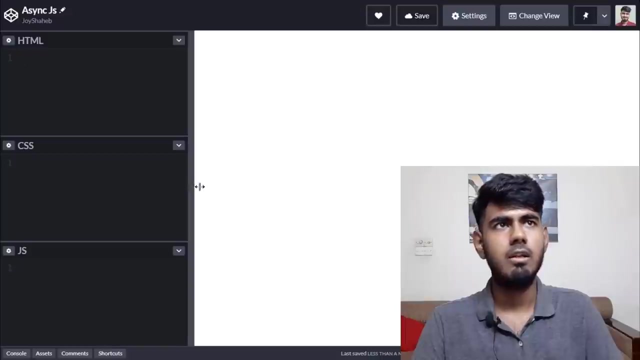 Then you're gonna click this small pen icon over here and you're gonna name this project anything you want. I'm gonna write it asyncjs. And then you save it. Ctrl S, Like this Ctrl S. And now you're gonna drag it in the middle like this, and double click on the JavaScript. 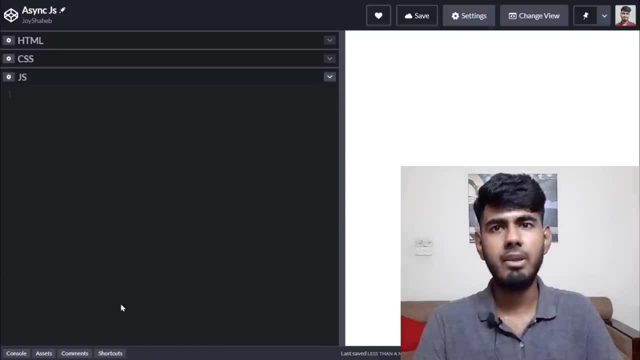 section like this and it's gonna expand. And in order to open the console, you're gonna click this small icon over here. You can see that, Like this, Double click on here and it's gonna expand like this. We need to know. 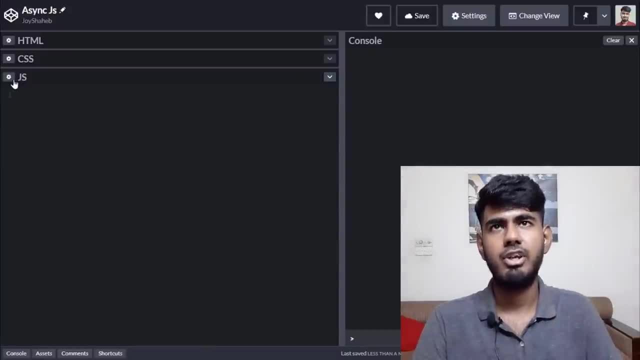 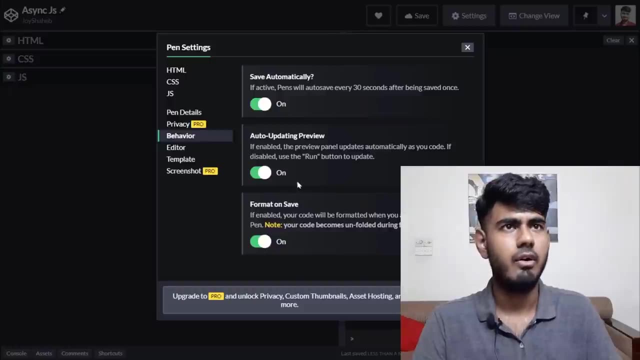 We need to do one more setting You come over here, this small gear icon over here, click it, click on behavior and you enable everything Except this one: the auto updating preview. Okay, Turn it off, Save and close, And then we're gonna manually get a run button over here. 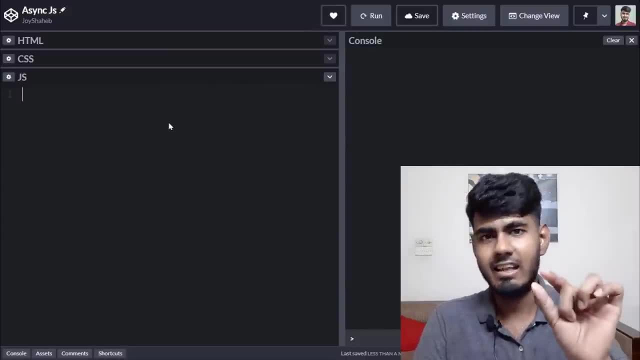 Why is that? That's because every time we write a single letter, codepen runs it automatically, which means that every time we write a single letter, we're gonna get an error after error after error. In order to avoid that, I have turned off the setting. 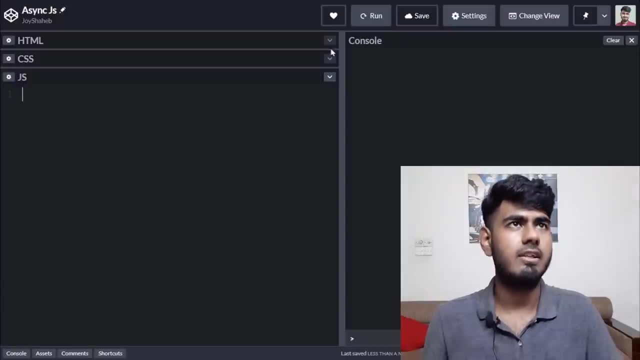 Every time we finish writing our code, we can manually run it like this: Okay, Now let's look at the synchronous system example. So we're here, You write synchronous- S-Y-N-C-H-R-O-N-O-U-S, synchronous, like this, and you comment this like this: 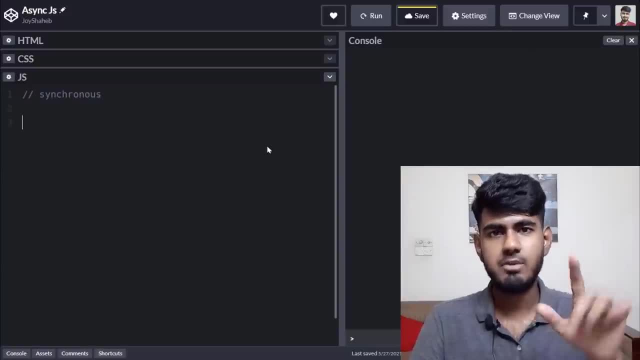 And over here we're gonna write console dot log five times. How many times? Five times? like this: Follow me: Console dot log. brackets, double quotes, space over here. Okay, You copy this, control C and then control V five times. 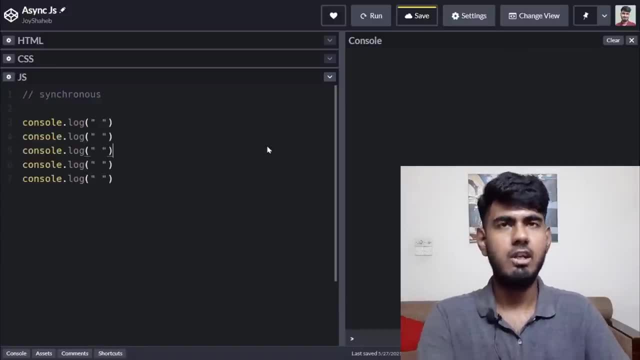 Okay, Four, five. Keep some gap over here as well. Additional gaps, um, like this, All right, So over here we're gonna write a full sentence. Okay, I eat ice cream with a spoon, So we're gonna divide it by phrases. 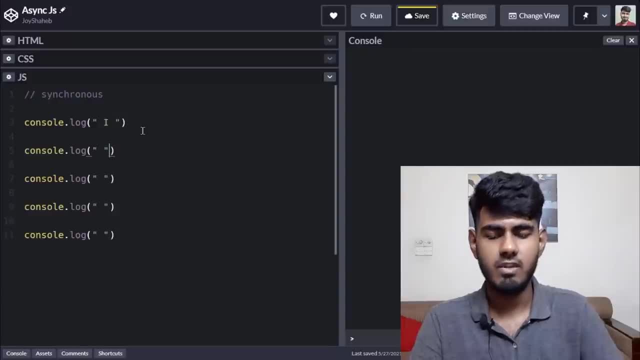 Okay, Then follow me along. I eat ice cream with- oh sorry, a spoon. Okay, I eat ice cream with a spoon. Okay, Control S to save it, And then you're gonna click this, run over here, And then we're gonna get the result. 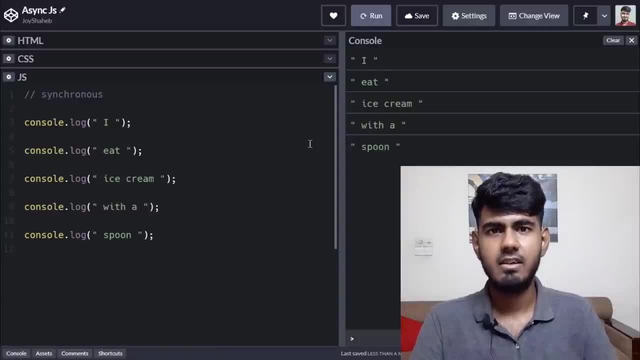 There we go. You can see that our phrases are printed one by one, serial. That's because JavaScript runs from the top to the bottom. How does JavaScript run from the top to the bottom Serially in this process? if anyone gets stuck, then the entire process. 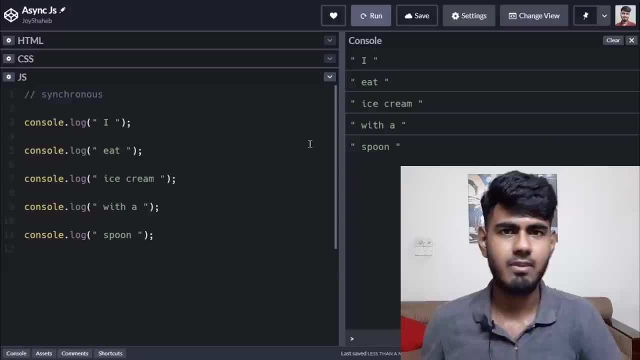 Get stuck. This is the synchronous system. If you change the serial, let's say that I want to change the spoon from here to here. Okay, Control X, And then you paste it over here. Control V, control S. you clear this console over here. 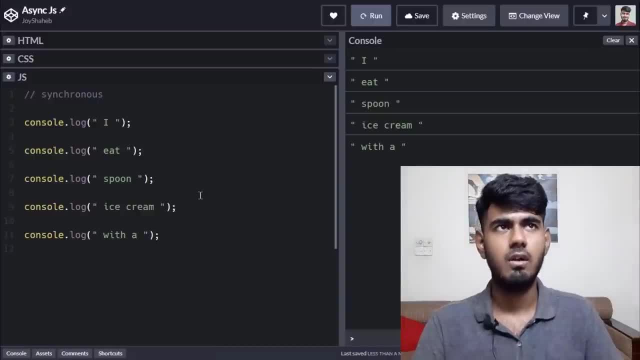 And then you run it again. Let's see what. let's see the result. Now you can see that I eat spoon ice cream with a. you see that JavaScript doesn't care about anything. It's gonna run the code from the top. 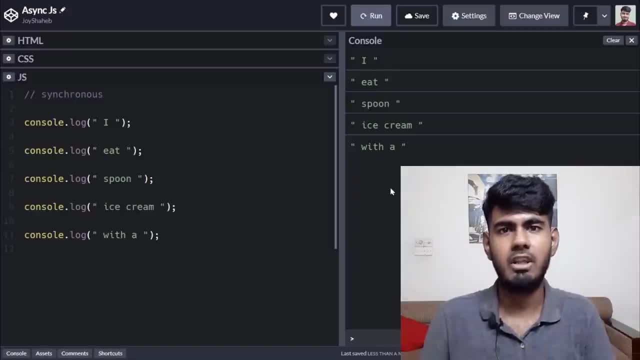 To the bottom. This is what the synchronous system. Now let's look at the asynchronous system Now over here. right, Asynchronous, Okay, A synchronous done. Clear the console over here. You change the serial control X, Okay, And we're here. 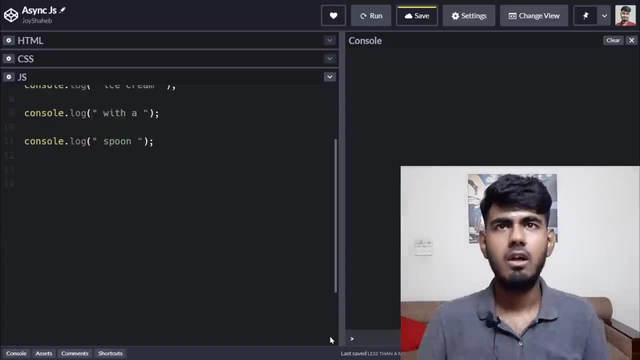 Control V, control S. And now come over here at the bottom. I need to make you understand a small function named set timeout function, which is a built-in function of JavaScript. What this does is it allows you to run a function after a specific amount of time. 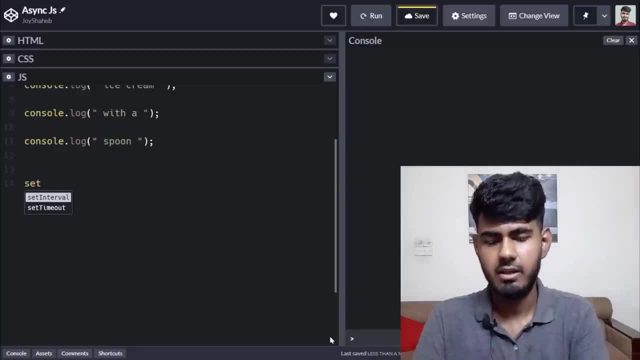 So you write set timeout, set, then capital letter, T timeout, this one, okay, Then brackets. The first thing that we are going to pass as an argument is a function, So we're going to use the arrow function. Don't worry, I'm going to explain arrow function and the regular function. 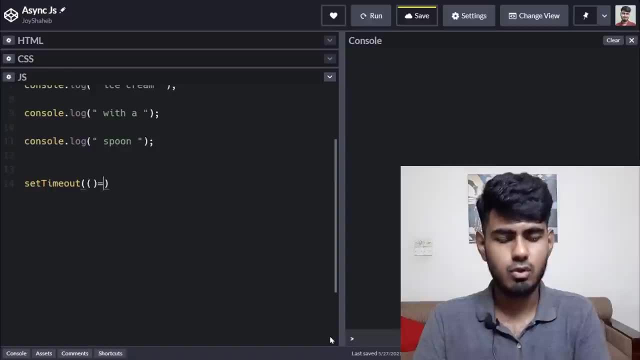 We write the arrow function like this: Okay, Equal to This side: curly braces. Now let's look at the difference between function- the regular one- and the arrow function. Okay, In the regular way, we write a function like this: first the function keyword: 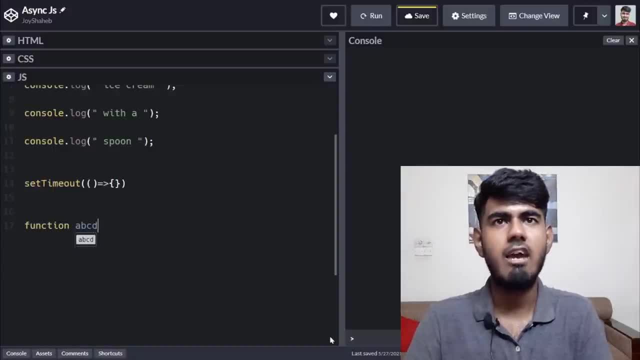 Okay, Then we're going to name it like this: A, B, C, D, E, F, G, However you like, right, Then you put that, then you put that bracket like this: Okay, And then curly braces. This is the regular function, but in the arrow function, how we write it is we're going to. 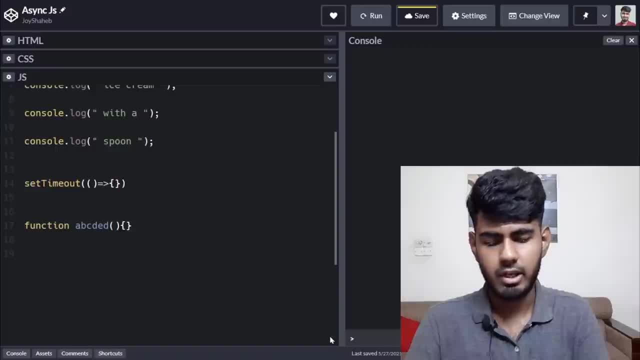 write either Let, var or const, Okay, Like this. And then we're going to put the name over here. What was the name of this function? A, B, C, D, E, D, right? So we're going to write A, B, C, D, E, D, which is the name of that function, like this, like: 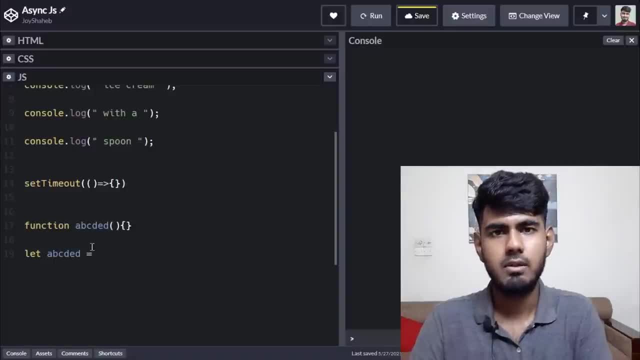 this and that equal to, and then we're going to put brackets over here, And then this sign over here, the arrow side, and then curly braces on the regular function. we used to put Our arguments on this bracket, like A, B, C, D et cetera. 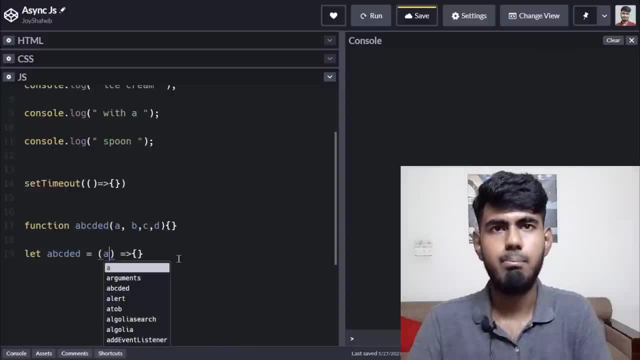 In the arrow function. we place our arguments over here: A, B- sorry- B, C, D, et cetera. I hope you understood the difference between two. for this project I'm going to use the arrow function, Okay. 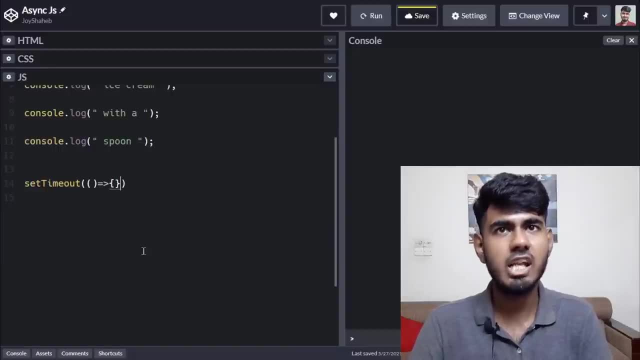 The latter one, this one. So, once we have entered the function inside the set timeout as an argument, the next thing that we're going to put Is the time. Okay, So it is actually counted as milliseconds. If we write, 1000 is going to count as millisecond, which means one second. 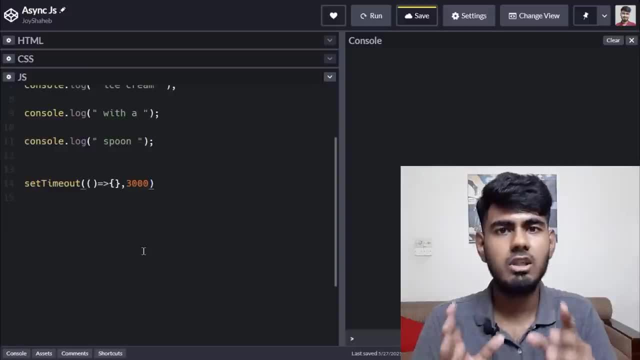 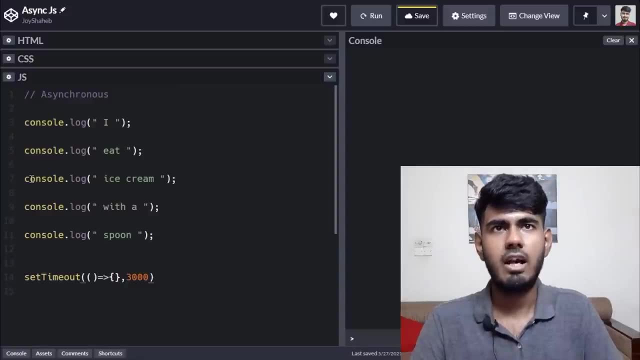 So if we write, let's say, 3000,, it means 3000 milliseconds, which means three seconds. Okay, Now come over here. Let's say that I want to cut this and place it inside the set timeout function. How will you do it? 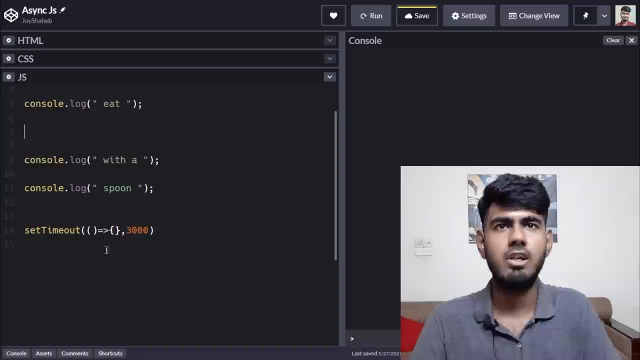 We'll cut it like this: control X, And then inside over here, this curly braces. we're going to place it over here. Okay, Control V, And now let's change it to four seconds. By the way, set timeout is a asynchronous function. 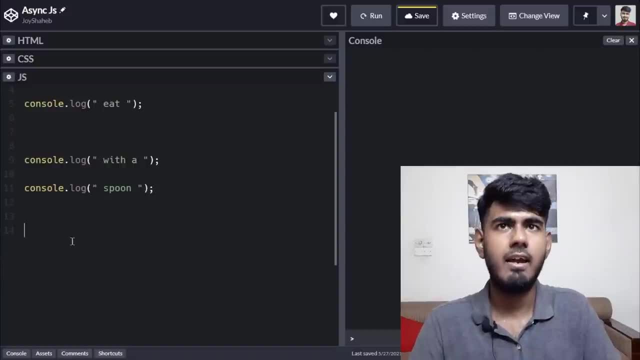 Okay, You cut this from here, control X, and you paste it over here Control V, like this control S, to save it, And then we're going to press this run function. But before that, do you remember what I told you? 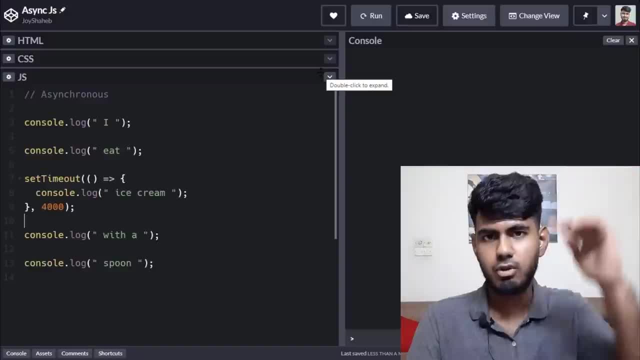 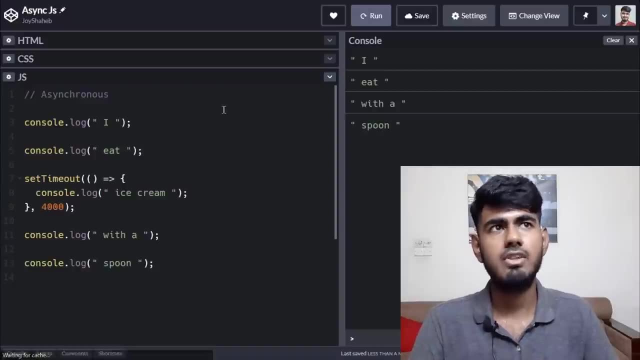 JavaScript runs from the top to the bottom. how? from the top to the bottom, And let's see how this works. Okay, So we're going to run it like this and let's see the result. Now you can see that we have got. I eat with a spoon. 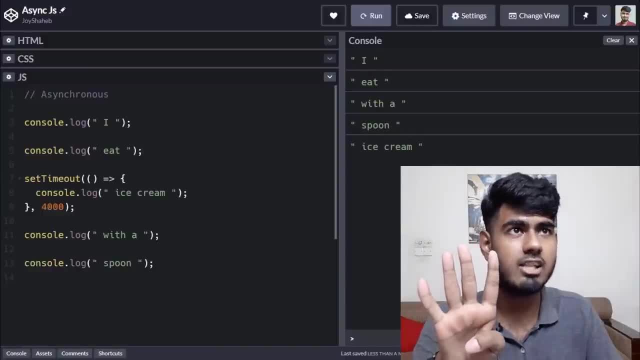 And then after how many seconds? after four seconds, we got the ice cream over here. Now, how does this system work? This is an asynchronous system. Okay, Asynchronous system. Look, the cereal is over here. Okay, I eat ice cream with a spoon. 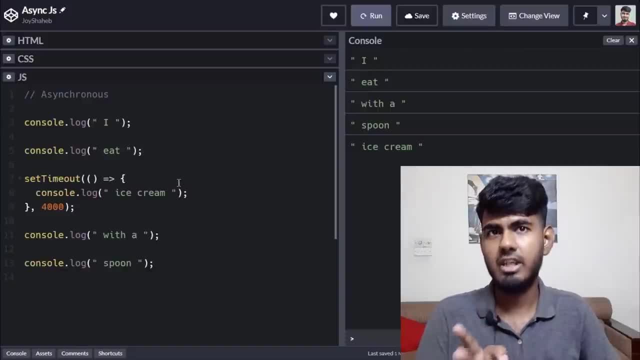 The cereal is over here as well. You can see that I eat ice cream with a spoon. The system is actually working like this: Look I eat, And then this ice cream over here. it has a set timeout function, which means that we're. 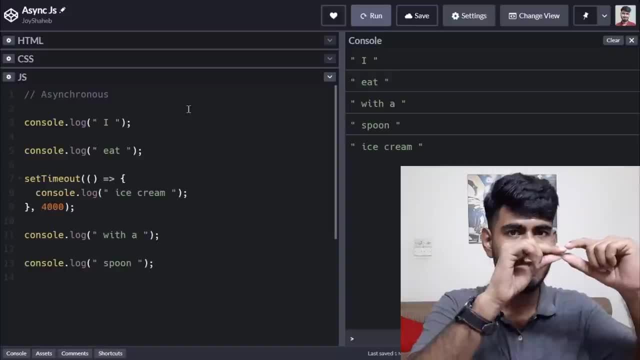 going to have another hand over here, is going to take this function at the side, which is our second lane. Okay, This is our main lane. I mean main road. this is the secondary road. It is taking that asynchronous call at this hand. 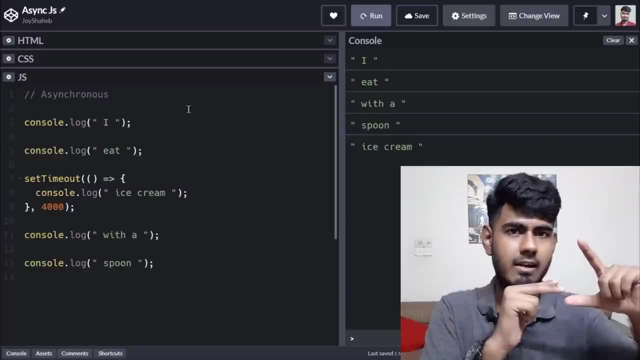 And after four seconds, it's going to release it on our main lane like this. Until then, what will happen? I eat ice cream is an asynchronous call, which means that it's going to take it over here. After four seconds it's going to get released. 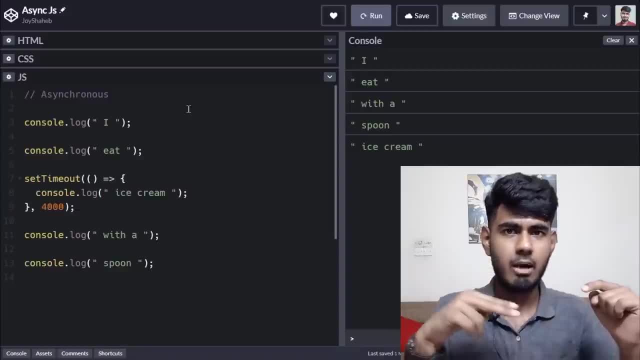 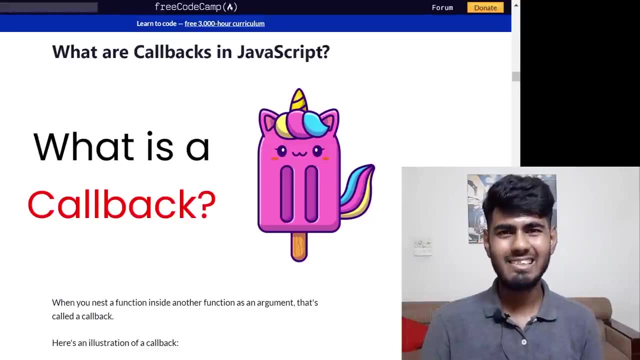 Then with a spoon, after four seconds it's going to come over here. So this is how the asynchronous system works. I hope you understood it. Now we're going to start our discussion with callbacks, But before that, if you're new to the channel, feel free to subscribe, because I post videos. 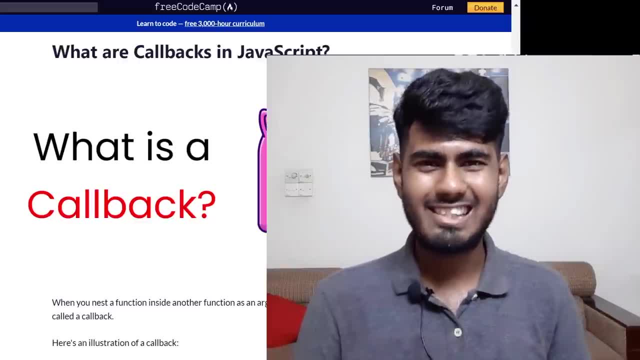 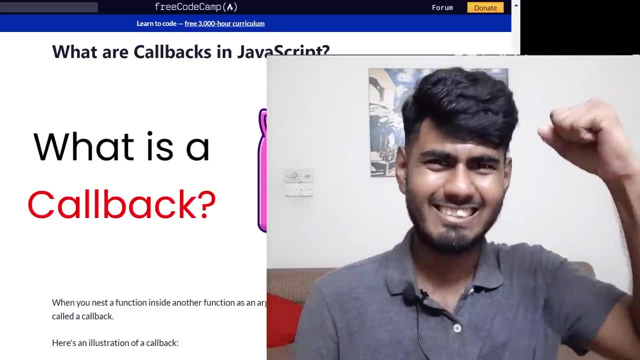 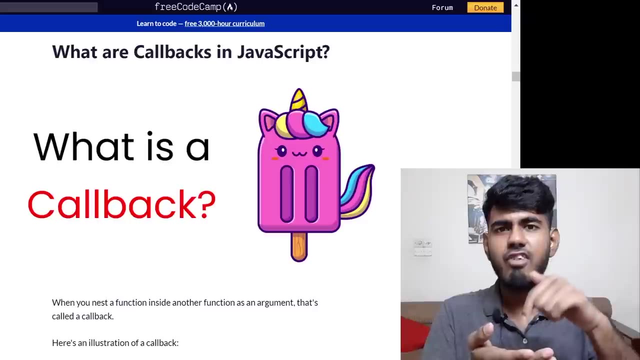 based on practical web dev projects So that you can level up your coding skills. If that sounds interesting, hit the subscribe button and join my gang into the further ado. Let's get started. Let's talk about callbacks. What are they in simple terms, very simple terms: calling a function inside another function. 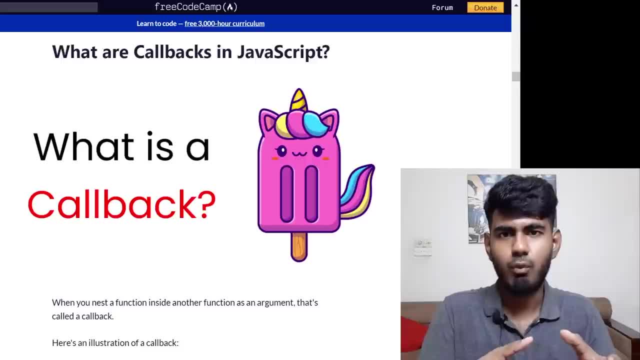 is called a callback. In even more simple terms, what it does is: it forms connection between what functions. Let's look at one example with callbacks. And then we're going to start our ice cream. Okay, Let's start our ice cream business. 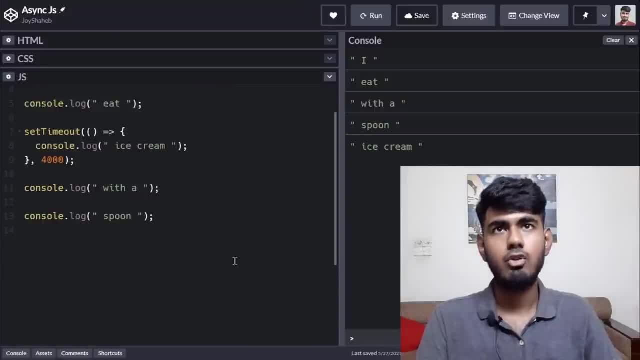 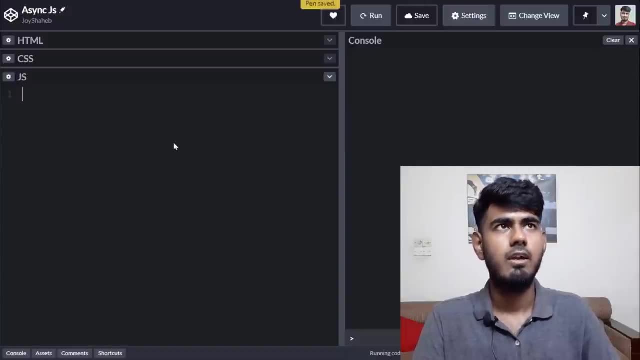 Okay. Now back to CodePen. You delete everything, Okay. Control a, then delete. Okay, You cleared the console over here as well. Control s Okay. So what did I tell you before? callbacks means calling a function inside another function. 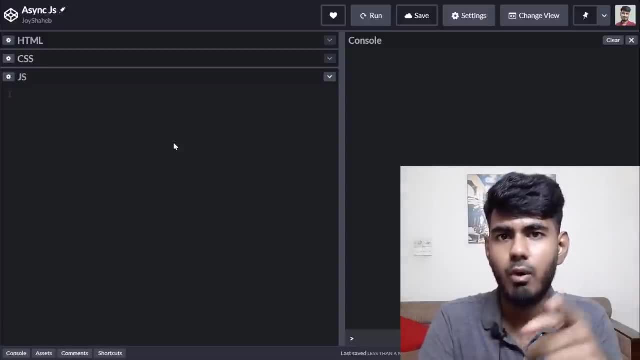 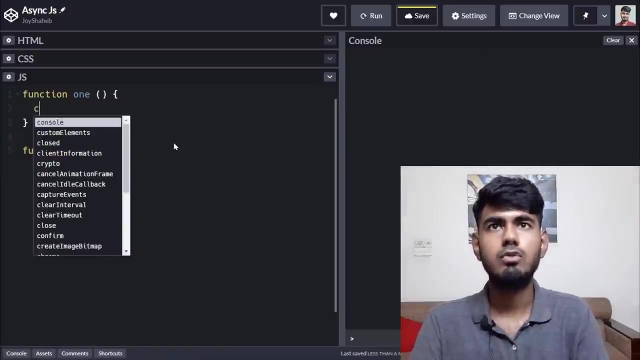 So we will create two functions to form the relationship. What relationship? Okay, Function one. function to like this. function one: Okay, We're going to use the regular function. Nothing complicated, No politics here. Okay. Function two: Okay, Now, inside function one, what we're going to write is consolelog. 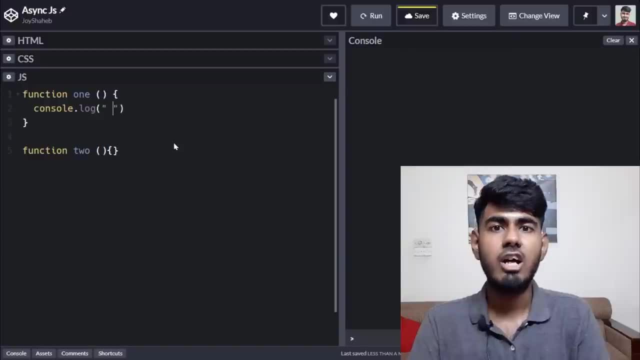 Okay, Consolelog. Over here we're going to write function one. or let's write step one: Okay, Step One. Oh, sorry, Like this Step one. Inside over here We're going to write consolelog Step two. 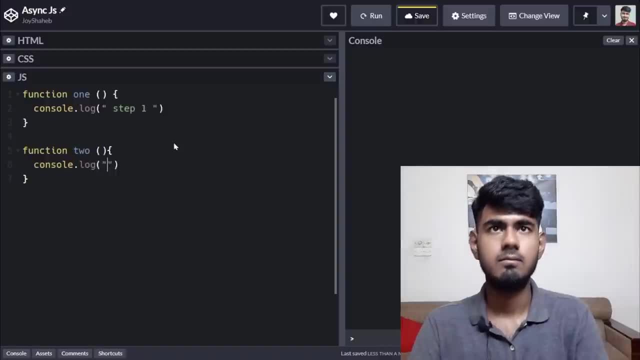 Okay, like this in order to run this function. what do we do? we write the name of the function at the bottom like this: look, we call it like this. one then brackets over here: ctrl s. you run this button over here after you clear the console. okay, run it like this and we're gonna see step one on the 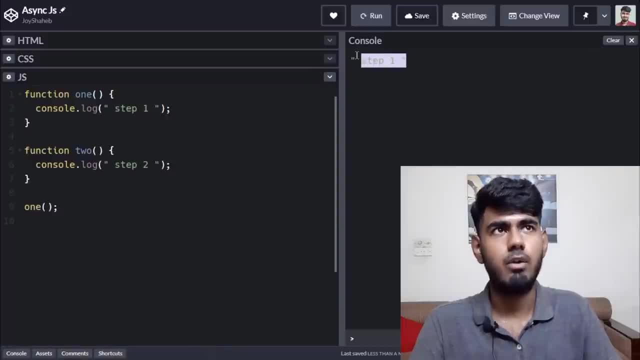 console. let's wait. ah, there we go. this is step one. okay, and how do we call the function two in the same process? we write it over here. i mean, we call it over here like this: okay, ctrl s. don't forget to clear the console over here. clear it like this, and then you press this run button. 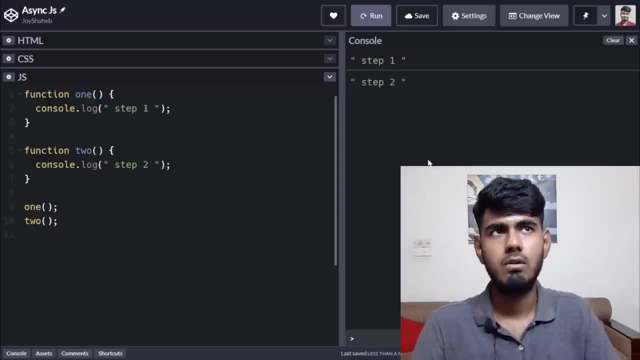 now you can see that we have step one, step two. that's because we have an order right. javascript runs from the top to the bottom. look which one is first. one is first and then two. but if we reverse the order, if i write two first and then one, like this, ctrl x, ctrl v, like this, so 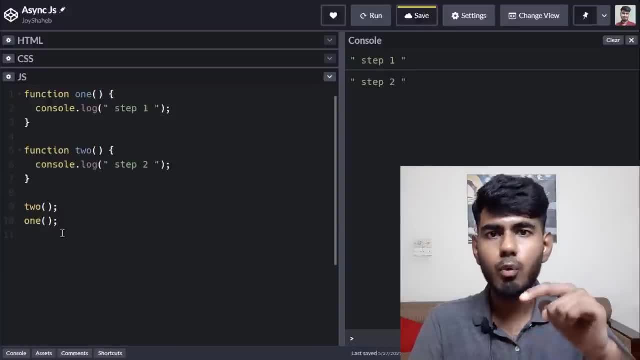 first is two and then one. so what will happen? two will run first and then one. clear the console, save it, run it. you can see that we have step two first and then step one. these are regular functions. now let's form a relationship between these two using a callback. what a callback, okay. 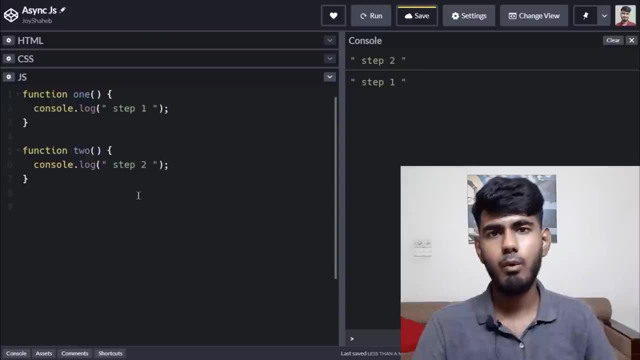 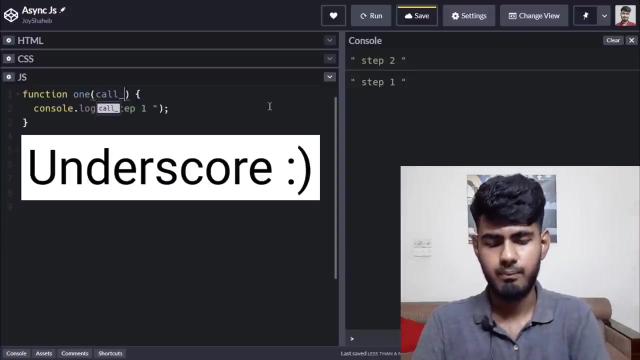 let's remove this. okay, now we're gonna make a connection of function two inside function one. so how do you do it? we do it using a argument. we're gonna write over here: call two, c, a, double l hyphen, okay, two. this is nothing, this is just an argument. okay, nothing else. and over here we're gonna write: step one complete. 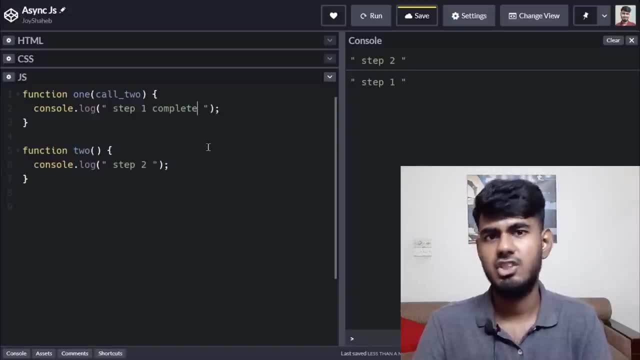 okay, this is nothing special, this is just gonna get printed on our console. okay, please call step two like this, okay, oh, like this. now, in order to provoke function two, what we do is we take this argument over here, call two and then, as number two, function is a function. 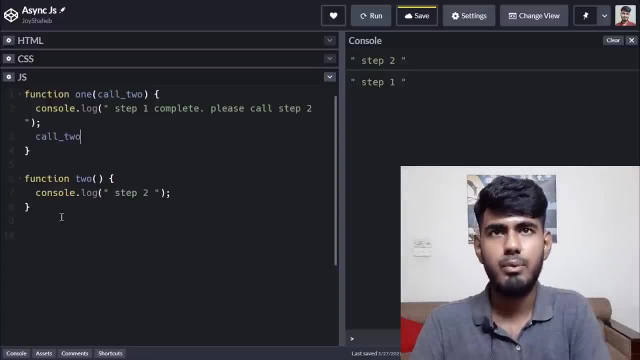 what we're gonna write is: we're gonna give brackets over here like this: and now it's gonna call it every time once our consolelog is printed like this: look, we don't have to call two anymore, we just call one, one. and then inside over here, we're gonna pass function number two. which one function. 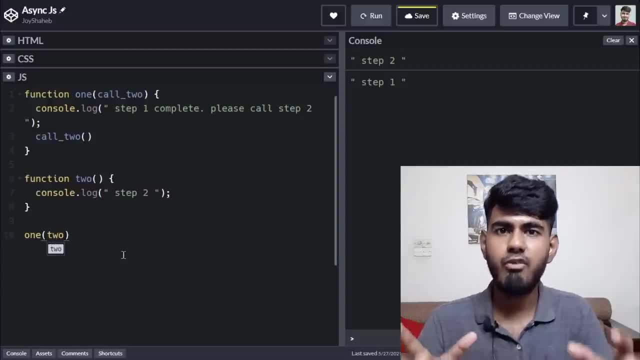 number two. okay, two like this. look how did i form a relationship between these two. if you clear the console, save it, run it, let's see the result. look what is happening. step one: complete. please call step two, and then we have the step two. if you remember java. 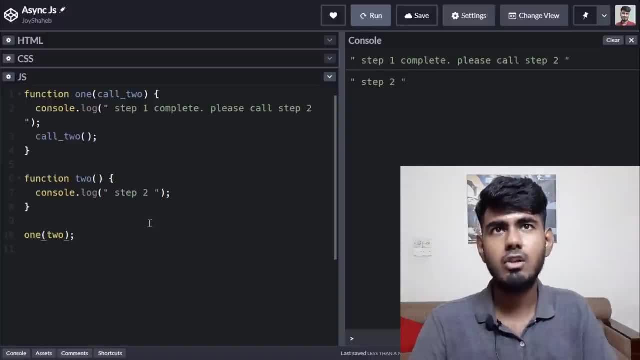 script runs from the top to the bottom right, so our consolelog is at the first, and then call two. but if you reverse the order, what will happen? let's see. control x- okay, call it over here. control v- control s- okay. and now clear the console, run it and let's see. 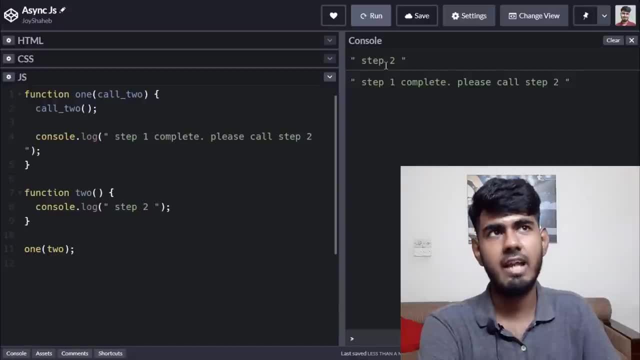 what happens now. you can see that step two is first and then step one complete. please call step two. don't worry about this. if you don't understand it, we're going to look at another example right now for that. we're gonna start our ice cream business right now for. 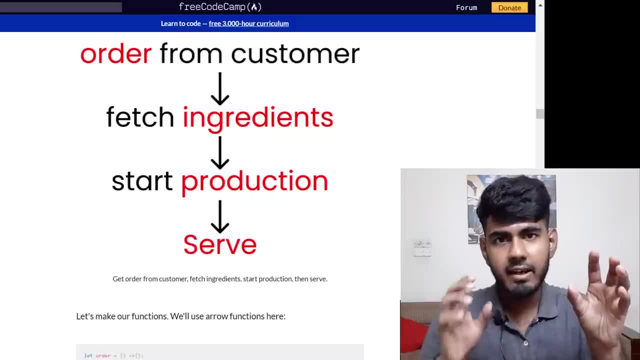 that we need to know the relationship between our customers and us. you can see that this is the flow. okay, first we get the order from the customers, then we're gonna fetch the ingredients, then we're gonna start the production and then we're gonna serve ice cream. okay, so we're. 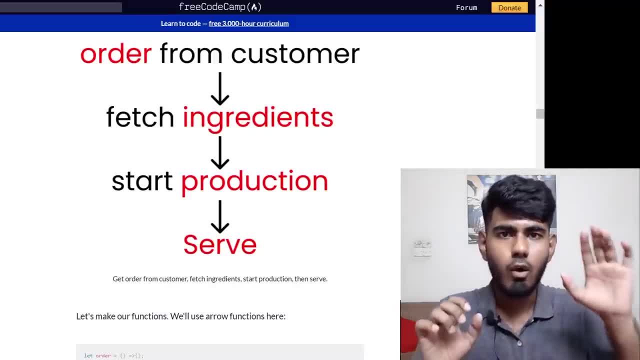 gonna create two functions. how many functions? two functions: order function, production function. okay, if we don't get the order, we cannot start the production. this is how we are forming a connection between these two functions. using what, tell me? using a callback. come on, let's go to code pen and see the example. come over to code pen over. 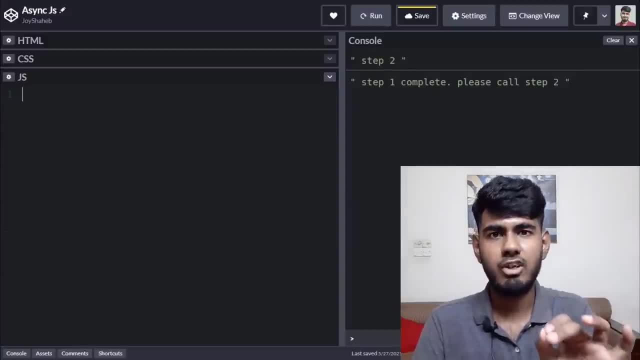 here you delete everything. okay, we're gonna use arrow function. what function arrow function? right, let first is order, because without the order the production doesn't start. okay, order equal to brackets, then arrow sign: curly braces like this. okay, now, right, the production function. but before that, clear this console. okay, let production reduction. here we're. 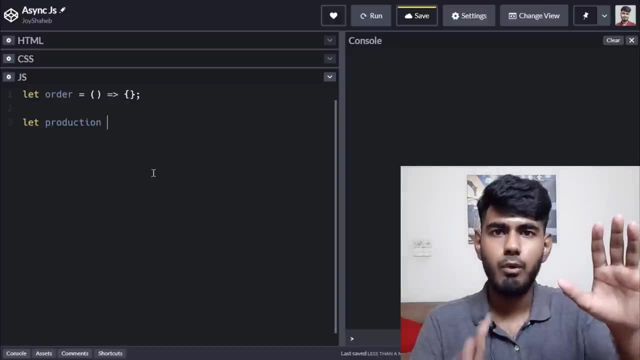 going to make the ice cream. okay, so once we get the order, we're going to start the production of our ice cream. okay, production equal to brackets- error sign: curly braces like this. okay, now, in order to form that connection that every time we get the order the production will start, we do it. 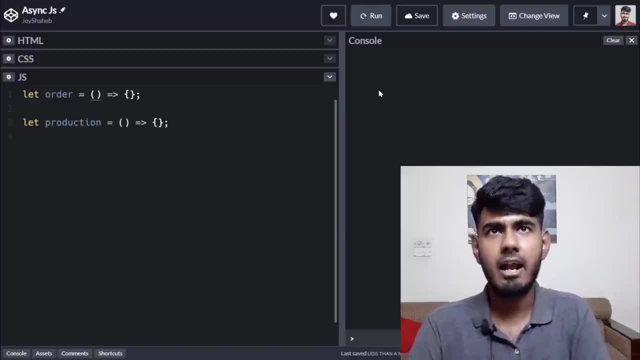 like this: okay, you come over here, okay, you pass an argument, we're gonna name it call production, okay. call underscore: pro duck shown- okay. and inside this curly braces, we're gonna write the same thing. okay, the exact same name. control c, control v over here and then brackets: okay. 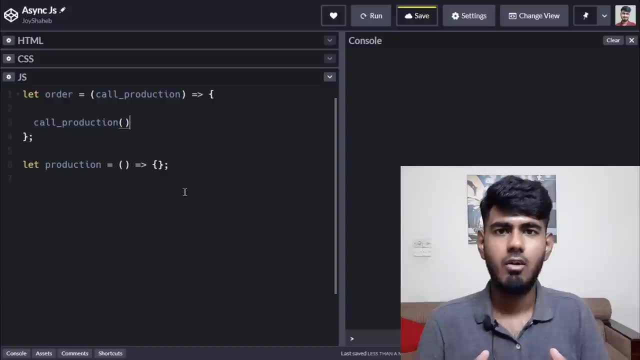 brackets like this and look at there, we have formed a relationship between these two functions using. what a callback. now let's test it. now we're gonna write consolelog: consolelog: okay, order placed. please call production like this: okay, and inside over here, we're gonna write consolelog: consolelog. 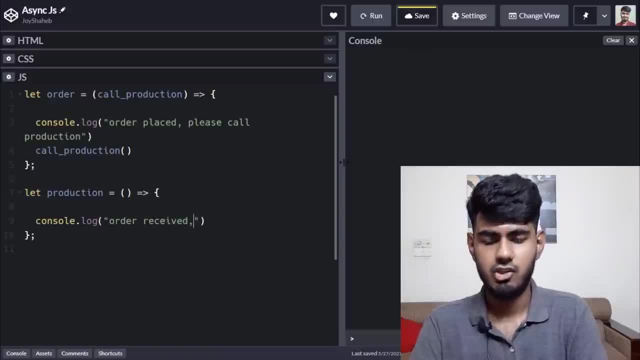 order received, starting production. like this: okay, now, in order to run our function, what we will do is we're gonna write order over here or there and inside that order we're gonna write the production. we're gonna pass this function over here, inside here. okay, pro duction. like this: okay, so control s clear. 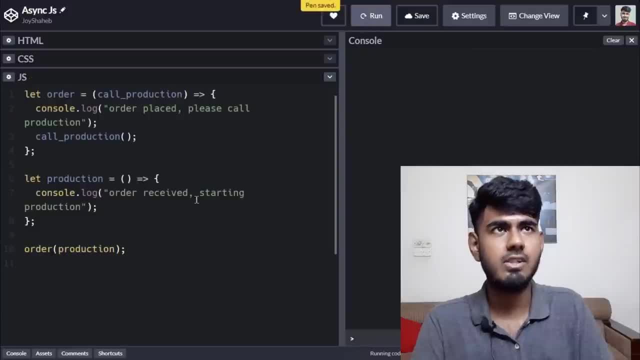 the console, save it, run it. let's see what happens. now you can see that we have order placed, please call production. and then we got order received, start production. i hope you understand how the system works of forming relationship between functions using a callback. now let's understand. 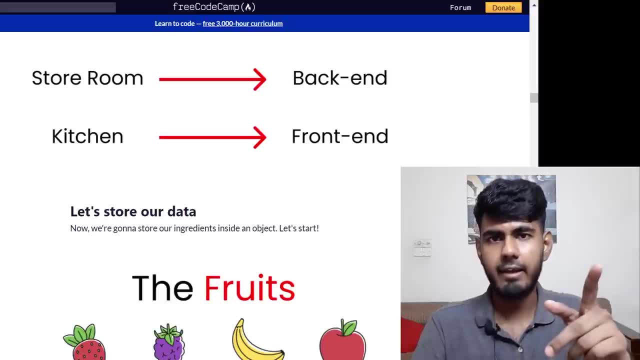 one more thing: the relationship between the front end and the back end. the front end is our kitchen, where we will make the ice cream, and the backend is where we will store ingredients like fruits, liquid stuffs, machineries, raw materials, chocolate, etc. you know what raw materials means? right, the stocks, our stocks. 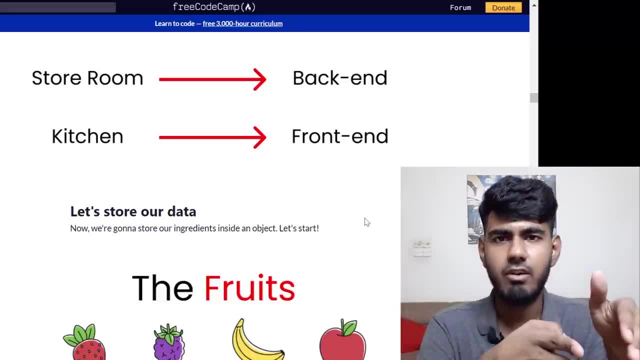 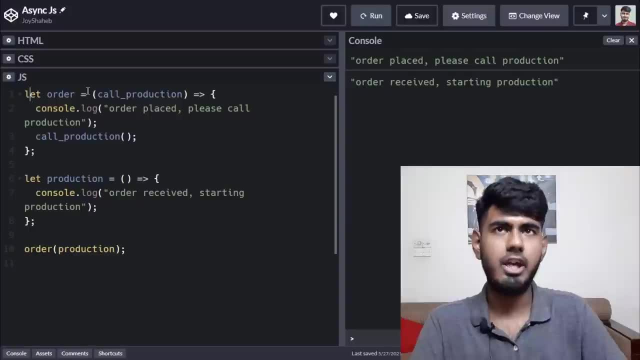 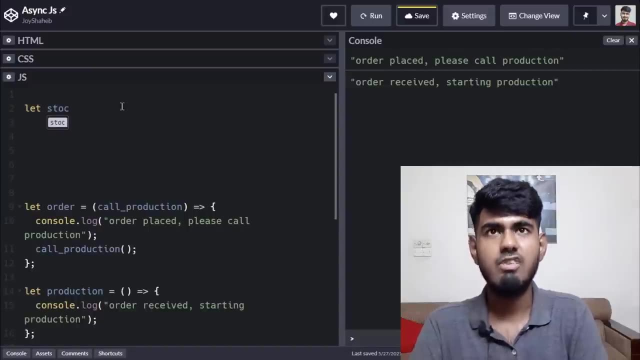 so the stocks is the back end, kitchen is the front end. okay, so we're gonna store our stocks inside a variable. okay, so come over to coat pan over here at the very top. okay, you keep some space over here and we're gonna write let, okay, let, stocks. so this variable will hold all of our 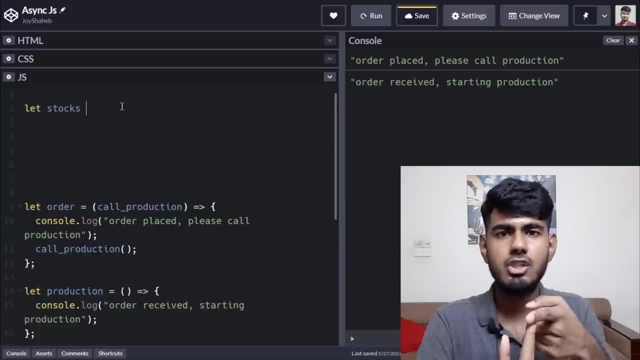 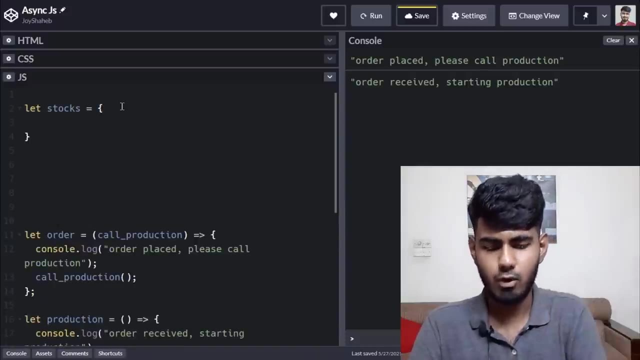 stocks like fruits, liquids, holders, toppings like chocolate, peanuts, etc. okay, and that equal to. we're gonna create a object over here like this object. okay, and inside that object we're gonna write arrays like this: look f r u i t s. okay, then colon. over here, we're gonna store all our fruits inside. 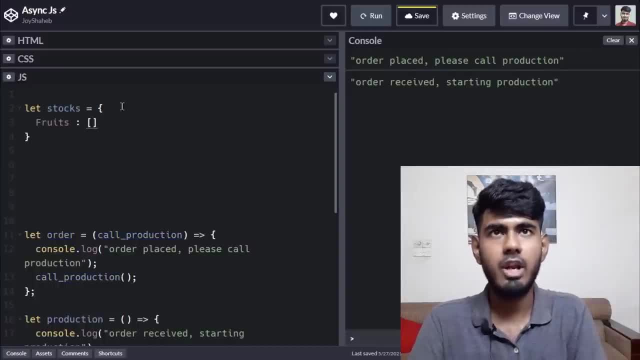 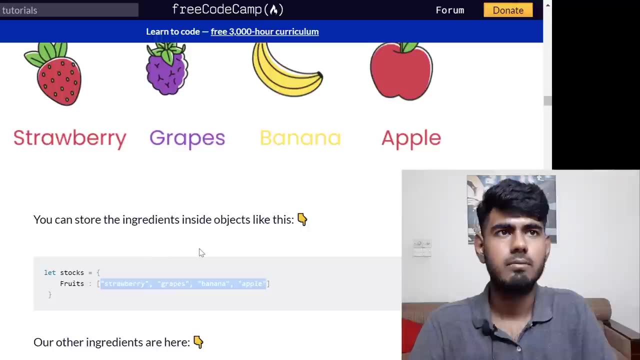 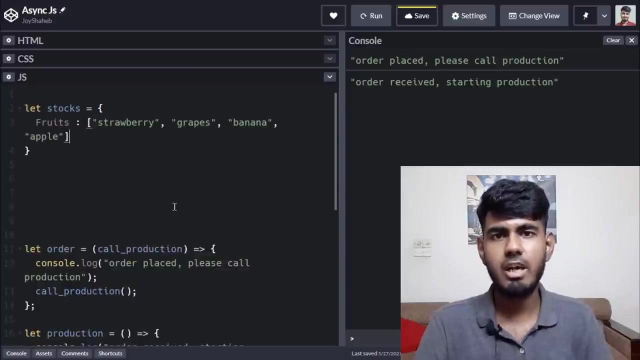 what and array: okay, like this: then we're gonna write the name of our fruits as i have defined them over here. i'm gonna copy it over here. okay, control c and then control v over here. now pause the video. take a moment to write these foods, okay. 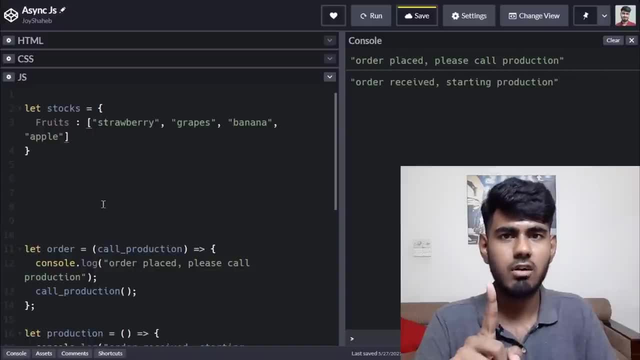 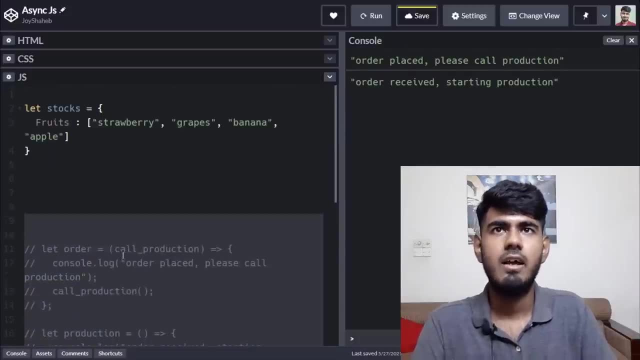 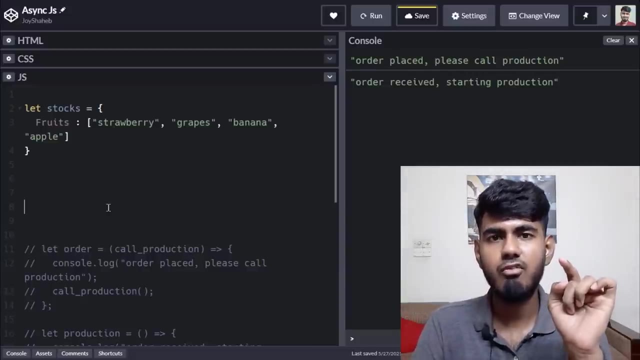 now, how do we access a single stock from this variable? okay, we comment everything from here, from the top to bottom, like this. comment this like this, and in order to select one stock, we'll do it like this: first of all, we write the name of the variable. what is the name of the variable stocks? okay, s t o c k? s. then dot y dot, because it is an. 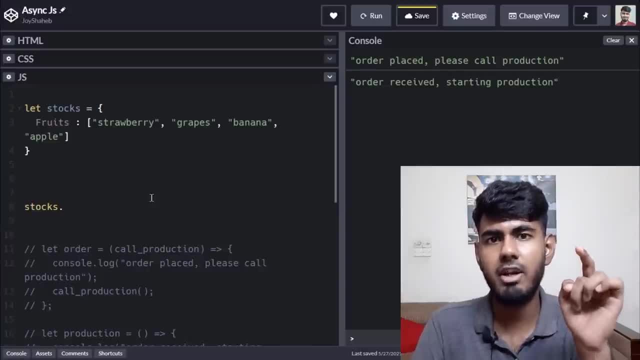 object. in order to access the object, we need to form a dot, and then the name of the object, which is fruits. okay, capital letter, f r, u, i, t, s. and then what is this? this is an array. so how does the array works? is it is arranged in the order of zero, one, two and three? okay, so in order to access that you? 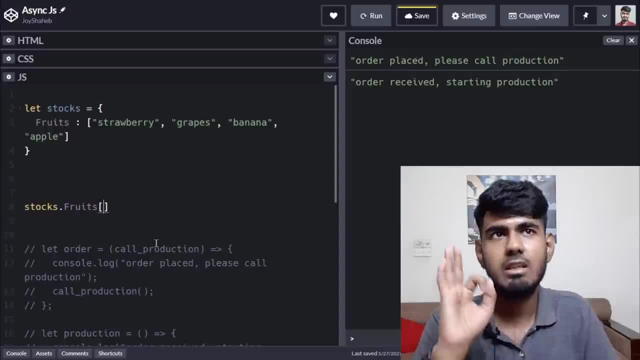 write square bracket, okay. and then, if you want to access the banana, let's look at the order zero, one, two. we write two over here, okay, and now let's print it on the console. in order to do that, we write console dot log, then brackets at the end bracket close it control s, clear it and then run. 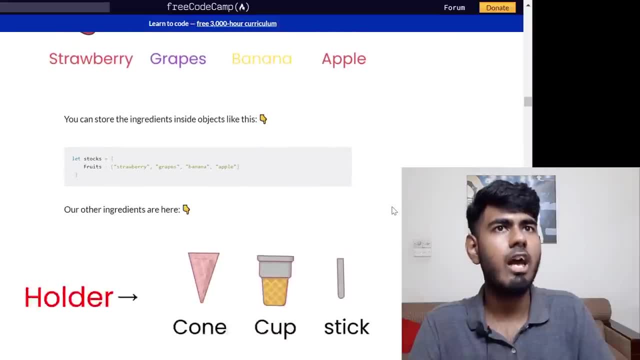 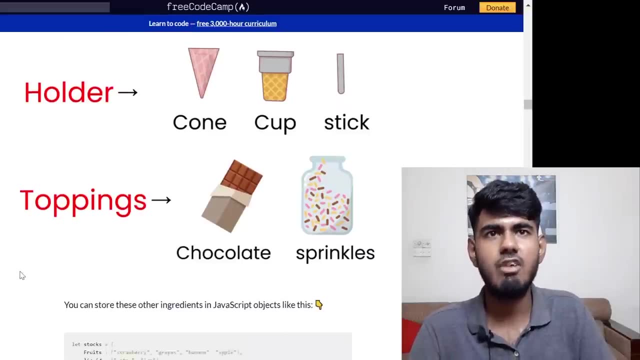 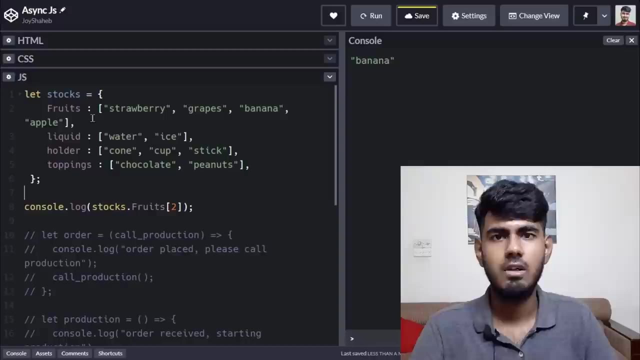 it. look, we got the banana in the same way. we have more stocks. we have the holders, the cups, cones and the toppings as chocolate sprinkles. so this is the variable that i have created. okay, i'm gonna copy it from here- ctrl c, and then over here i'm gonna paste it: ctrl v. now pause the video. take. 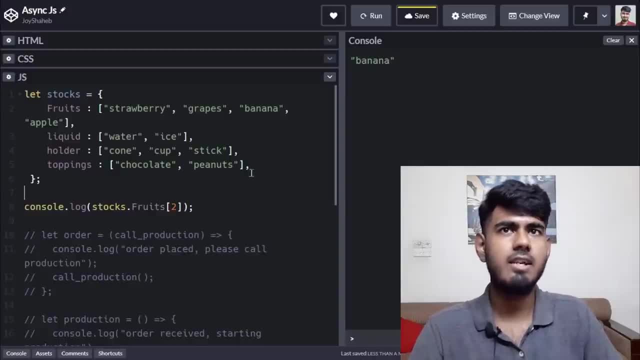 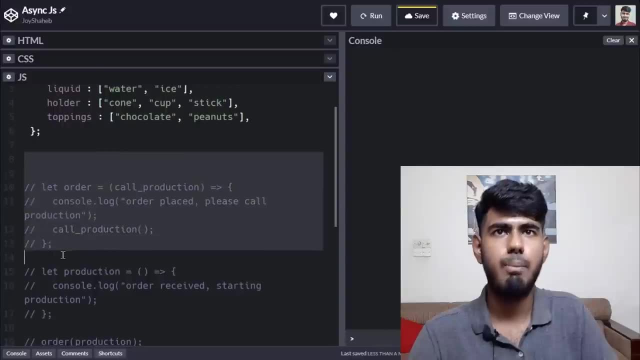 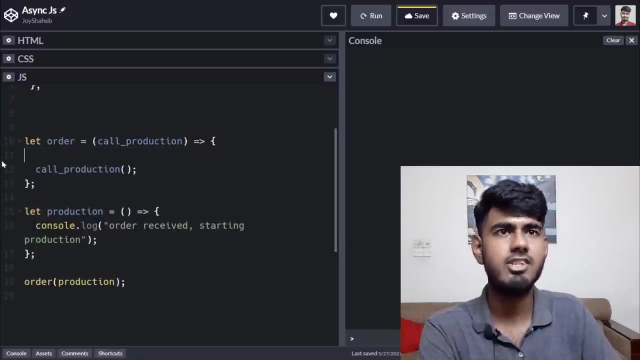 a moment and write these stocks on your code editor. so once that's done, you clear this from here. okay, clear the console and you bring all of this back. okay, like this: there we go. okay, now we're gonna clean our console from here, remove this and we're gonna remove. 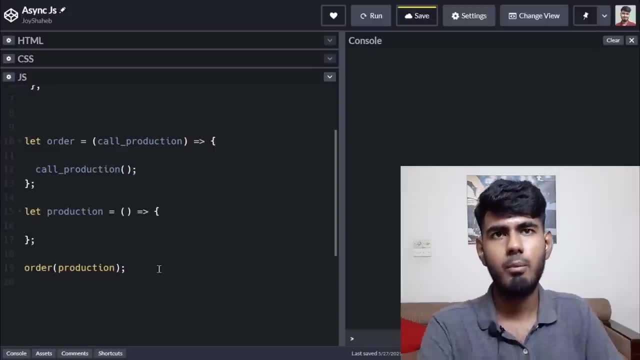 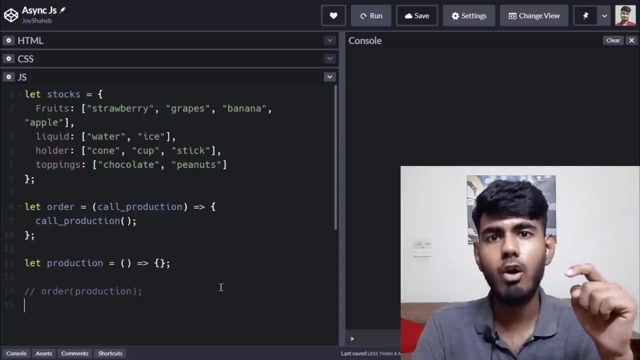 this, okay, and keep everything else, and then you comment this from here. okay, now the now. the first thing is the order. right, customer places the order. the order is changeable, which means: how many options do we have? look at our menu: we have the strawberry, grapes, banana and apple, which means 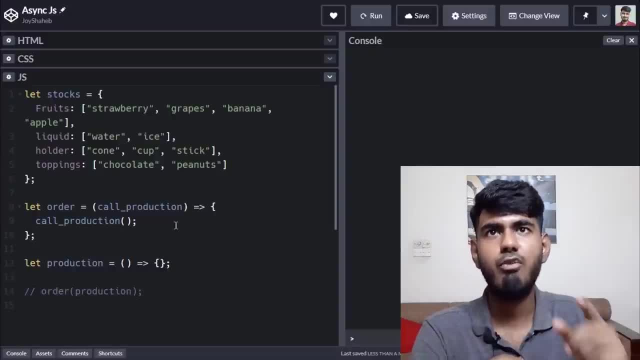 that the customer can pick anything he wishes, which means that for this we need a variable. so over here we're gonna write fruit name f-r-u-i-t. okay, underscore a-m-e like this, then place comma over here. so we have two arguments: the fruit name and the call. 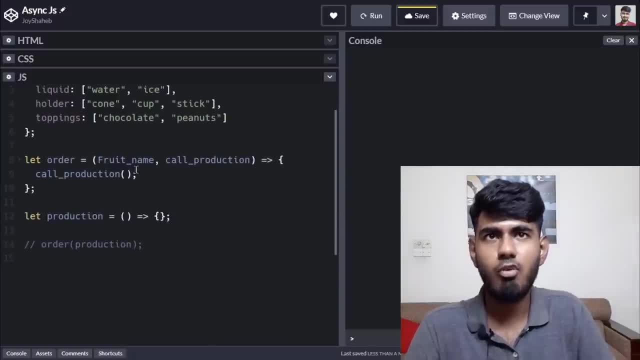 production. the customer picks the fruit, it gets over here and then we get to know that what the customer picked and then we're gonna start the production. this is how we are forming a relationship between our functions. okay, and over here you uncomment this and we need to keep it. 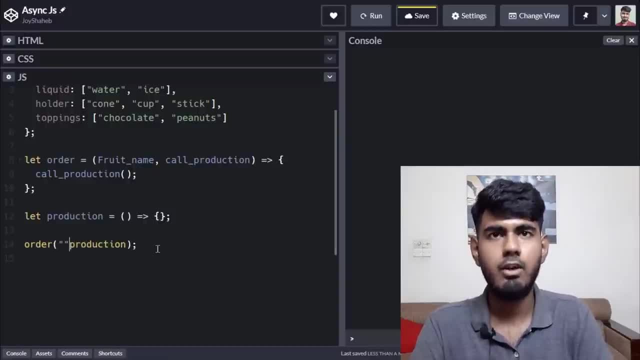 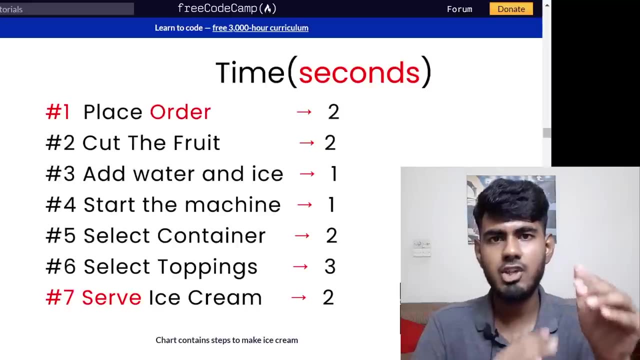 blank for now. okay, you give double quotes over here, then comma. okay, you control s. if you remember, this is our steps, along with the time. so, in order to ensure the time function, we're going to use set timeout and we're going to print the steps on our console. 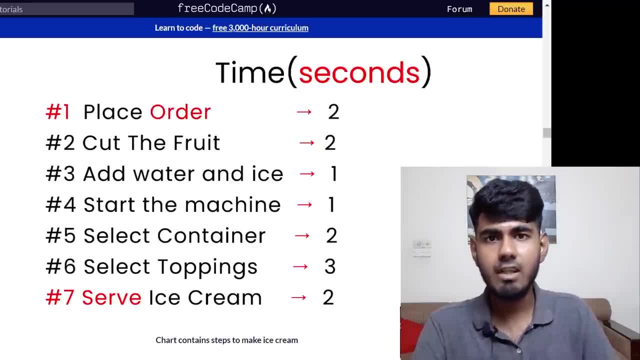 okay, so follow along with me. first of all, we're going to place the order by picking a fruit name. okay, come back to vs code over here. and and in order to select the fruit and place the order, it takes two seconds. how many seconds? two seconds. so come back to vs code over here. 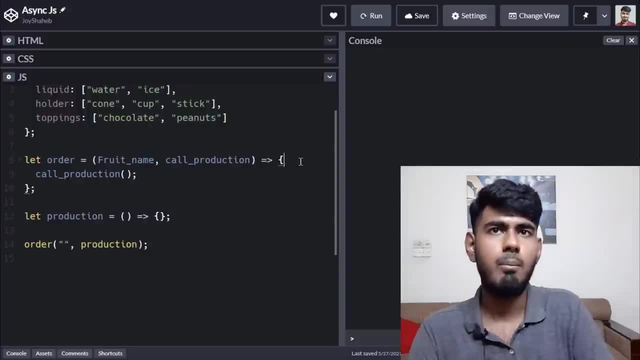 inside this order function. okay, come here and write console. or before writing consolelog, you have to use a set timeout function because it takes how many seconds? two seconds set timeout like this, and inside over here we're gonna use an arrow function. you can also use an anonymous. 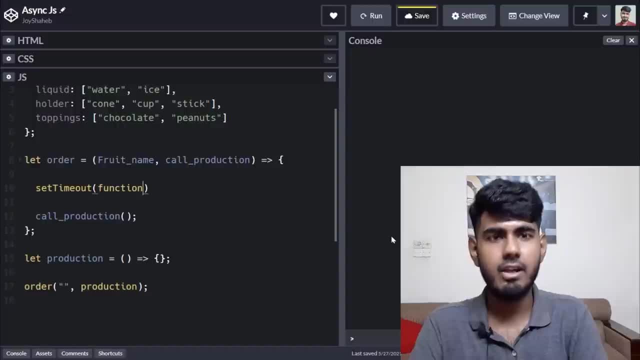 function like this: look: function: bracket, curly braces like this. but we're gonna keep it simple. we remove this, this function from here and you're gonna give that arrow sign like this: okay, and at the end we're gonna place the time function. okay, how many seconds? two seconds. so we're gonna write. 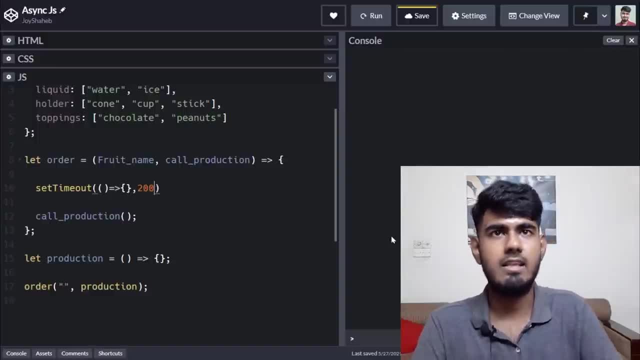 two thousand milliseconds, okay, two, one, two, three like this, and inside over here we're gonna write consolelog, because we're gonna, because we're gonna print the result on our console, okay, and use a back tick. we are not gonna use double quote. no, no, we're not using double quotes, we're. 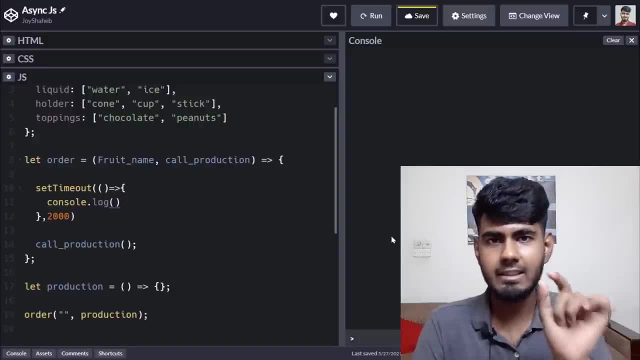 going to use a back tick. we're not going to use double quotes. we're going to use a back tick. we're going to use a back tick. we're going to use double quote. no, we're not using double quote. no, we're not back tick. what back tick? if you want to access the back tick, look at my keyboard over here. 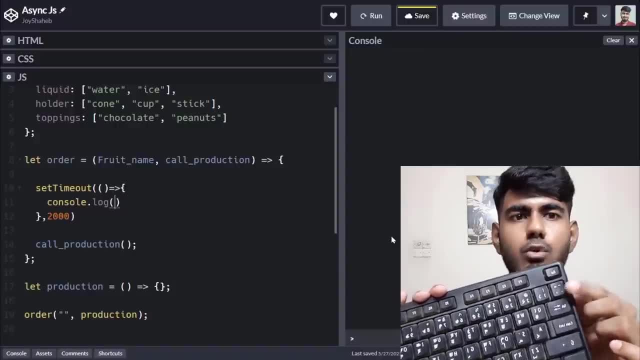 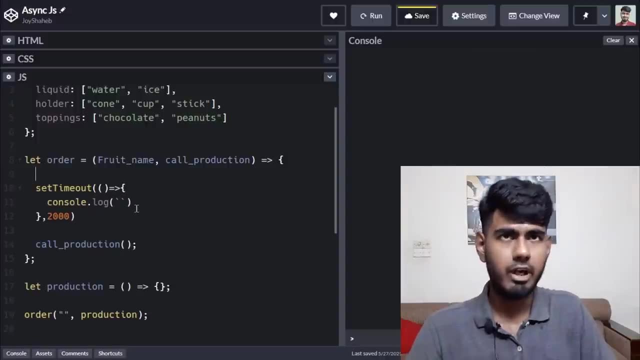 this is the exit key and this is the key to write back ticks. okay, so you click this just once and it is gonna print us two back ticks like this. now we're gonna pass this foot name inside this consolelog. so how do we do this? first of all, we're gonna write a dollar sign. okay, what a dollar sign. 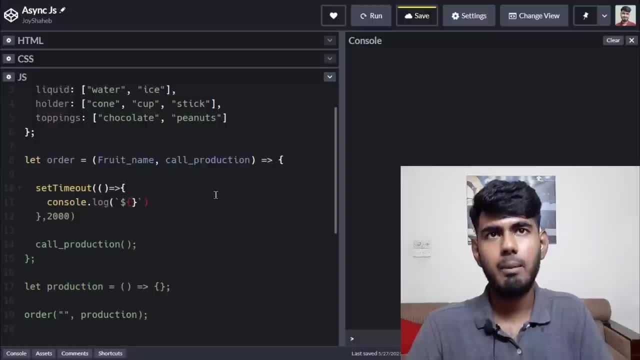 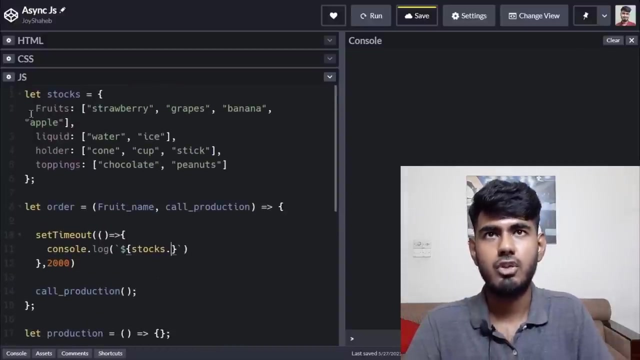 dollar sign and then curly braces like this, and then we're gonna place this inside here. but the before that we need to write something, we need to write the stocks. okay, that's because we are picking it from our stocks, right, so stocks, then the name of our um fruits. okay, so dot f r u i t s. 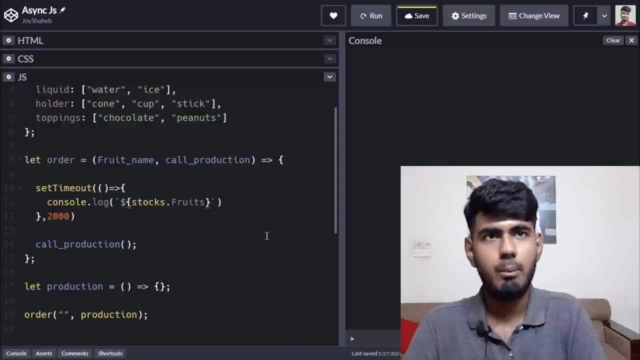 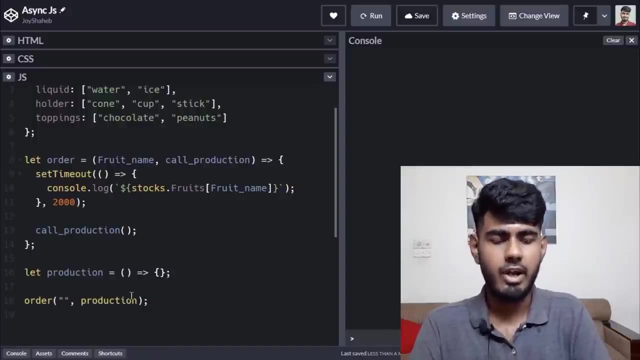 and then what square brackets, right square brackets over here, and then we're gonna pass this inside there. okay, ctrl c, ctrl c, and then right ctrl v over here. okay, now we're gonna save it. let me show you how the system works. okay, so over here, um, we're gonna write zero control s clear. 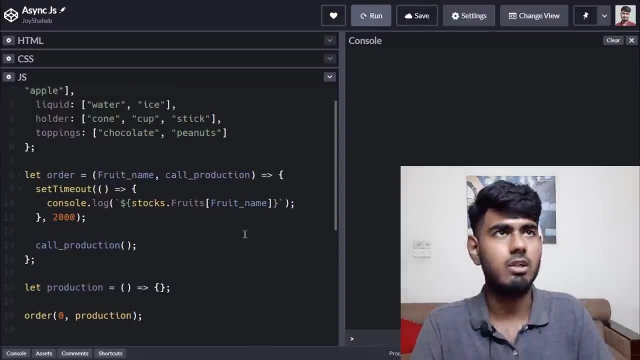 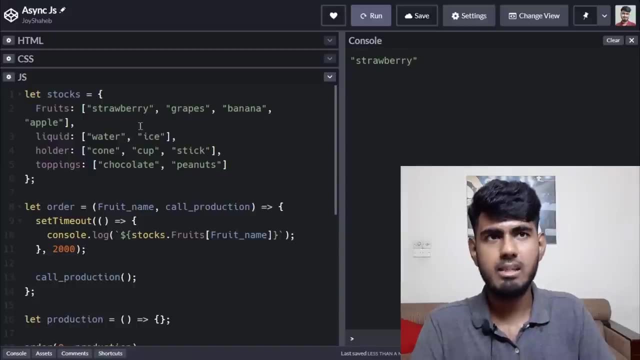 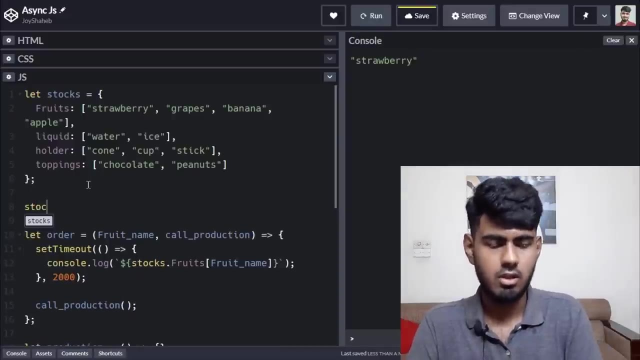 the console, run it, let's see what do we get on the result? we got strawberry. you can see that the first fruit on our stocks is the strawberry, right? i explained this to you, right? if you can recall how to access the stocks, we do it like this: stocks, dot, f r u i t s, then square brackets and then the. 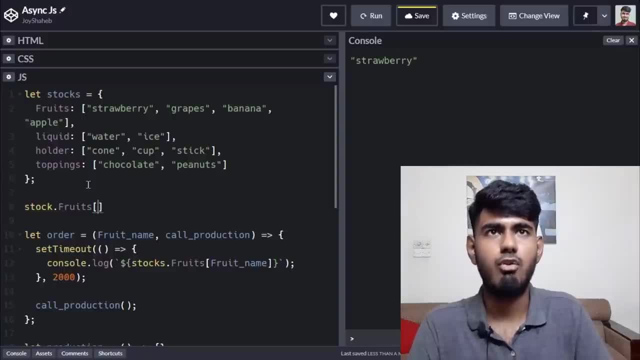 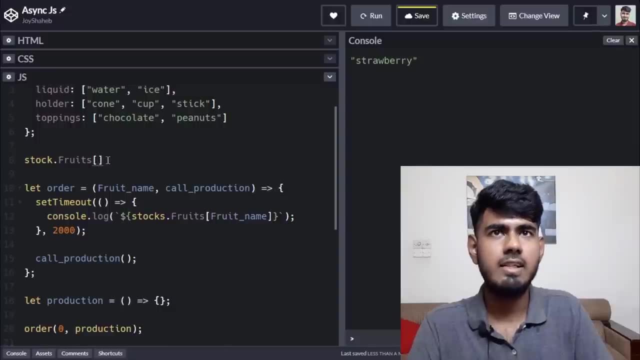 i mean the order of, i mean the order of the fruit: zero, one, two, three, right. so i have placed this inside, over here, and then inside the array i have placed this and over here i have placed zero, which means that this zero is coming over here, which eventually means that we're gonna get the strawberry. 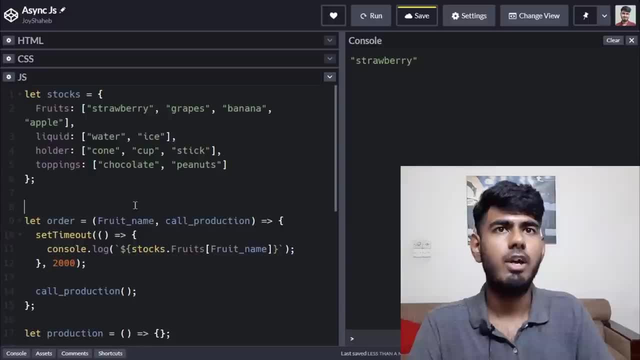 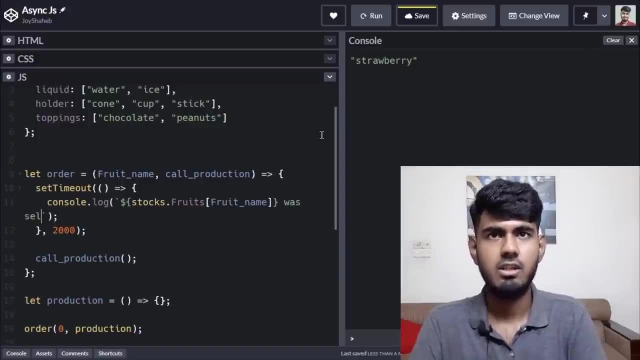 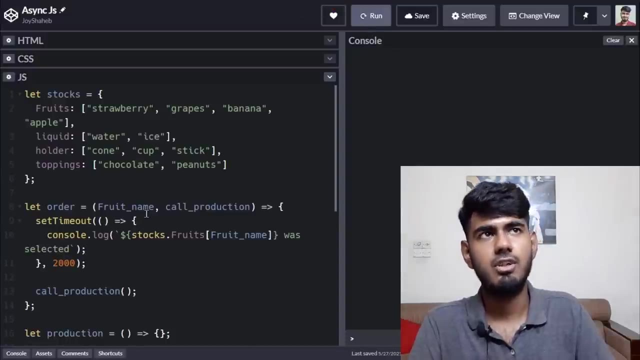 i hope you understood this. nothing complicated, okay. stocks dot fruits. then this, and over here you write: was selected like this. then ctrl s clear the console, run it and let's see what we get. strawberry was selected. you can see that. you can notice that we got the result after two seconds. 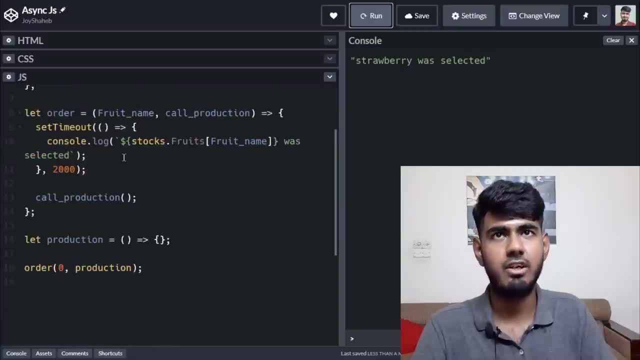 why is that? that is because we are using a set timeout function over here which takes two seconds. i mean it. i mean it prints our result after two seconds. okay, let's start writing inside our production function. okay, so come over here. we're gonna use another set timeout function which runs. 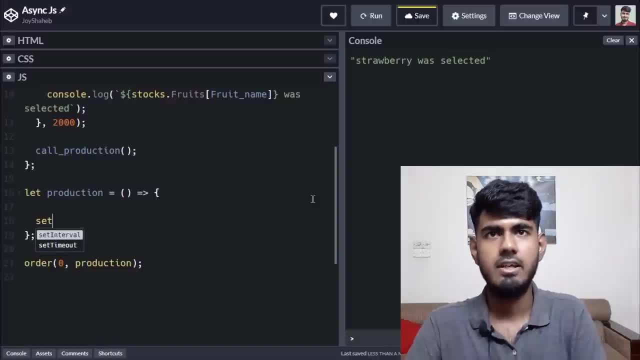 zero seconds. how do we do it? we do it like this: right, set timeout brackets and pass a function over here like this: arrow function: okay, and then it's gonna run in zero seconds. how many seconds? zero seconds. so right, zero, zero, zero, zero. inside over here, we're gonna write consolelog. 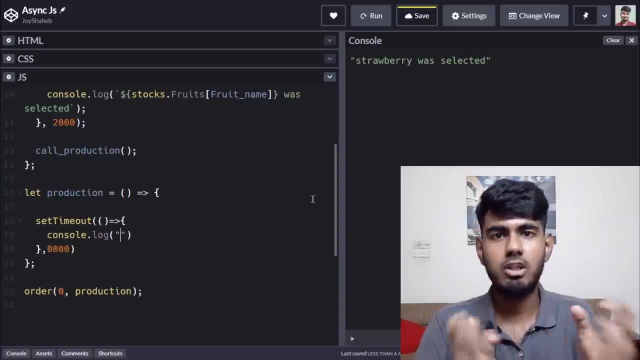 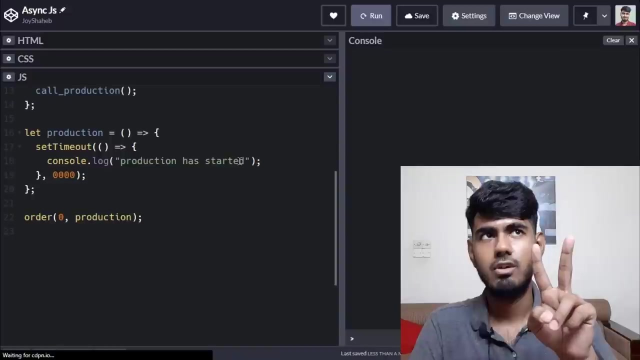 and write production has started. and that is because we got the order right. production has started. ctrl s clear the console. let's run it, so we're gonna get the result after two seconds. one, two, there we go we have the production has started. and then strawberry was selected. 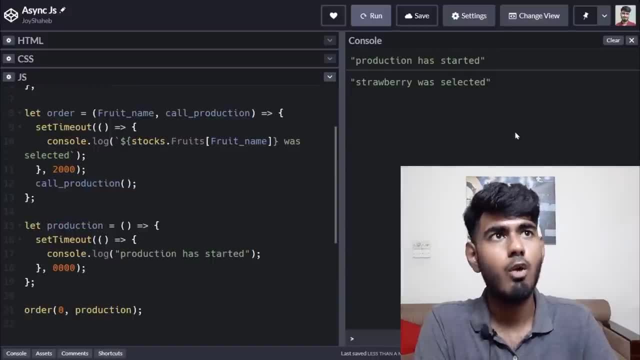 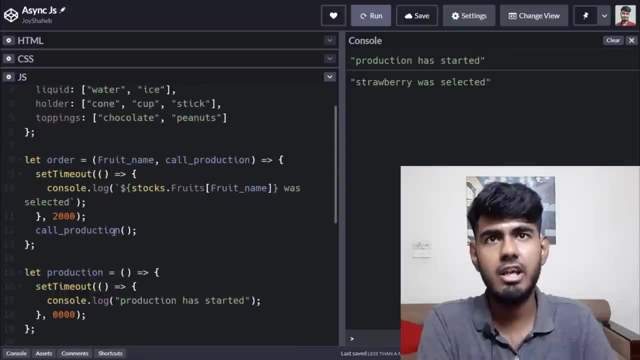 now we are seeing a odd behavior over here. why is that? we were supposed to get this one first and the production has started at the last. that's because if you focus over here, you can see that. look at the order. okay, javascript runs from the top to the bottom. 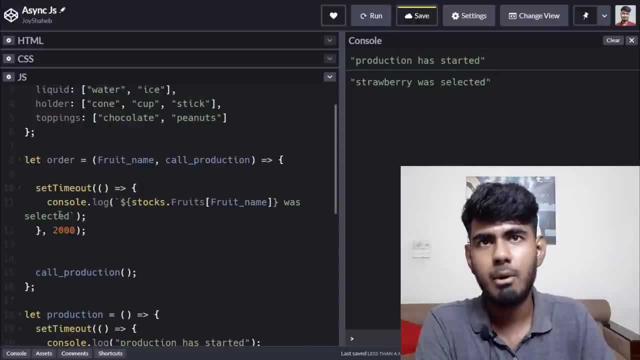 okay, so javascript runs from the top to the bottom. okay, so javascript runs from the top to the bottom. so it is saying that this is a set timeout function, which means that it's gonna take two seconds, and this one. this is gonna take how many seconds? zero seconds, okay, so this one will. 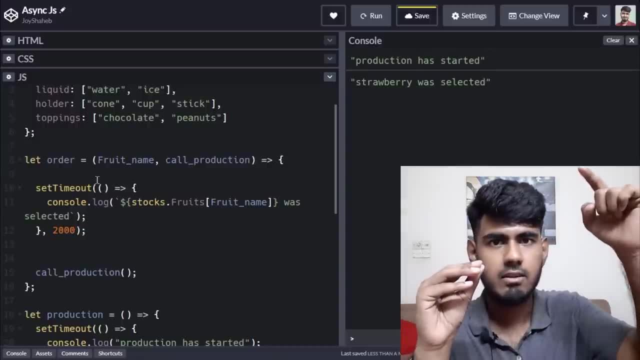 be stopped. this is over here and thus call production will start immediately. so this is the call production, which is: production has started over here and strawberry was selected. this is over here. that's why we're getting this order, but if you want to fix that, what you have to do is 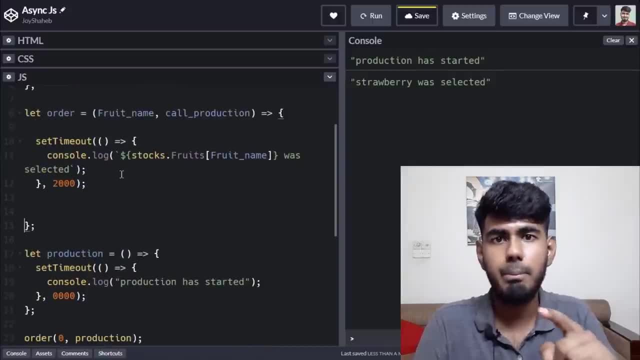 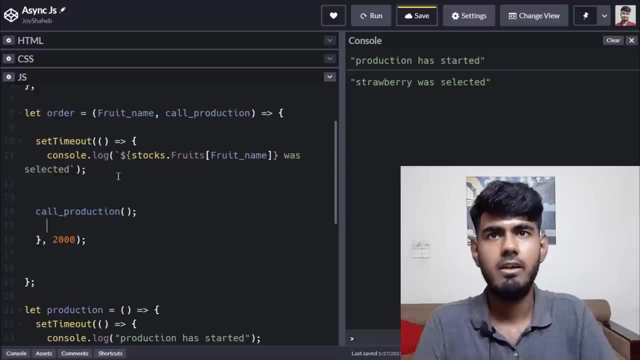 you're gonna cut it from here- ctrl x- and you're gonna place it where inside. that set them out. function. okay, like this. look, control v over here. okay, now what will happen is it's not gonna start the production unless the foot was selected. now let's save it, clear the console and run it, and 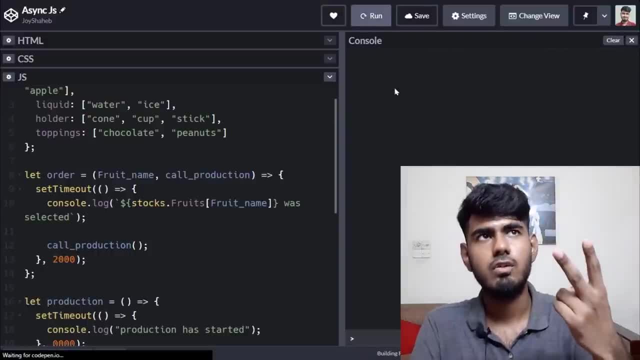 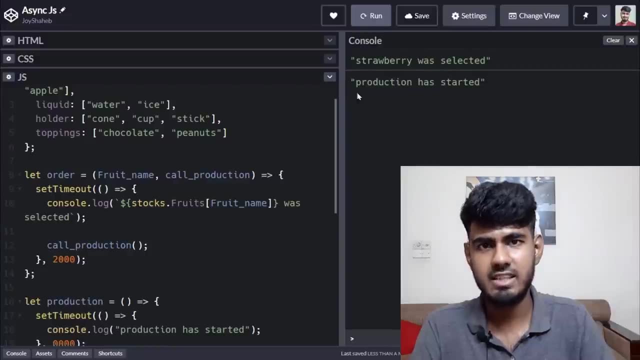 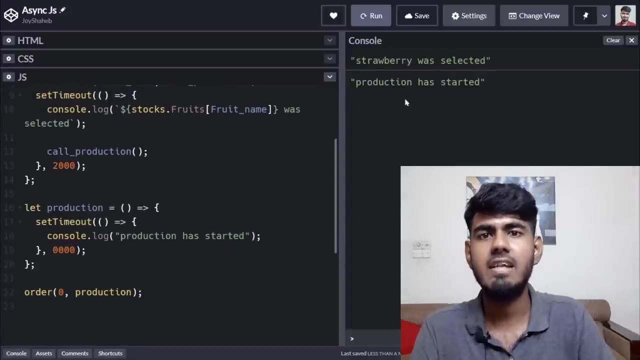 let's see what happens. one, two. so you can see that after two seconds strawberry was selected and immediately we got the result: production has started. that's because we have set two seconds for which one strawberry was selected and zero seconds for which one. production has started, like 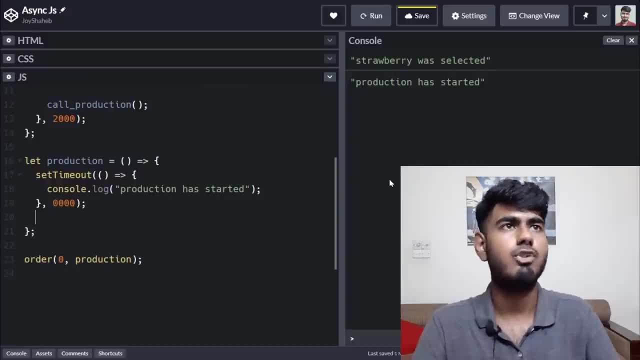 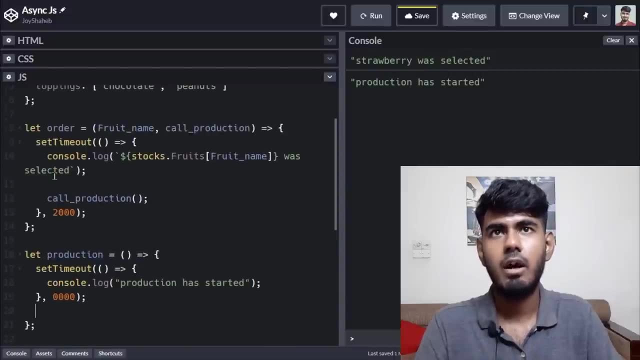 this. i hope you understood so far. now let's look at our second step, which is um. we're gonna cut the fruit and it will take two seconds, so come inside the production function. we are done with our um order function. okay, you can minimize it like this. we don't need it anymore. 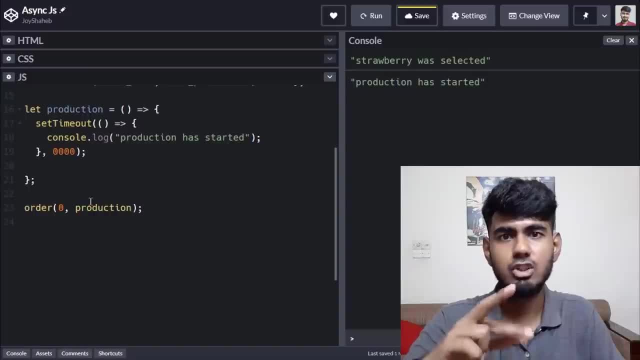 and don't make that mistake again, otherwise you're gonna get the reverse order which we watched previously, which is we got the production first and the strawberry at the last. don't write it outside, okay. don't write it over here. you're gonna write it inside this set timeout. 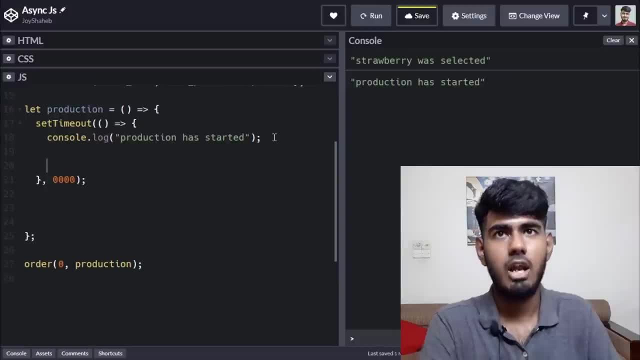 function okay. so you come over here and you're gonna write another set timeout: okay, it's gonna be two seconds. how many two seconds set timeout, okay, brackets, and then pass a arrow. function like this: okay. arrow sign: curly braces and then the time function. okay, how many seconds? 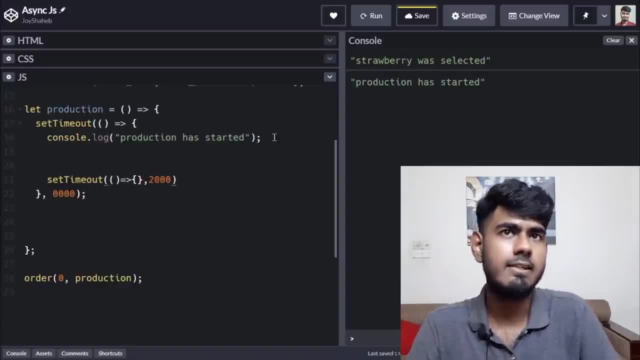 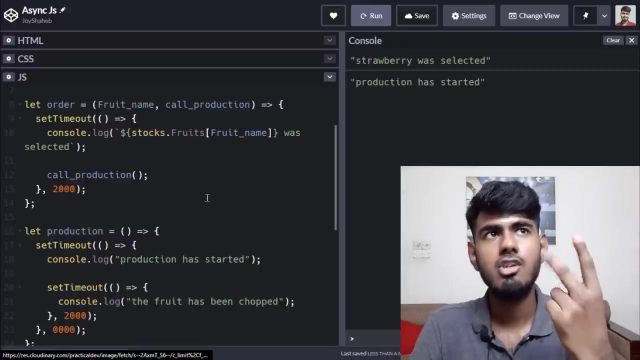 two seconds. two, one, two, three, like this, and inside over here we're gonna write: the fruit has been chopped. console the log. the fruit has been chopped, control s. let's clear the console, save it. let's run it and see what happens. one, two, again one, two. so we're getting the strawberry after two seconds. 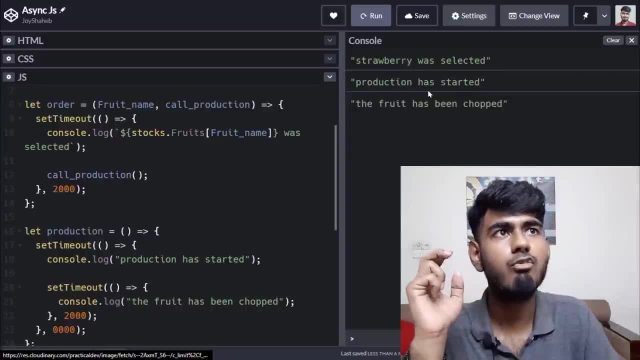 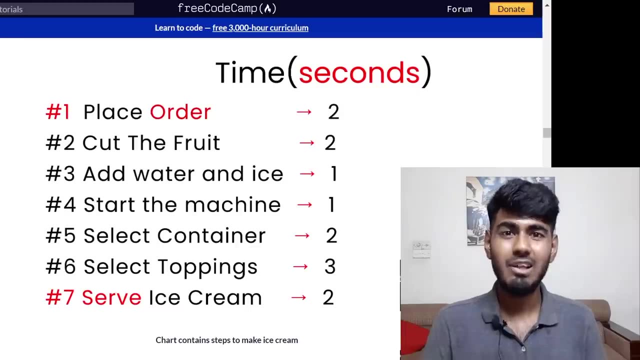 we have got the production immediately, and then we have got the fruit has been chopped after another additional two seconds. now our system is running perfectly fine. now let's follow the steps and complete our ice cream production so that we can buy ourselves a lambo. because why not? now the third? 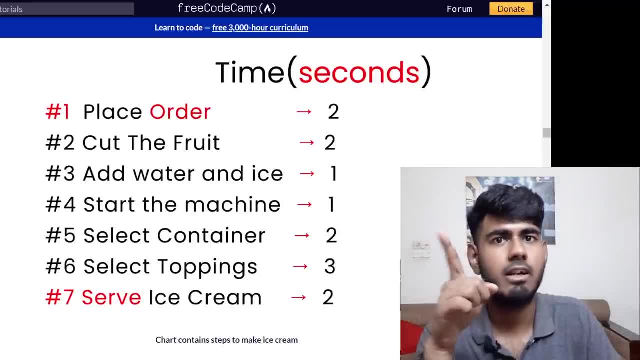 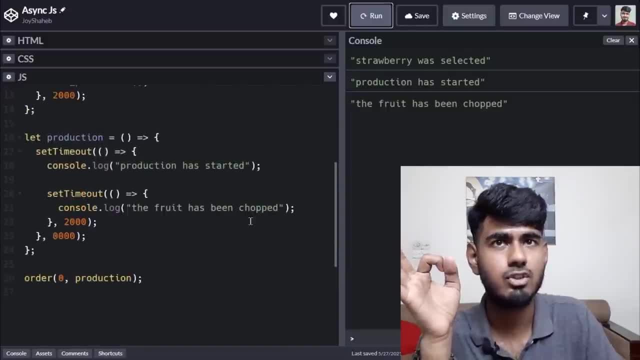 step is to add water and ice, and it takes one second. how many one seconds? so inside the production function. where will we write? we're gonna write it inside this set timeout function. so this is the. it will be the grandchildren. okay, so the fruit has been chopped over here. 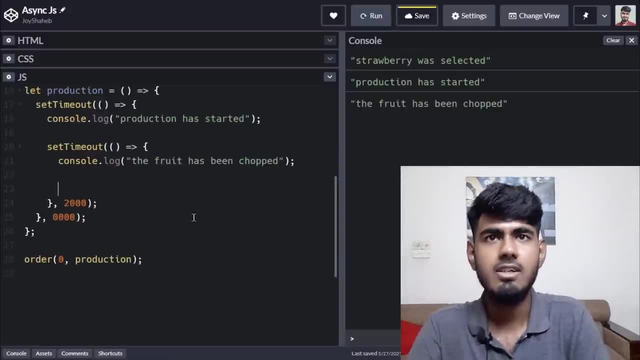 enter to give some spacings and you're gonna write set timeout like this: okay, brackets. then pass the arrow function like this: equal to okay, curly braces. don't worry, i know where we're going. we are going to a callback hell. this is called a callback hell and i'm coming to the point, don't. 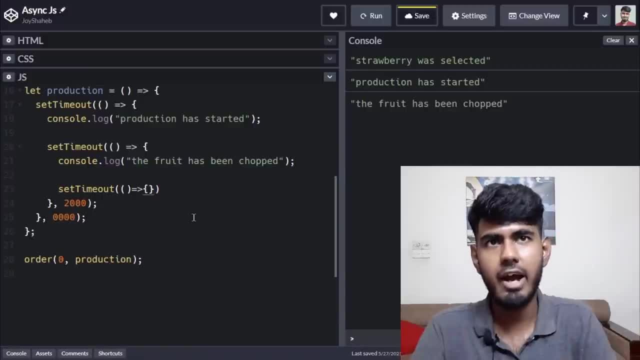 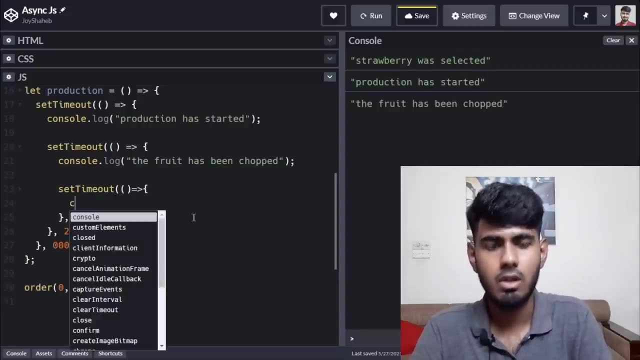 worry, don't, don't panic. okay, and over here you write the time function, okay, one thousand seconds, like this: okay. and inside over here, console dot log, like this: okay. inside over here, we are not gonna write double quotes, we're gonna write batics. that's because we have to add water. 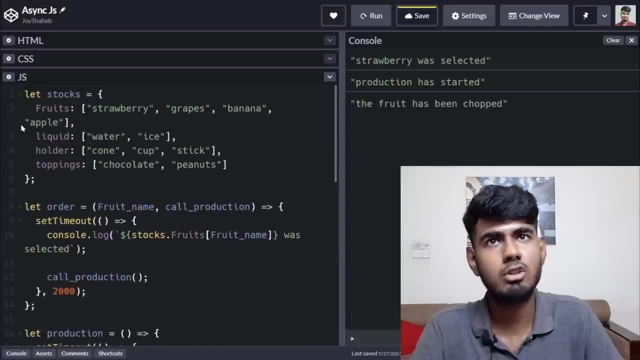 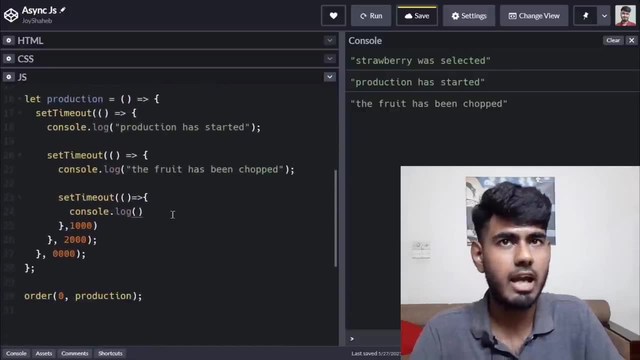 and ice and the water and ice is inside our stocks over here, which is the liquid, and then water. eyes zero and one in order to pick them. pay close attention to what i write over here. okay, don't focus on anything else. one, two, three. this is the next big chapter of the. we are going to write double quotes over here. okay, touler lower that we. how much that le studio number eachר. 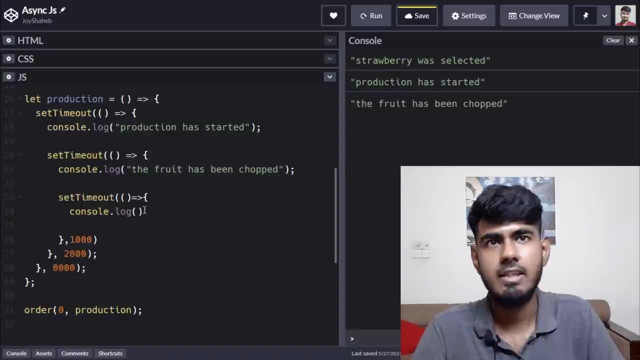 one, two, three. this is the third step. okay, inside over here, back ticks, what back ticks, like this dollar sign. and then curly braces, okay, curly braces like this, and you write end over here, okay, and then curly braces again, like this, along with the dollar sign. okay, you're gonna, you're. 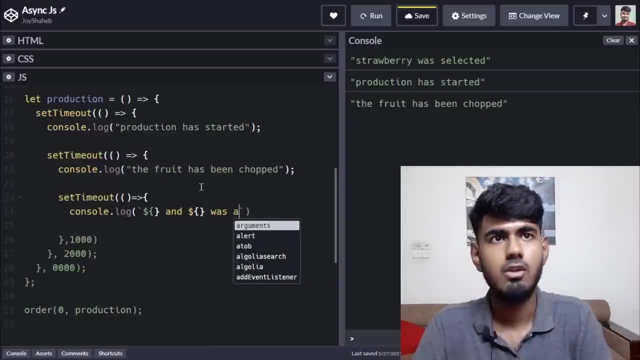 gonna write was added. so if you translate, it sounds like this dash and dash was added. so we're gonna write, so we're gonna pick the water and ice. so first of all, we're gonna write stocks- okay. stocks dot liquid. okay, as because it is the name of that object, liquid and then square. 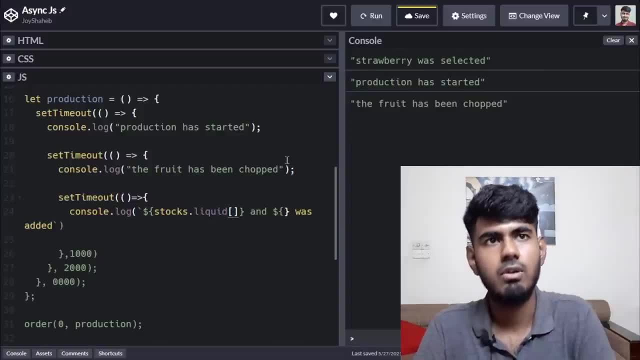 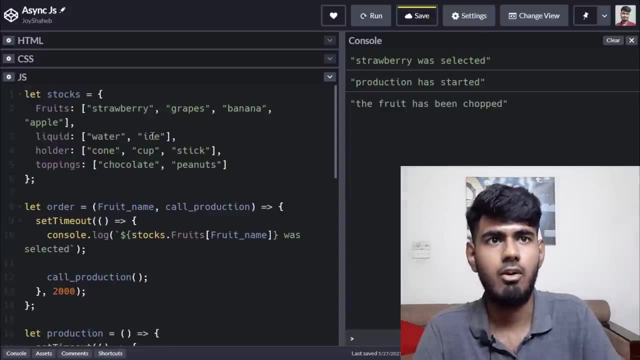 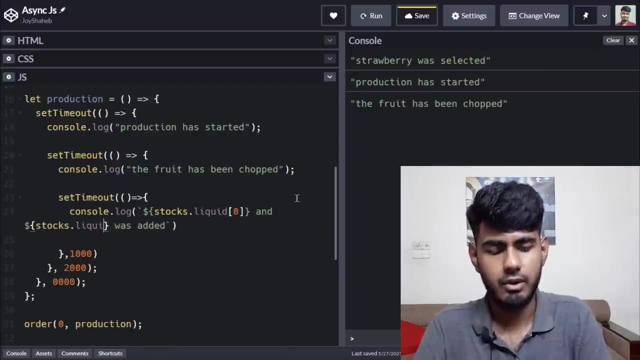 brackets like this: over here, you're gonna write zero. okay, that's because it will select the water. the first thing is the water, and then we have the ice. in order to pick that ice, over here, okay, we're gonna write stocks dot liquid. okay, then square brackets, we're gonna write one. 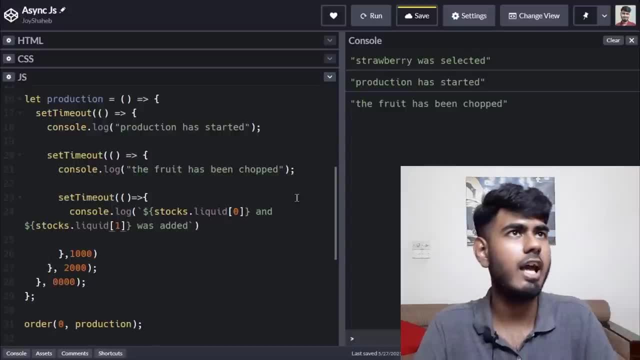 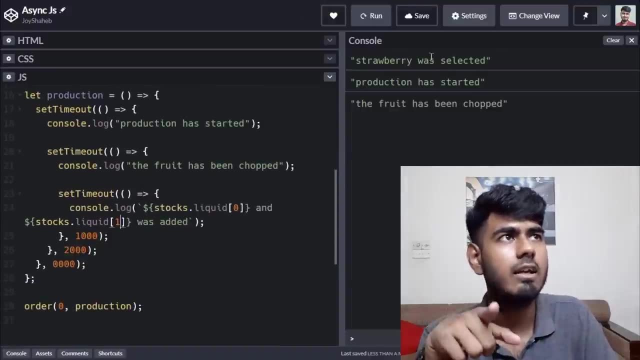 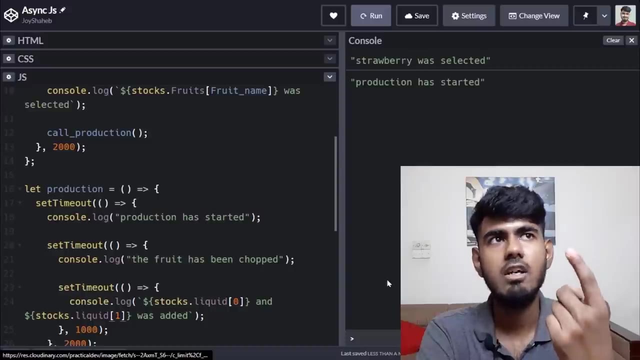 and it will pick the ice like this: okay, control s and then um, we have also set it to one second. okay, so we're gonna get it after one second. clear the console, save it right. let's count one two again. one two one. now you can see that we got this after two seconds. we got this immediately. 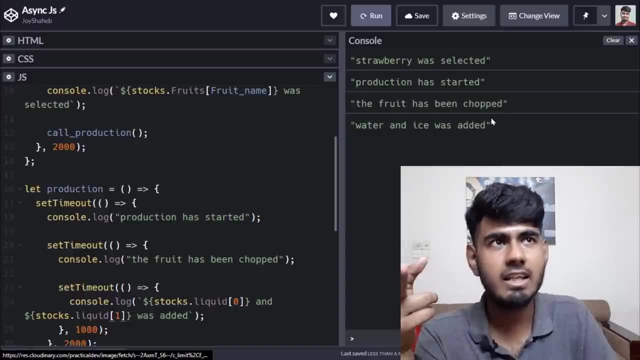 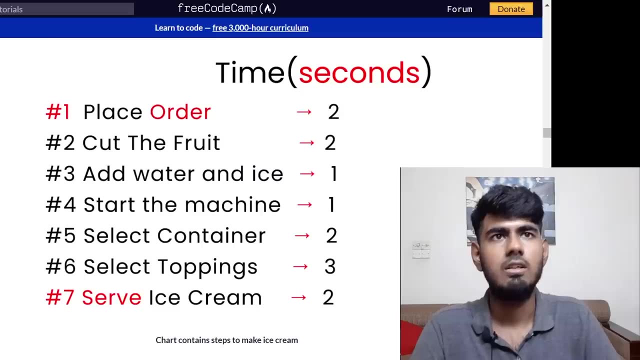 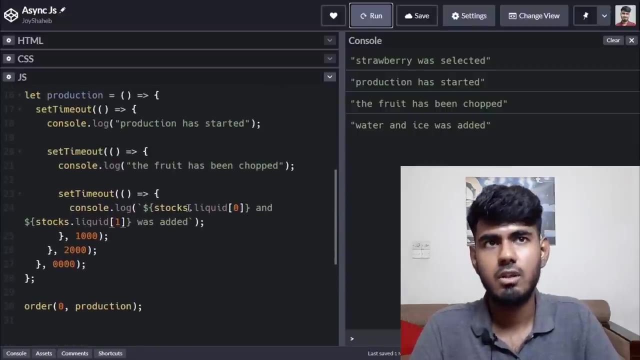 we got it after two seconds and an additional one second later we got water and ice was added, which means that our function is running properly. now we're gonna start the machine. it will take one second, okay, um, inside this, okay stocks dot liquid. i mean where we have selected. 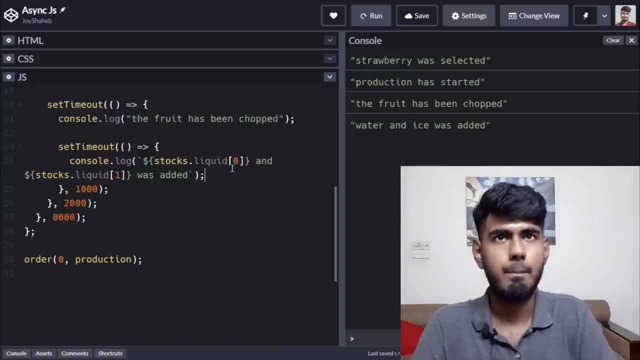 the water and ice. okay, so inside over here, um, we're gonna write set timeout. okay, then the arrow function over here, curly braces. and over here we're gonna write what the time function. okay, 1000 seconds, like this. and inside here we're gonna write console dot log and then we're gonna write. 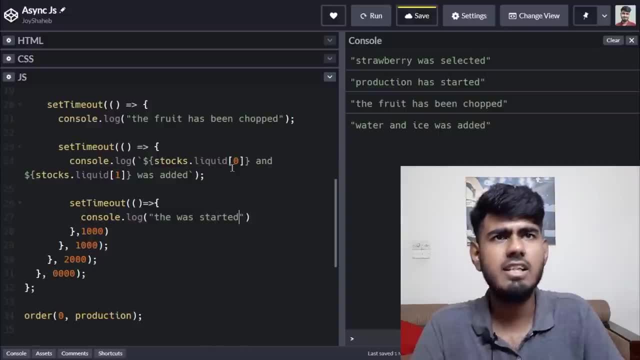 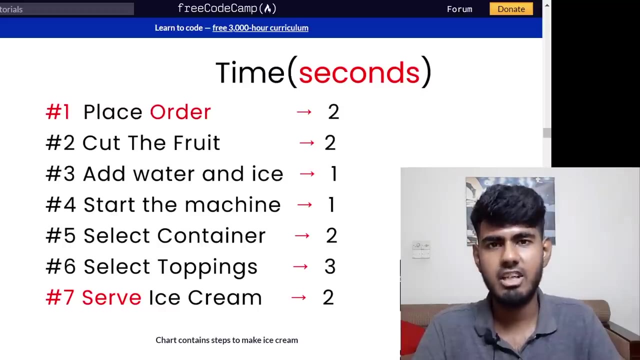 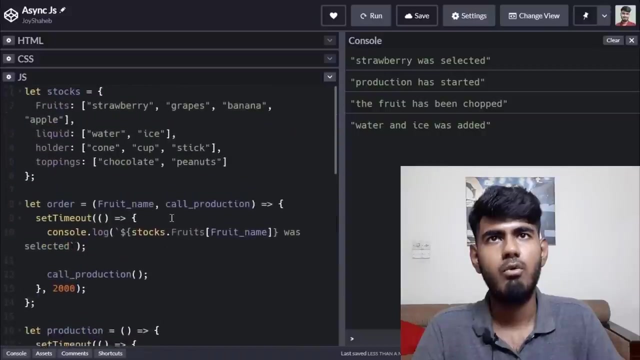 the machine was started. now let's write: the machine has been started. made. the machine has been. let's write: the machine was started. okay, control s. let's complete all of our steps and then run it together. okay, the next step is we need to select the container. okay, now, if you come over to the stocks, you can. 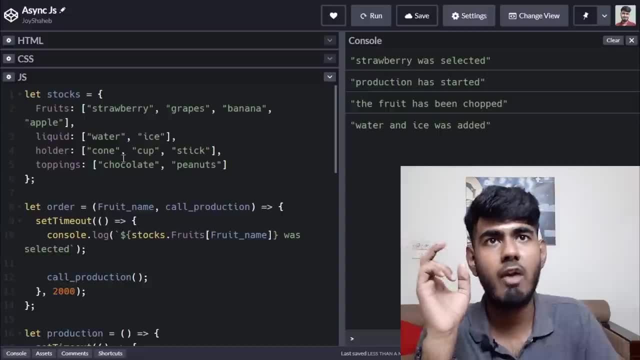 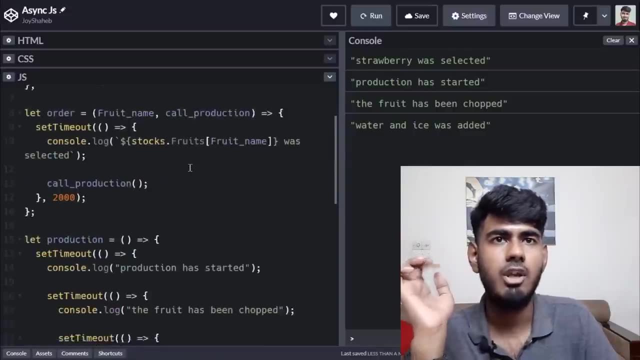 see that on the holder object we have a lot of options. we have the cone, the cup and the stick. let's pick the cup. no, i changed my mind. let's pick the cone. okay, in order to do that, you come over here. okay, where the machine was started. okay, and at the bottom, over here, we're gonna write the set. 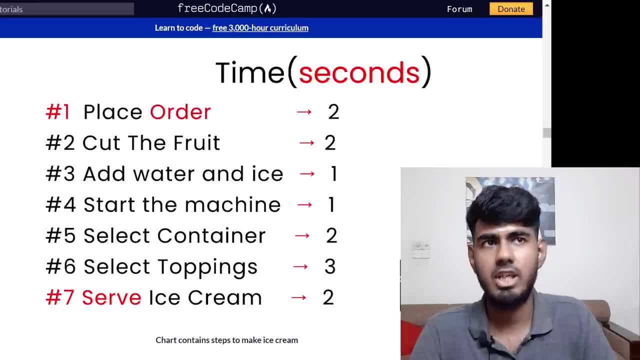 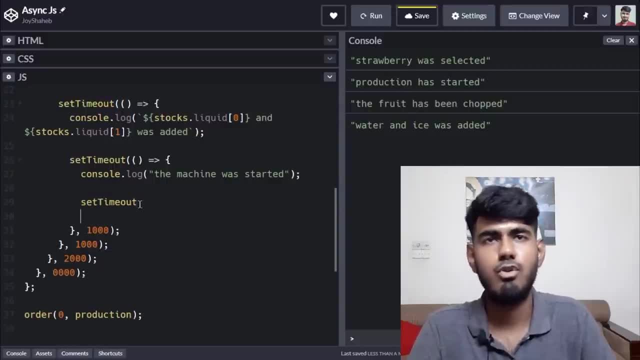 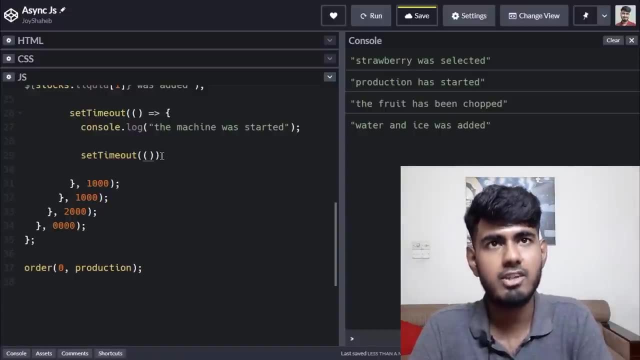 timeout, so the cup takes um two seconds. okay, so you're gonna write set timeout like this: okay, keep some space, otherwise you're gonna get confused by yourself. okay, set timeout and then brackets. then over here you're gonna give that arrow sign- i mean the arrow function- and then you're gonna set it. oh sorry, uh, the time over here. 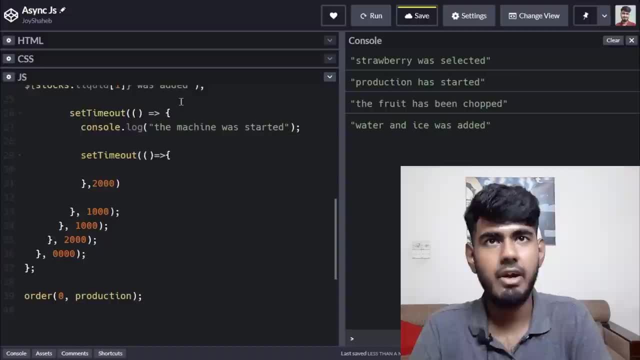 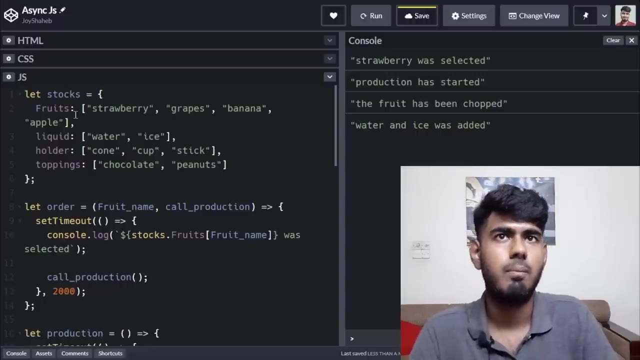 two seconds and then inside over here we're gonna write console dot log. we have picked which one, the cone, right, let's see that. where is the cone holder? okay, stocks dot holder, dot zero: okay, let's write it over here. okay, don't get confused, it is over here below the machine. 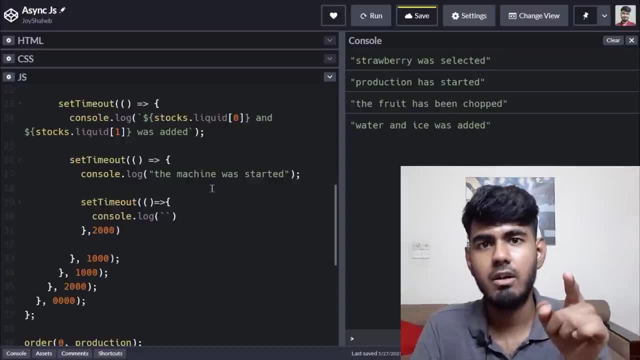 okay, we're gonna give what back ticks? that's because we are trying to get something out of the outside the function. okay, so dollar sign curly braces stocks s-t-o-c-k-s stocks dot. which one was that holder? h-o-l-d-e-r. that's because this is the holder over here. okay, stocks dot holder. and. 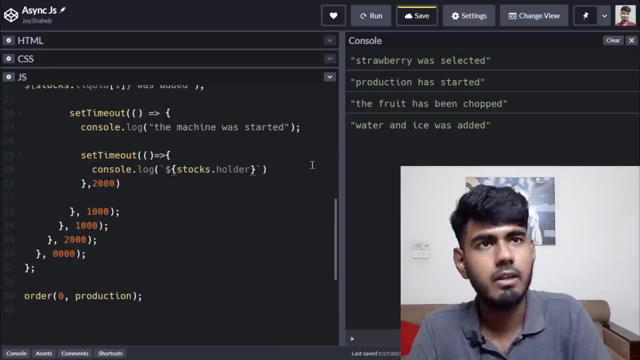 then zero. let's come back over here. then we're gonna give um square brackets like this, and then we're gonna write zero over here, and then we're done. what's the next step? the next step is: we're going to select the topping. ah, my god. what's the next step? we're going to select the topping. ah, my. 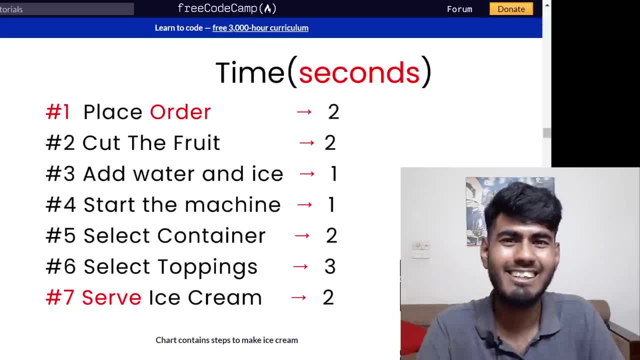 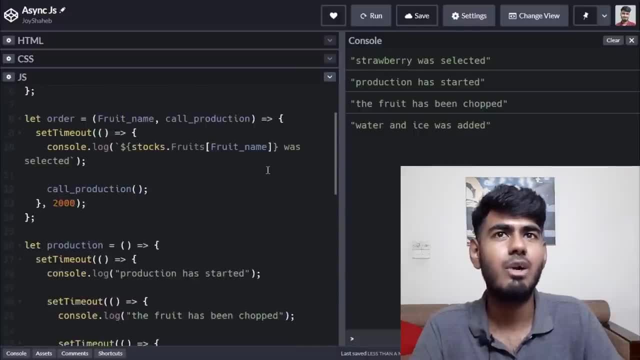 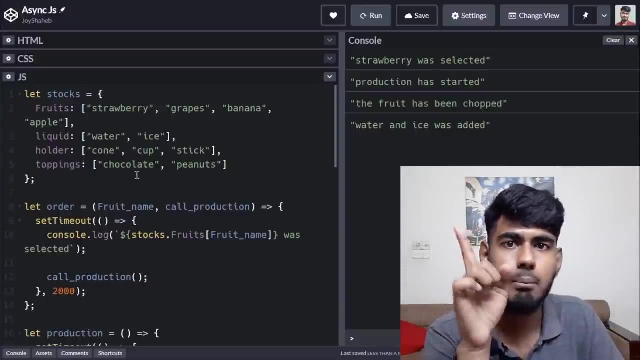 favorite: i love chocolates. what about you comment down below: do you like waffles, chocolates or peanuts? okay then, um, where was i? oh yes, we're gonna select what chocolates. okay, as the toppings look. stocks dot toppings. we have that s don't forget that. okay, and then we're gonna pick the zero you. 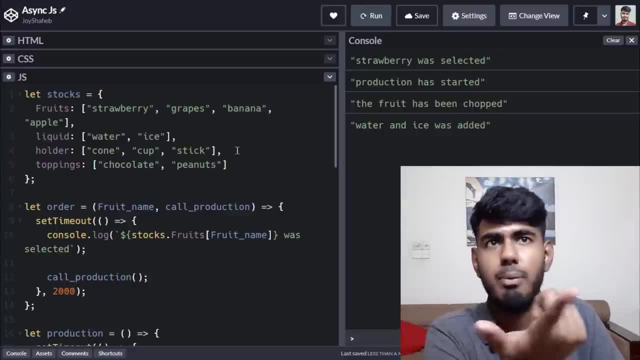 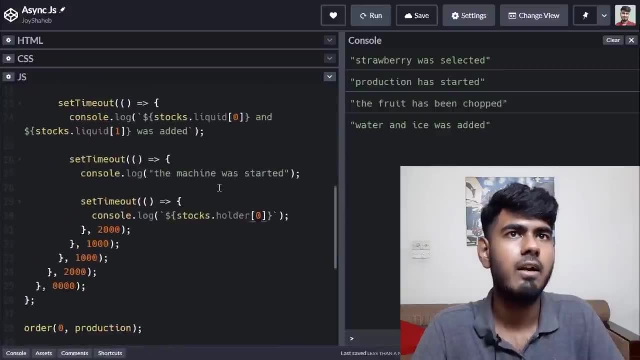 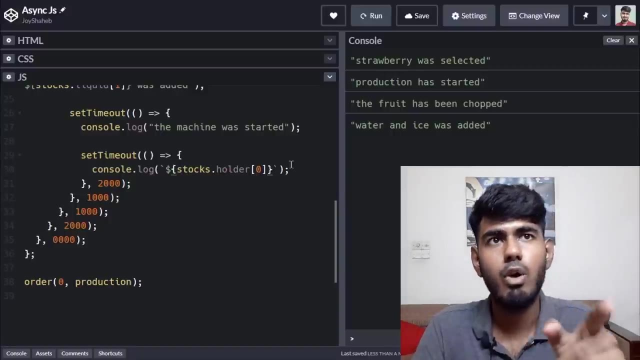 can also pick peanuts also as well. in order to pick that peanut, you're gonna write one: okay, stocks dot, toppings, dot one, okay, um, over here. okay, this is the holder. oh, i forgot to write okay, which means that the cup was. i mean the cone was selected, okay, selected. or you can also write: ice cream was placed on the cone. okay, come over here. 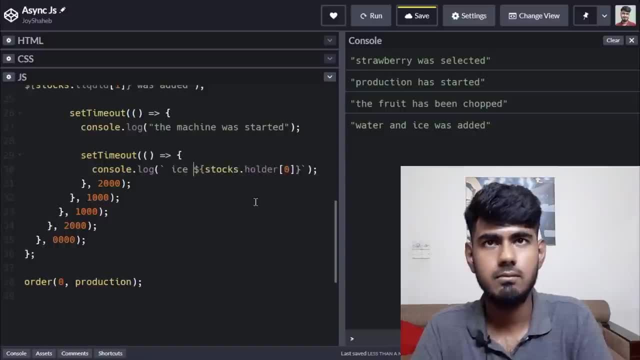 and write: ice cream was placed on what? the ice cream was placed on this one, which means on the ice cream was placed on the cone. ice cream was placed on the cone. ice cream was placed on cone. all right, so inside, over here, uh, give some spacings and we're gonna pick what the topping. 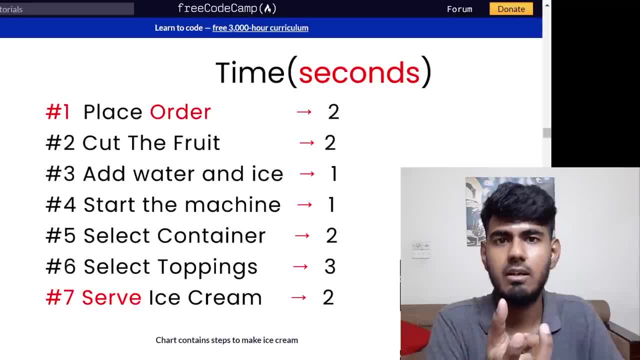 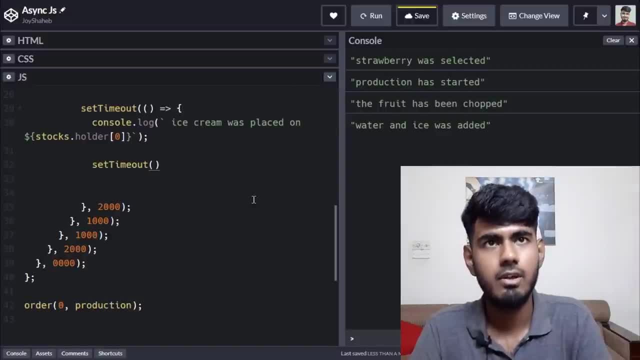 it takes three seconds because you need some time to melt the chocolate, right? so over here you write a sec timeout. okay, it's gonna take an arrow function like this and then it's gonna take three- oh sorry, three- seconds. okay, so what are we gonna do? we're gonna pick toppings, so console with log, like a. 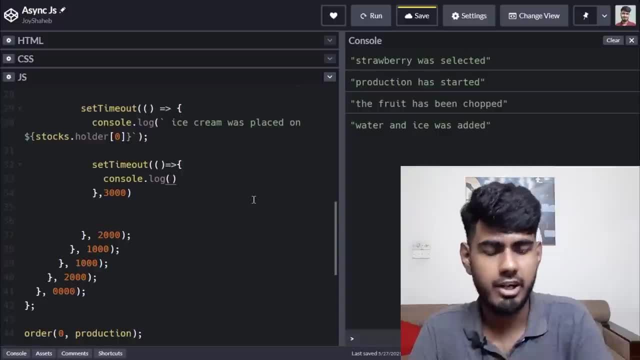 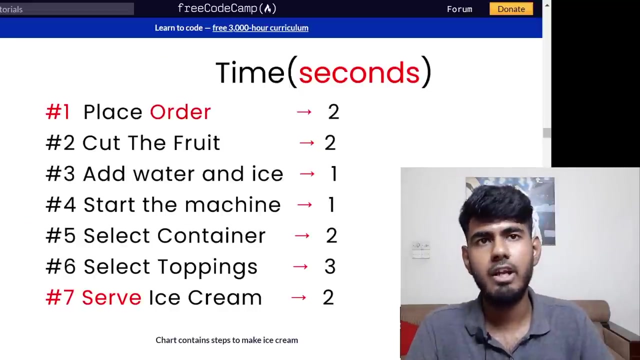 this and back ticks- okay, don't forget that. back ticks like this dollar sign, curly braces. and what we're gonna write? uh, stocks, stocks, dot toppings. we have that s at the last toppings. and then this square brackets. we're gonna write zero control s. and what's the last step? we're gonna serve the. 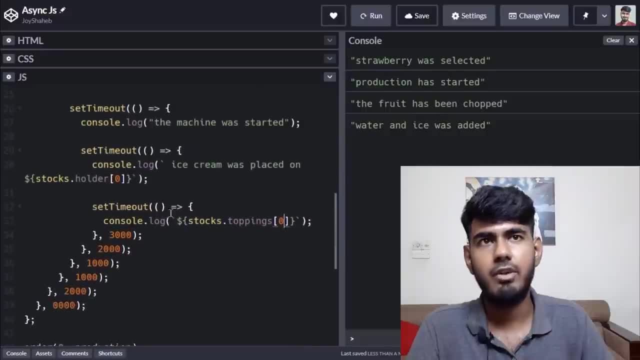 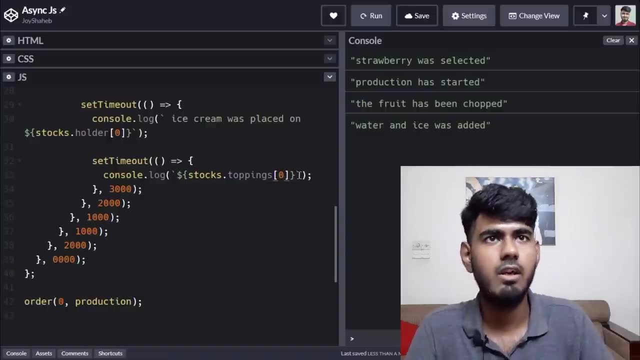 ice cream. okay, so in order to serve that ice cream, come over here, okay, where we have written this: oh, this is just plain chocolate. i forgot to write more text. okay, so stocks dot toppings, which is the chocolate was added. okay, as toppings like this. okay, and over here, give some spacing, write. 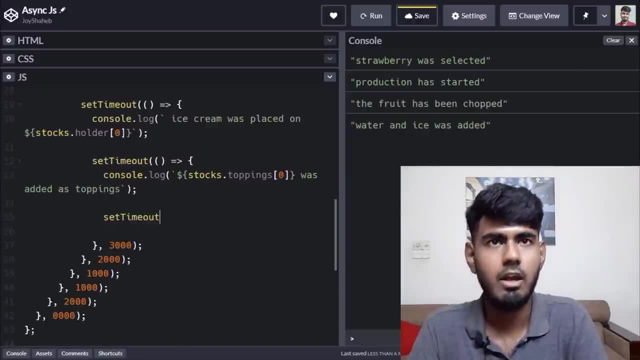 another set timeout function: okay, set timeout, and over here, um, we're gonna place in arrow function like this, and over here we're gonna place an arrow function like this: okay, and over here we're gonna like this. and then we're going to set the time which takes how many seconds to serve two seconds. 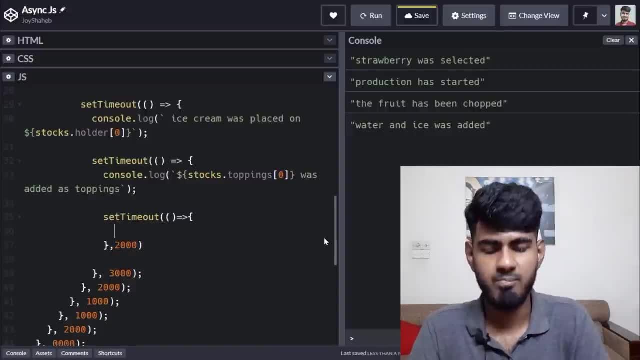 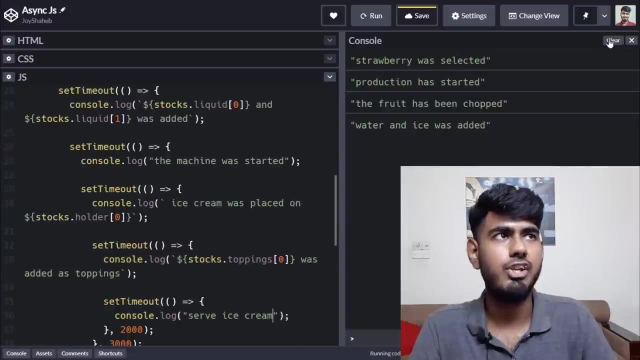 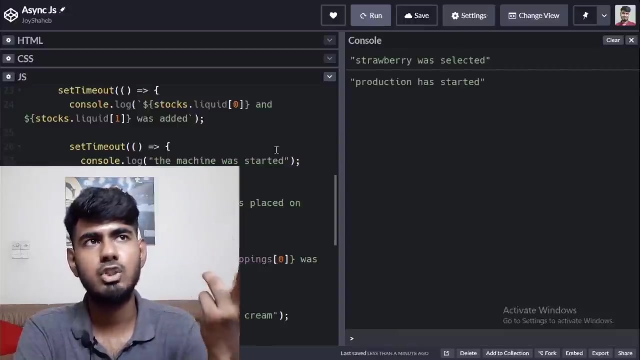 okay, two, one, two, three. console dot log. uh, then, double quotes serve ice cream control s. okay, now clear the console over here. so now run the code. let's see what happens. okay, strawberry was selected. production has started. fruit has been chopped, water and ice added. the machine was started. ice cream was placed on cone. chocolate was added as toppings. 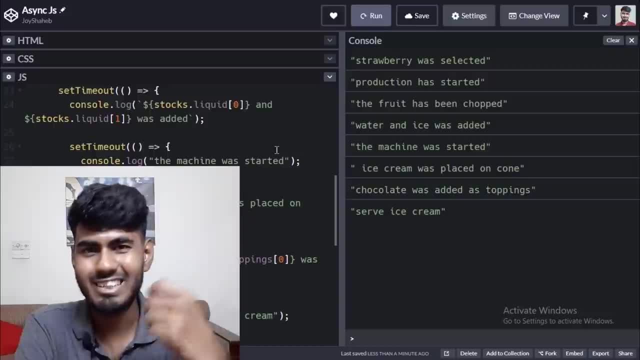 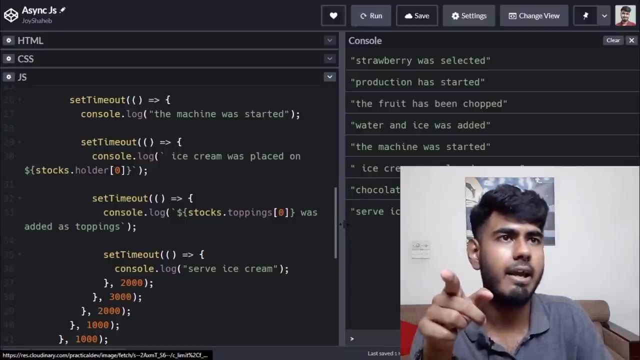 then we're gonna serve the ice cream, then we're gonna take the money and buy ourselves a lambo yay party. okay, now we have completed our process, the callbacks. but look at, look at this, what have we created? let me expand this and let me show you what we have created. it is called a callback hell. 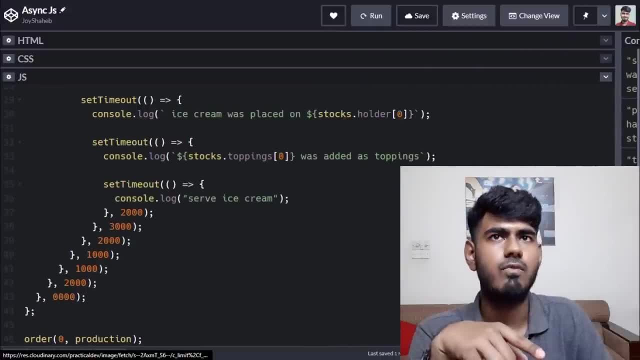 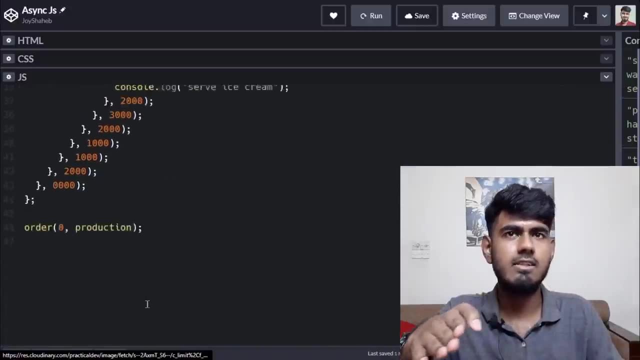 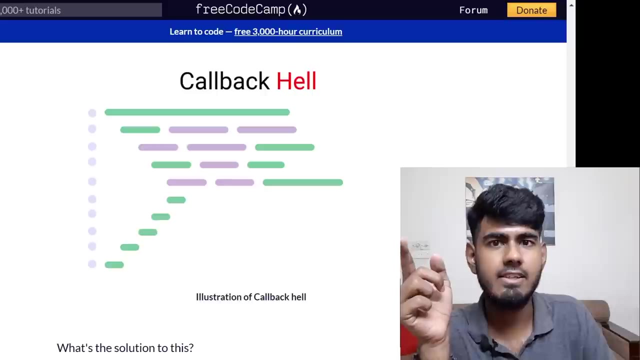 okay, look at here, look, look at this format of how it is going. okay, look, look, look, look like this. and then it is ending like this: this is called a callback hell. what is it called callback hell? let me show you the format. the callback hell looks something like this. look at this format over here. 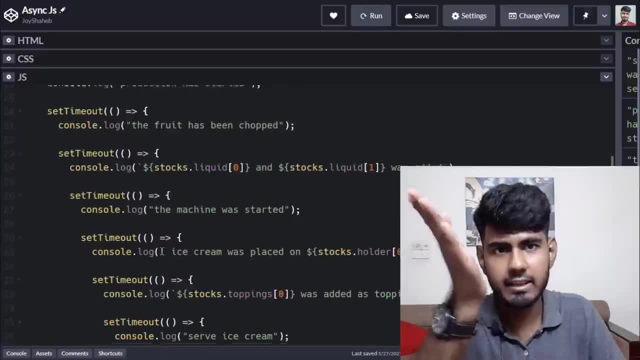 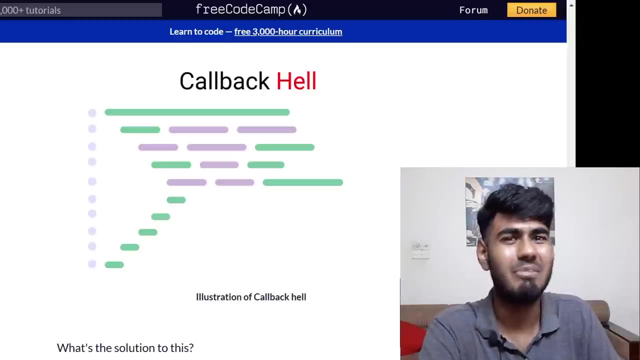 and look at our code over here. it looks similar. it looks like this: look, it looks like a christmas tree. you can also call it the christmas tree of hell, because- why not? i know, i know, i know that callbacks are very confusing and it is a hell. so what's the solution? 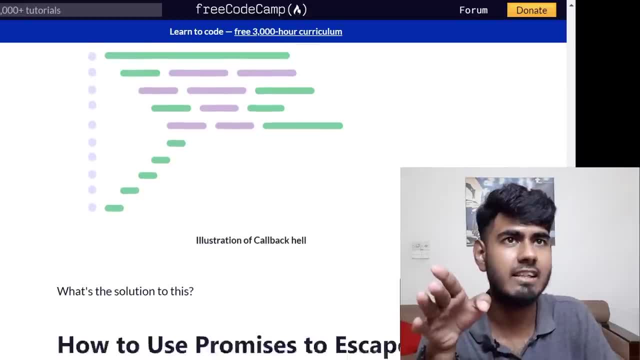 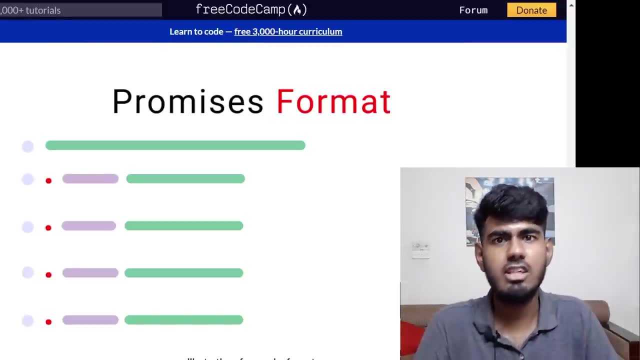 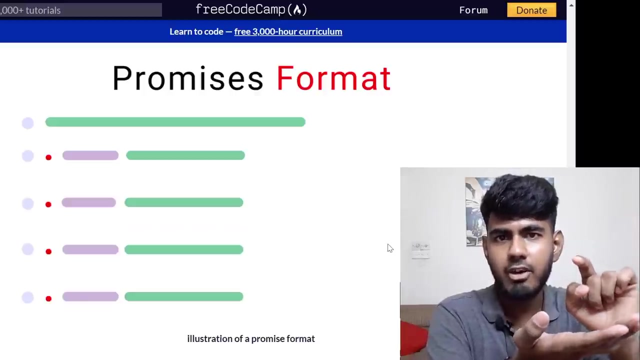 of callbacks. we have promises, and promises looks like this: look, this is the promises. it looks very clean, very neat. so let's compare again: this is our callback hell and this is our promises. look how clean it looks. the thing works like this. callbacks make relationships parent children, grandchildren, grand grandchildren, grand grand grandchildren, grand grand grandchildren. 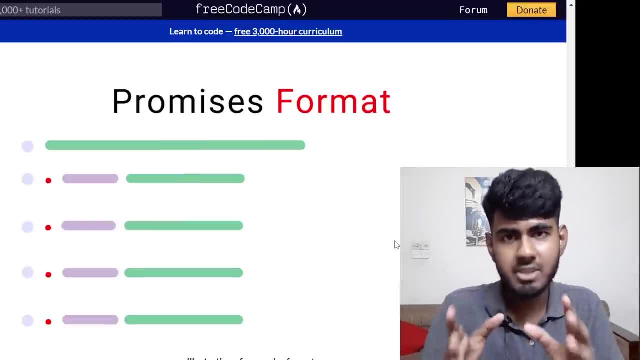 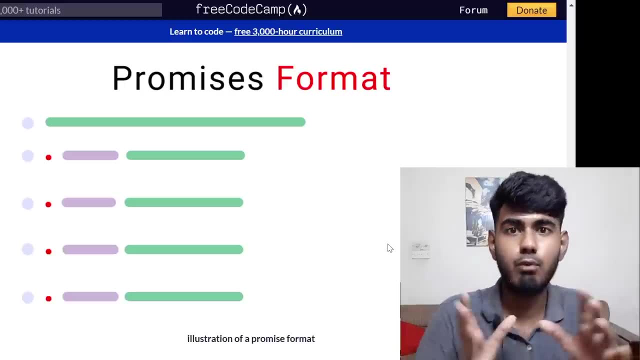 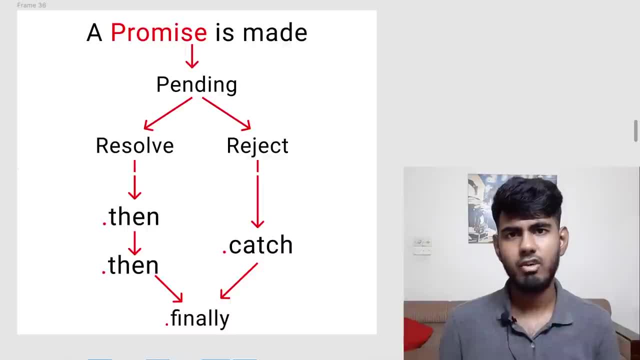 our promises. in order to understand the promise, first of all you need to understand the promise cycle. so this is the diagram i made about the promise cycle. first of all, a promise is made. what promise do we make to our customers, sir? we promise that we are gonna serve you ice cream. what? 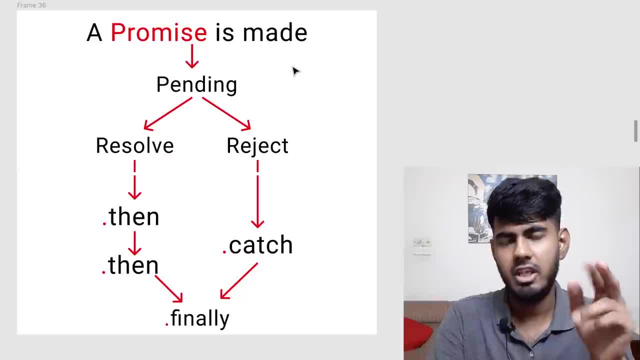 ice cream. we promise we're gonna serve you ice cream. so there are two parts of this promise: either it will be fulfilled or it will get rejected. okay, so here, first of all, it comes to this stage, the pending stage. every customer, when they come in to our shop, we promise we're gonna serve you ice cream. so our customer enters our shop, sits on. 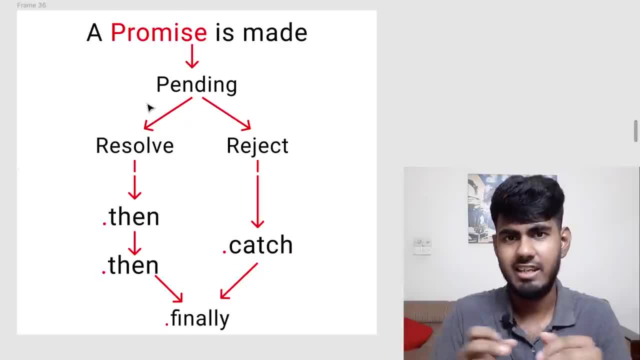 the table, looks at the menu and he or she didn't order anything. he's just sitting over there, so this stage is called the pending stage. he didn't order anything, just sitting over there, so this is the pending stage. nothing is happening. we didn't take the order, we didn't start the production. 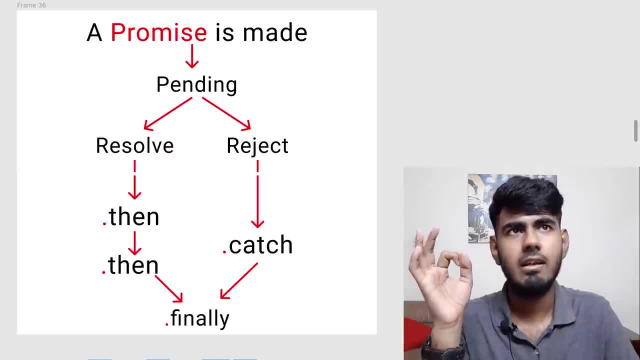 okay, and now let's say that the customer has placed an order. he wants mango ice cream. if we have the mango on our stock, then we can go to the next stage, which is we can resolve the promise, which means that we can serve ice cream to our customer, but if we don't have the mango, 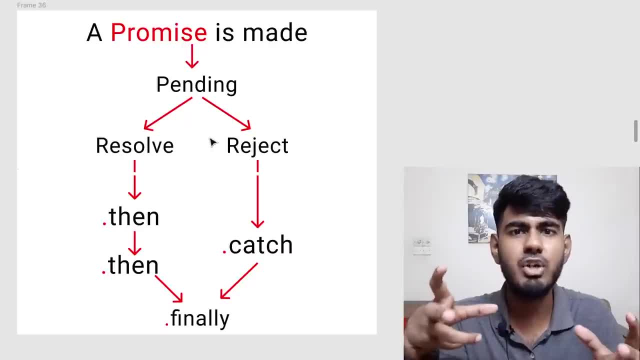 then what will happen is we have to reject it by saying: yes, sir, we don't have mango at our stocks, we are very sorry. so let's say that we have mango on our stocks. what will happen is it's gonna get resolved first of all, and then after that what will happen is we have seven steps to make ice cream. 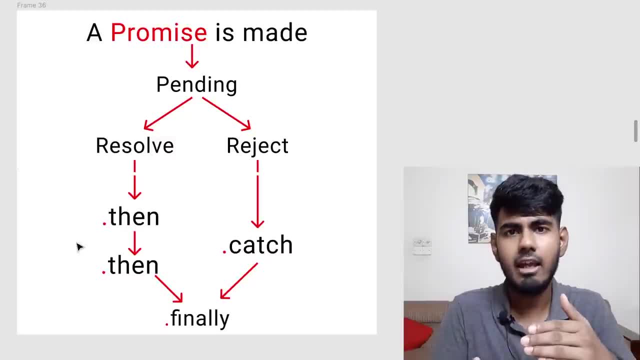 or no. we have seven steps to make ice cream and it will follow like this: first of all do this, then this, then this, then this. like this: in total, there are seven thens, or six thens, depending on the circumstances, depending on the situation. don't worry, we're gonna write code. 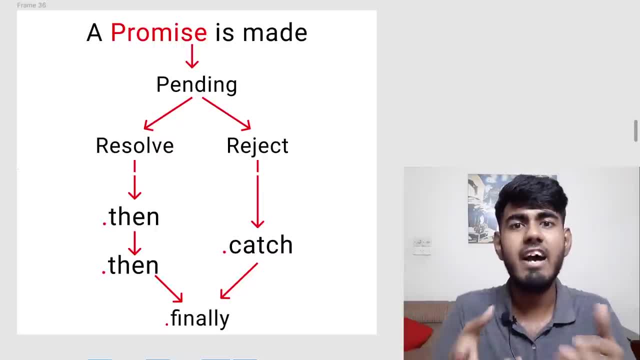 and see how this thing works. once that's done, we can serve ice cream to our customers, but let's say that we don't have mango. what will happen is we have to pass through this reject stage, and then we are going to write a sorry note. we're going to say: sir, we're very sorry, we don't have this on. 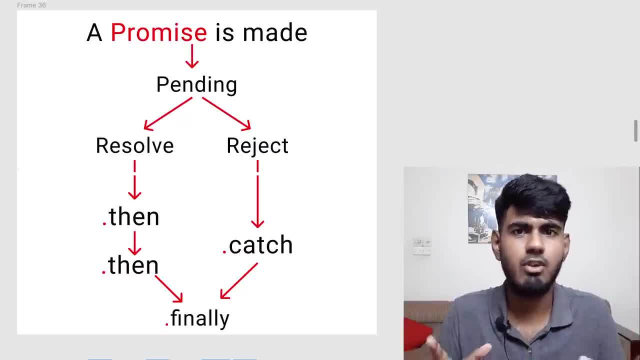 our stock. we sincerely apologize for the inconvenience and once either we get resolved, either our promise gets resolved or rejected. this, finally, will always run. let's say that we serve zero customers. at the end of the day, we have to close our shutters. i mean, we have to close our. 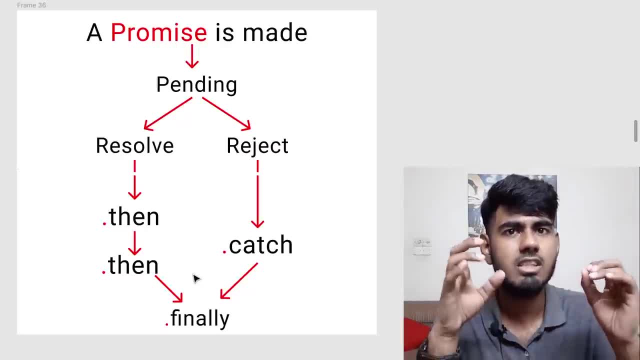 shop, but let's say that at the end of the day, we served hundred customers, 100 customers. we still have to close our shop, right, because the employees has to leave, we have to leave. this is the finally handler. don't worry, we're going to discuss all of them in details once. 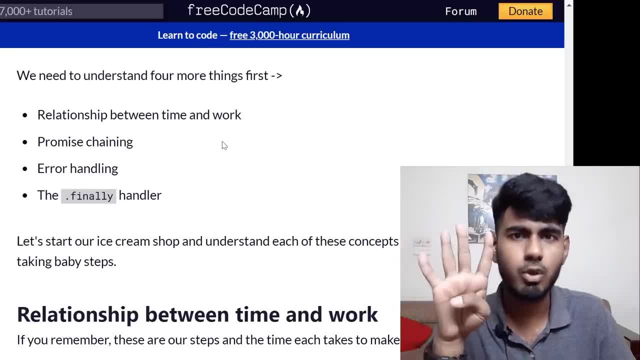 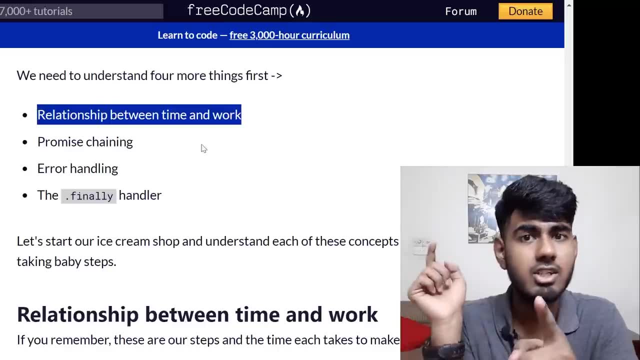 you have understood this promise cycle. we need to understand four more things. don't worry, this is very short. first of all, we need to understand the relationship between two things: time and work. what time and work? because we have this list over here. you can see that first of all, we have the work and 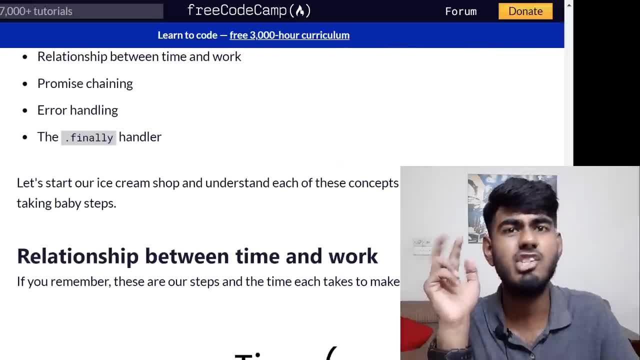 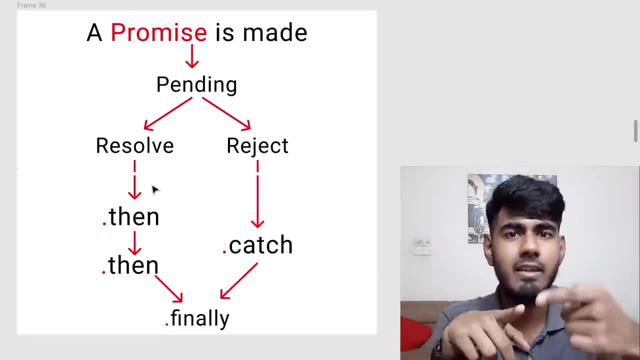 those two relationships. the next thing is the promise chaining. what promise chaining is? um, if you come over here, you can see that we are doing all the steps through, then, then, then, then this is the promise chaining, okay. so first of all, we get resolved, okay, and then it comes over here. 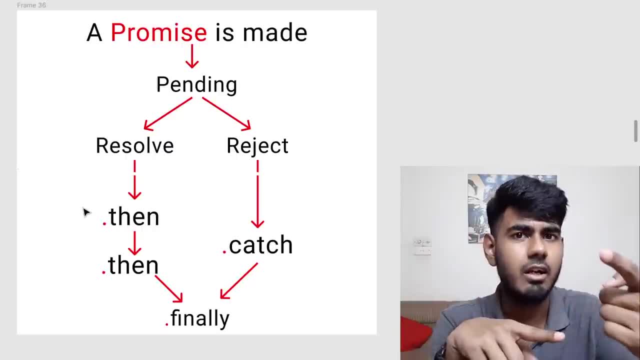 then we return it. first of all resolve, then return, return, return, return, like that. don't worry, we're gonna write code and explain, and i'm gonna explain that to you all right? so this is the promise chain error handling part. is this one? look, this catch handler is the error handling part. when we have 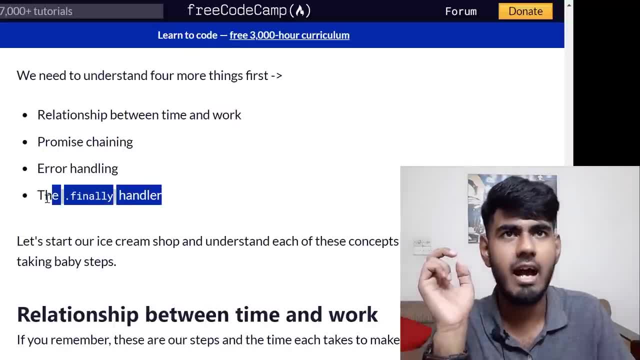 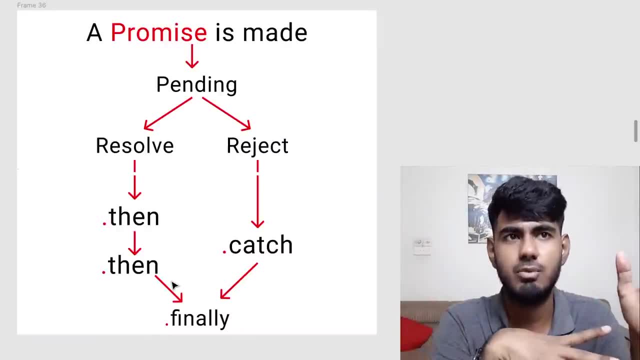 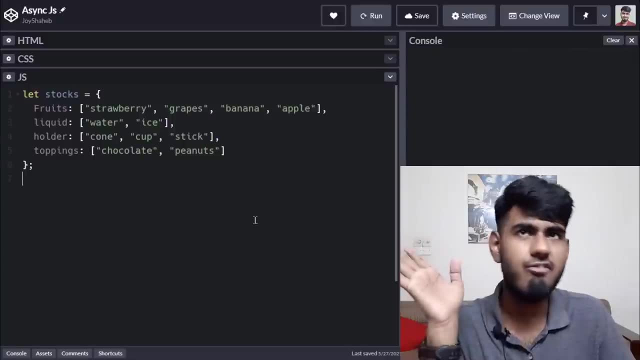 a reject, all right. and the final handler i told you earlier: right, this is the final handler. handler is gonna run whether we serve zero or hundred customers, i mean whether our promise gets resolved or rejected, all right. then come to your code editor over here. delete everything except. 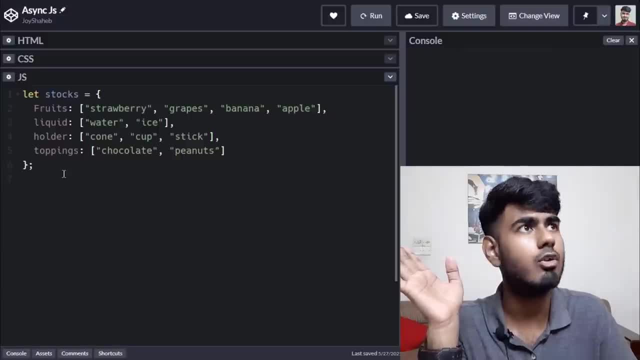 your stocks variable over here and you clear the console over here. okay, now the first thing is the absolute first thing is we're gonna create a variable named is shop open. follow me, let is underscore shop. underscore open. okay, equal to true. so what this is holding is: we are asking the question: is our shop open or closed? if it is true, we are. 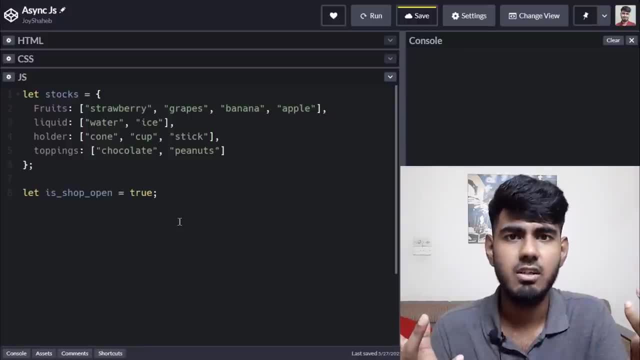 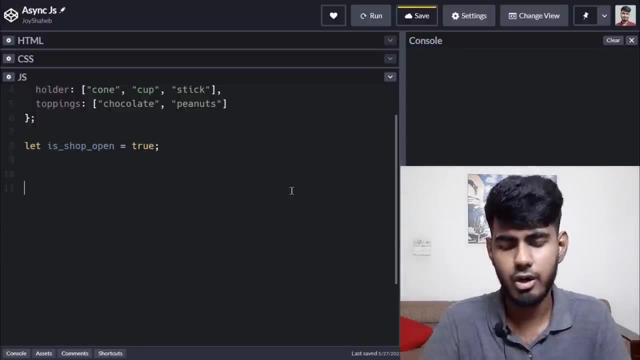 serving ice cream. if it is closed, we are sorry, sir, we are closed. okay, now we're gonna create a function, an arrow function, with the name order, like this: let order equal to brackets over here, then equal to arrow function. now what we're gonna do is: do you remember the relationship between? 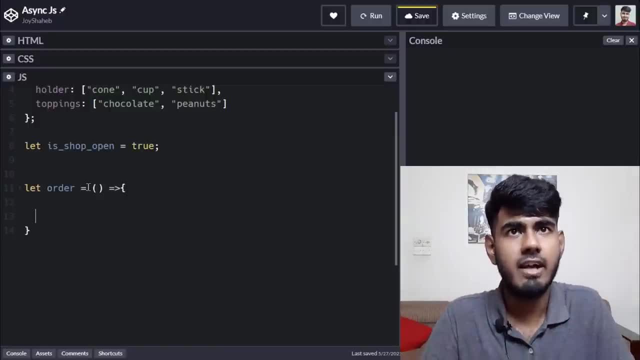 time and work that i told you earlier. we're gonna write time and work over here. okay, time over here and work over here. you can also shift the positions. you can write work first and then time. it totally depends on you. and the next thing is we're gonna make a promise. first, we made the 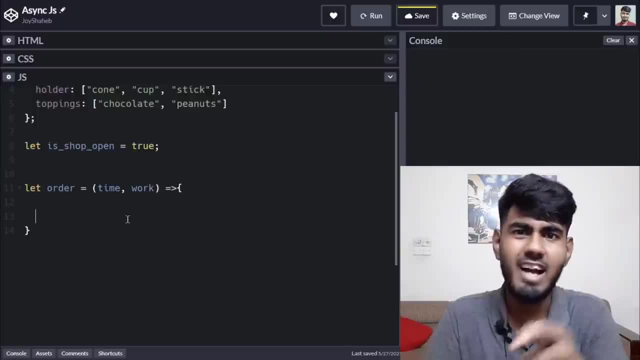 order. then we made the promise, sir, we're gonna serve you ice cream like this: follow me first of all. you're gonna write return. okay, new, then capital letter p. what capital letter? p? p r o m i s? e promise like this: look then brackets give a little bit of space so that you can understand. 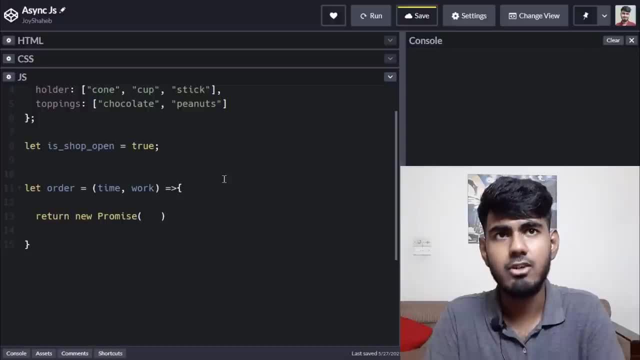 what we are writing. okay, over here, we're gonna give brackets. over here again, we're gonna create a arrow function. look like this: okay, like this. we made an arrow function over here now, press enter. now, um, inside this brackets, we're gonna pass two arguments: resolve, reject. which means that we have how many stage? three stages pending. 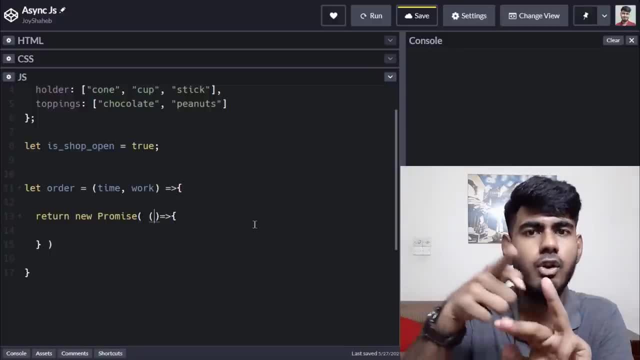 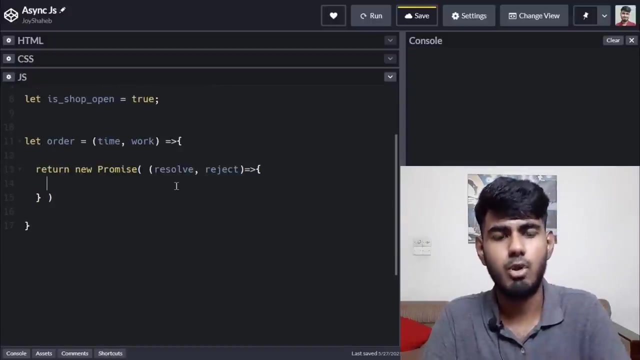 resolve, reject. we're gonna write resolve, reject. we don't need the pending. okay, now write resolve like this, resolve like this. and over here you're gonna write reject, reject like this. okay, so we made a promise. now it's time to run that promise. okay, now we have two stages resolve. 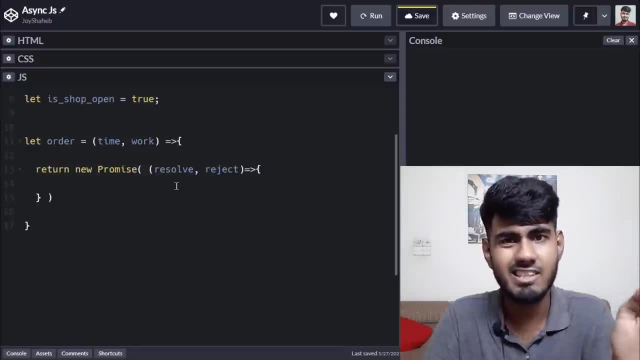 and reject. let's write an if else statement. so write um if is shop open, which means that if our shop is open, then we are gonna resolve it like this: resolve, which means that we're gonna ice cream, that our shop is open. welcome, sir, we're gonna serve you ice cream. how are we gonna? 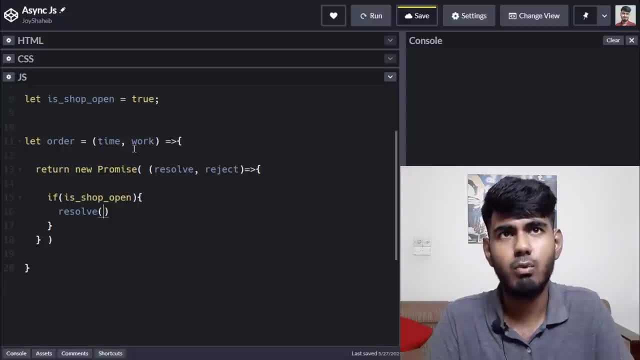 serve our ice cream. we're gonna write this work. you see this work over here. we're gonna write this work over here like this: look, we pass the work over here. which means that when the shop is open, when our customer came, we're gonna say, sir, we promise that we're gonna serve you. 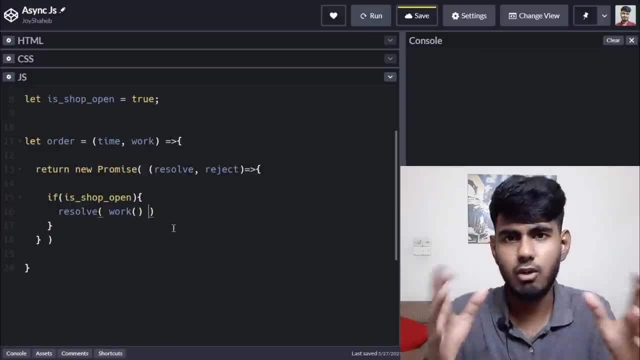 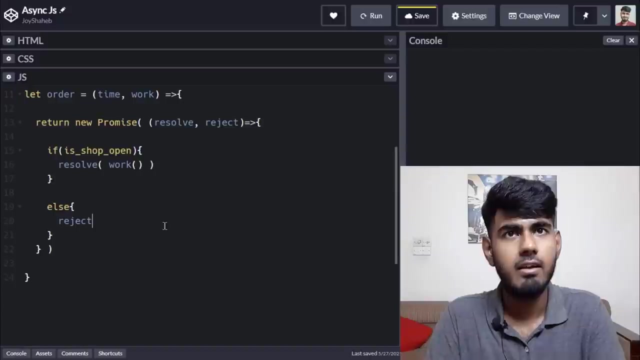 ice cream. as long as we have all the stocks and the raw materials, then we're gonna start working. all right now, if our shop is closed, then what will happen? we're gonna write an l statement over here- okay, curly braces. and over here we're gonna write what: reject, reject, like this and 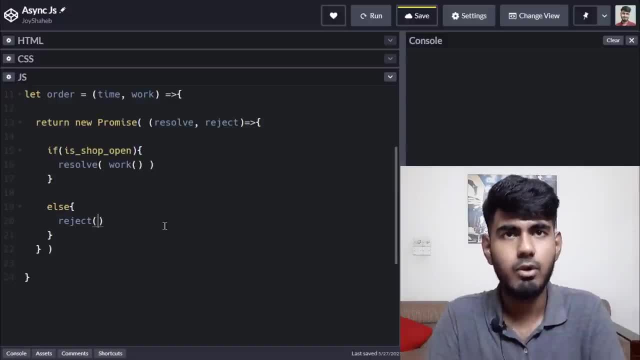 you close it like this- i mean the brackets- and over here you write console- oh sorry, console dot log. like this: okay, and over here we're gonna write our oh sorry, our shop is closed, okay. like this. so far, so good. now you can see that we have formed relationship between with, just 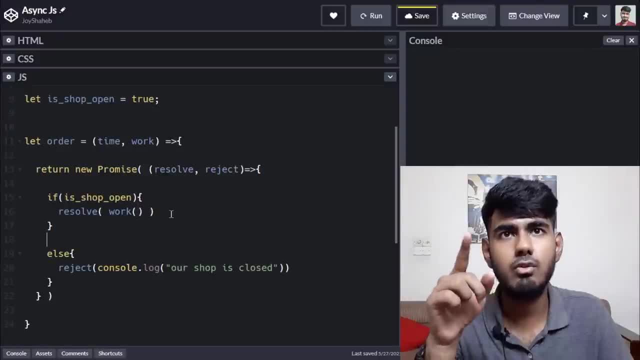 work. look, this work is over here. but we also need to form relationship between time, also along with work. so what will we use? we're gonna use a set timeout function so that we can form the relationship between our time and work. follow along with me, okay. so below this, if statement write set timeout- okay, and then brackets over here, form a. 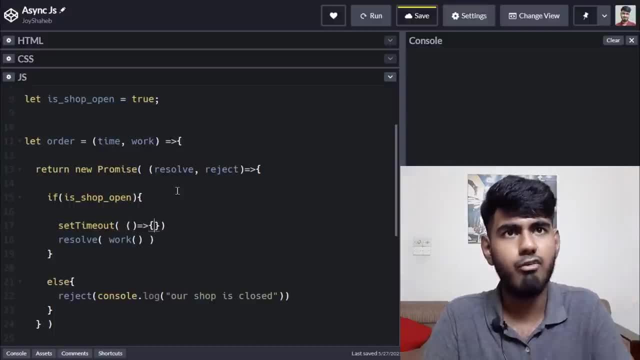 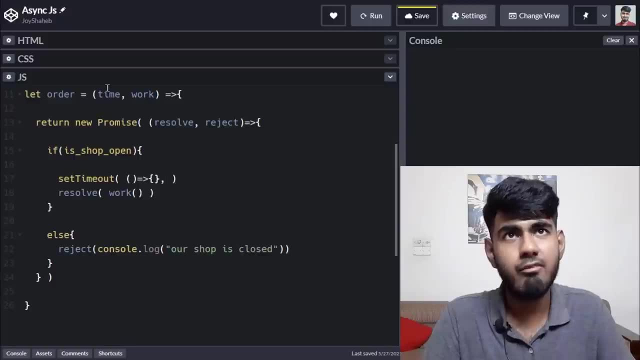 row function like this. look okay. arrow function like this. and then what you're gonna do is you're gonna put a comma over here. comma, we're gonna pass this time function- i mean the time word over here, which means that every time we need to write the order function, we're gonna place the time. 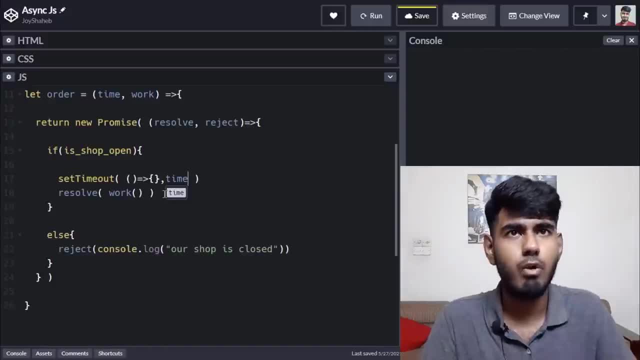 and the work. don't worry, we're gonna write it. and then what you're gonna do is you're gonna cut this result from here, control x, okay, and then you're gonna paste it inside this arrow function. now what will happen is it's gonna form a serial after one, two, three, four, five, six, seven. we have. 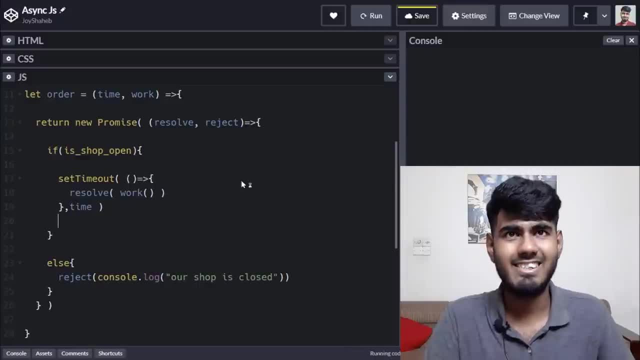 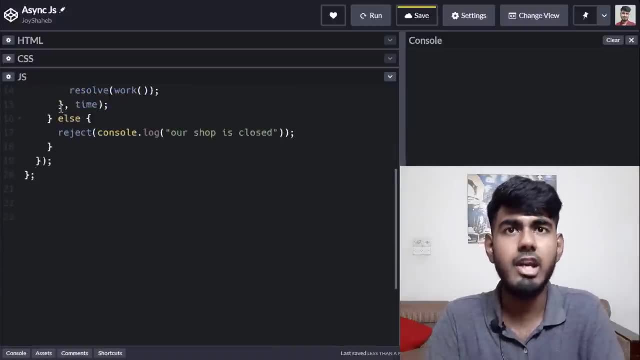 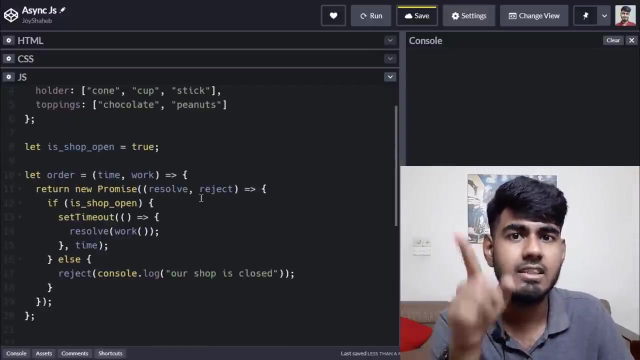 to draw seven steps. now save this code. let's test it. okay, so what is the name of our function? it's order. okay, so come at the very bottom over here you write order. okay, now brackets. now look at the first thing. what is it? first thing is the time and then the work. so how you are gonna. 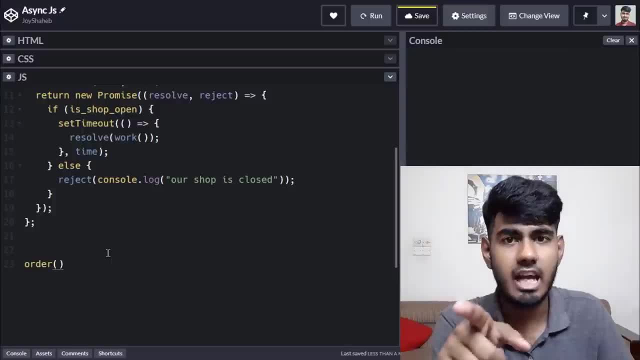 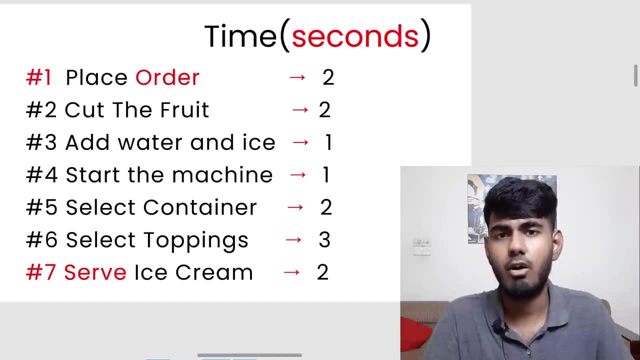 find this. follow along with me. the first thing is time. okay, so let's look at the chart. so this is our chart, which carries all the steps. first thing is we need to place the order. okay, it's gonna take two seconds in order to write that. first of all, we're gonna give the time. okay, you're gonna write. 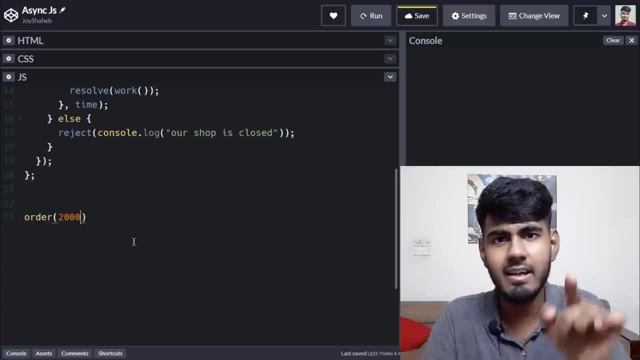 two seconds like this: two, one, two, three, two thousand milliseconds, and then a comma. comma like this: and now we're gonna create a small arrow function- look at this, okay- and then the arrow sign in a single line. you don't have to put this curly braces, you can just use directly, like this: 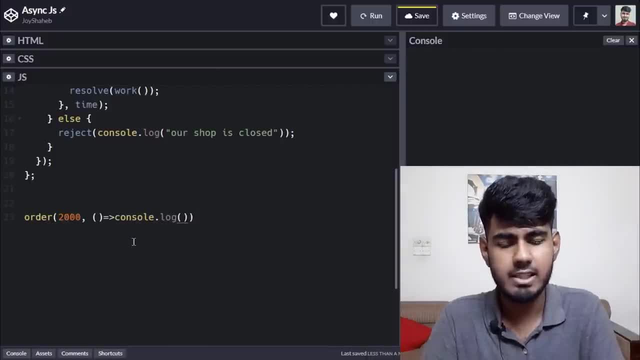 console dot log. okay, first of all, we're gonna select the fruit in order to select the foot. what do you need? back ticks, what back ticks? like this? okay, then dollar sign: curly braces like this. so what's the name of our stocks? this one, okay, stocks dot fruit. uh, let me check fruits. yes, stocks dot. 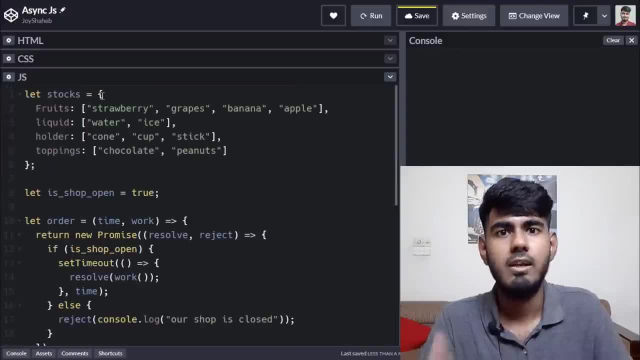 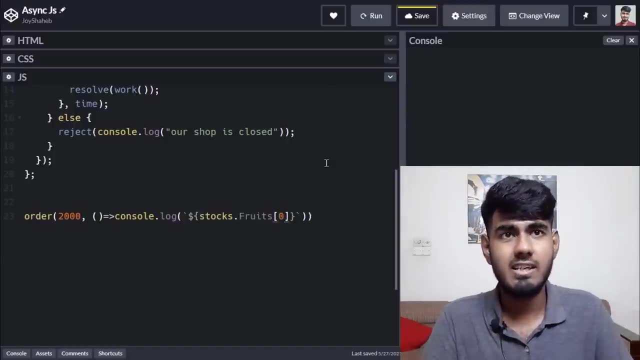 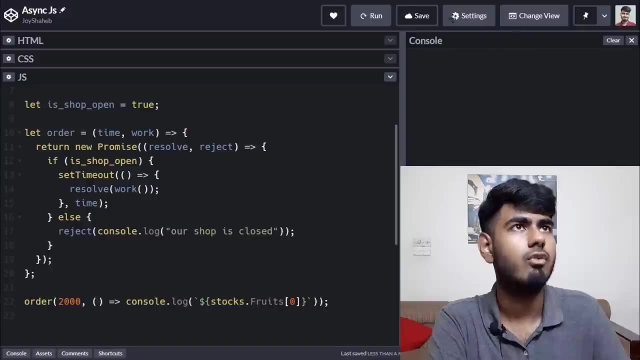 like this: and then we're gonna pick the strawberry: okay, zero this hand, uh, square brackets and then zero, like this: now let's test it: control s and then um, clear the console, save it and run it like this. after two seconds we're gonna get the result one, two. there we go, we have. 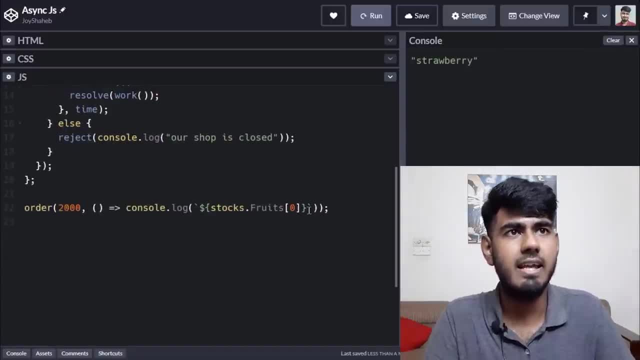 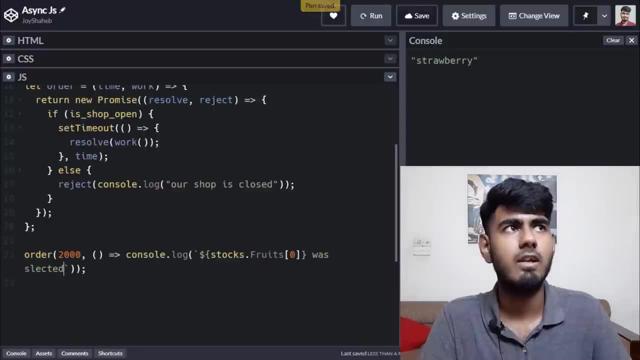 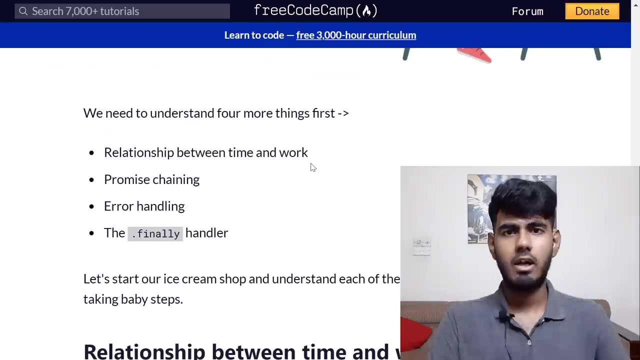 strawberry over here. now let's complete this by saying that strawberry was six selected. okay, control s clear. the console run it. one, two, there we go. we have our strawberry was selected. i hope you understood the relationship between the time and work function. this was pretty simple. now let's start discussing about the promise chaining, which is this one over here. 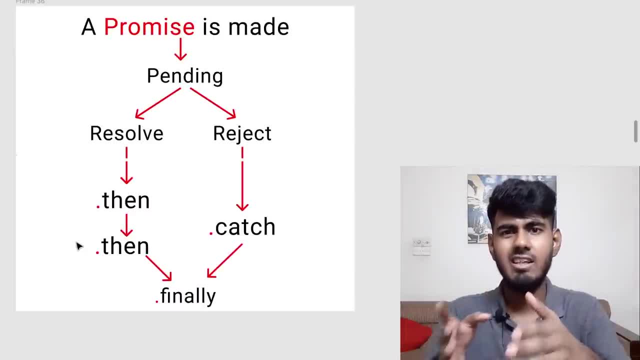 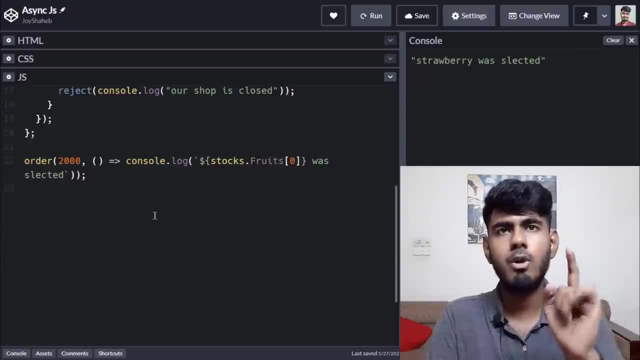 the then, then, then, then part. first you have to do this, then this, then this, etc. let's come back to the vs code over here and, at the very bottom, want to work with the promise chaining. you cannot have anything between the first call of the order and then your then handler, like this: if you want to do promise chaining, you have to do this dot. 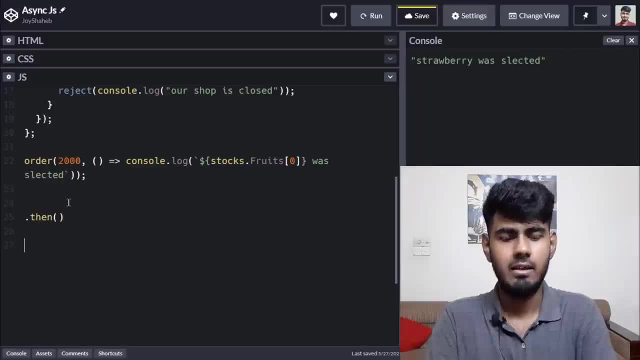 then okay, then dot, then dot, then so on and so forth. oh, i made a spelling mistake, my bad. then you cannot have this semicolon over here, okay, so just remove the semicolon from there. okay, now it's going to work perfectly fine. you can have 100 lines of spaces like this, and it's still going. 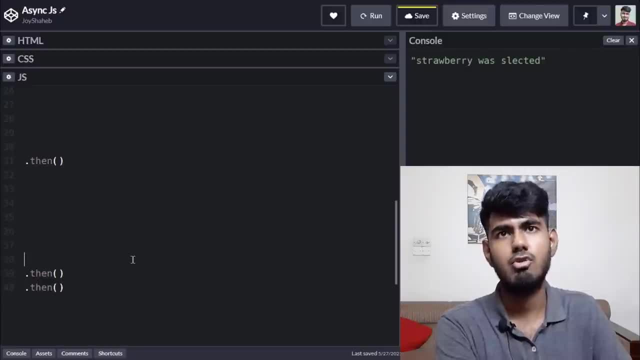 to work like this, but for this tutorial i'm going to have just two spaces, so that it can look very good and tidy. okay, so, like this, look at that. it looks quite good. and now, in order to write, i mean in order to give an instruction inside that, then let's look at our chart. so this is the chart. 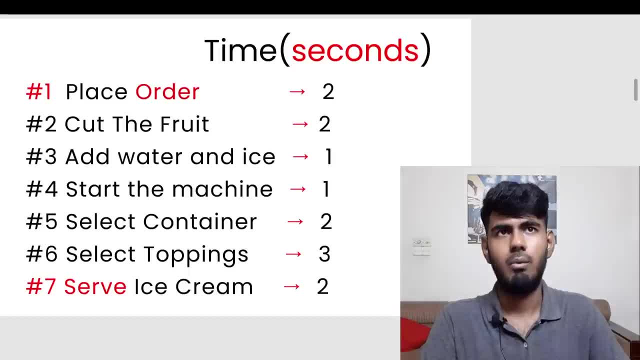 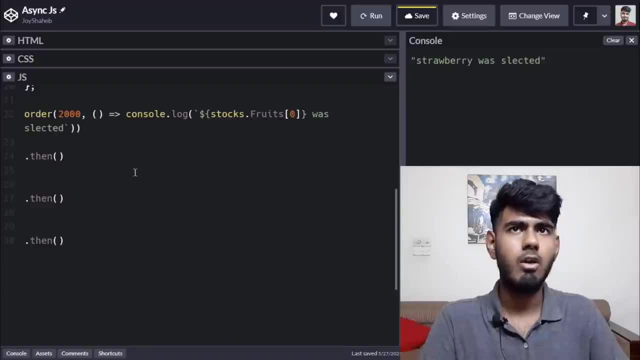 cut the fruit and it's gonna take two seconds. okay, now come back to code pen and over here, before cutting the fruit, let's give a call to start the production. how do you do this? first of all, write an arrow function like this: look, okay, arrow sign. you can also write it in a: 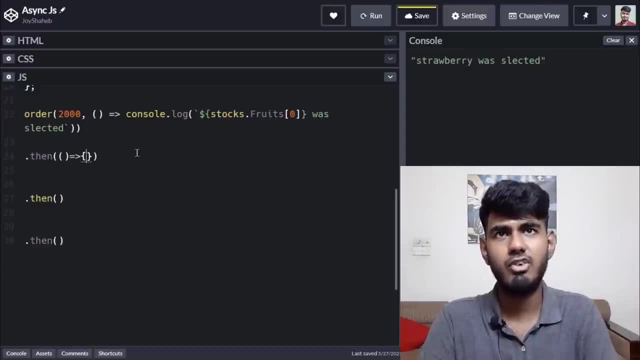 single line, but i'm gonna give curly braces over here and then you're gonna return it. you have to return it, otherwise it's not gonna work. the first part is resolve, then return, return, return, return, return, return, return, so on and so forth. if you don't write the return over there, then it's not. 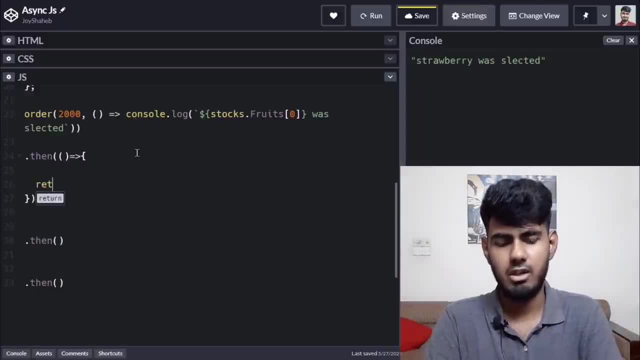 gonna work. okay, follow along with me. you write return over here. okay, then order what was that? order the name of our function? okay, like this look, and then you're gonna place what time first in order to start the production. it takes zero, second, zero, zero, zero, zero comma. 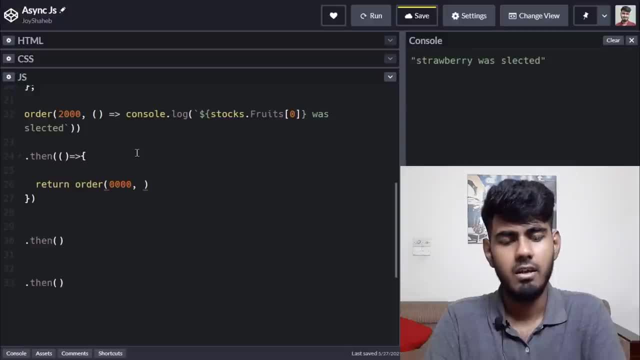 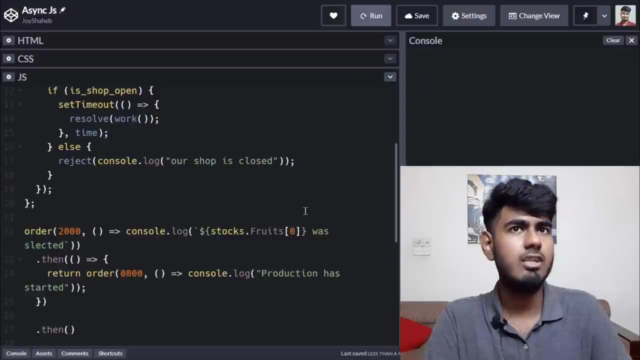 and then you're gonna write a function over here- okay, arrow function like this, console dot log, like this. and then we're gonna write over here: production has started, production has, sorry, started, okay, save it. and then we're gonna clear the console, let's run it. so we're gonna get this one after two seconds and this one immediately. one, two, there is our. 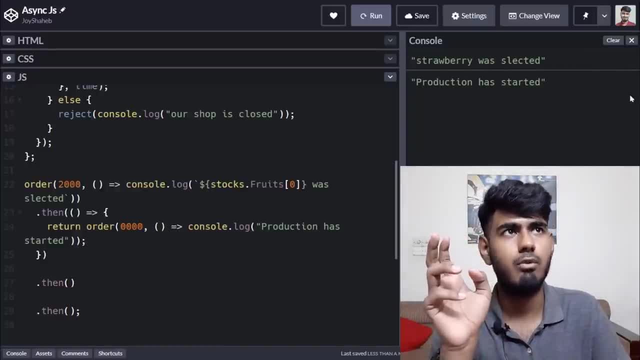 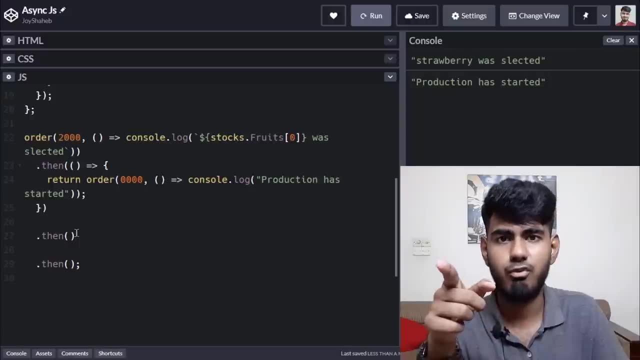 strawberry was selected and production has started. it took two seconds, and then we're gonna write over here: okay, and this one took just zero seconds. okay, now let's write the next step. what was the next step? we need to chop the foot. it takes two seconds. i mean, cut the foot. okay, let's follow the 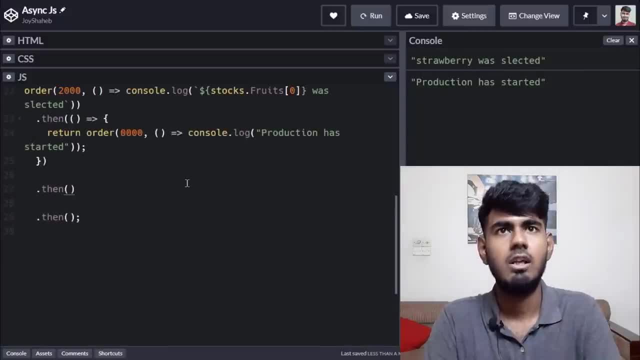 same process. okay, over here, you're gonna write an arrow function like this: equal to. then this arrow sign: curly braces right over here. what return? what was it? return? return like this: okay, order, we're gonna write uh 2000 over here, which means two seconds. okay, equal to. like this. then console dot log: um, what was it? we're gonna cut the foot, okay. 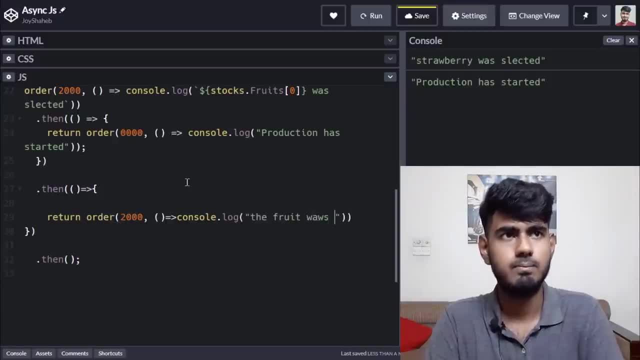 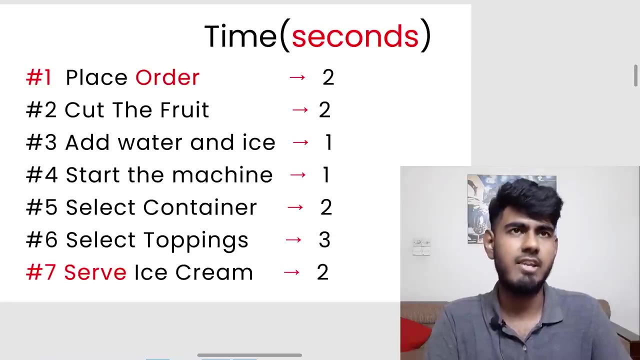 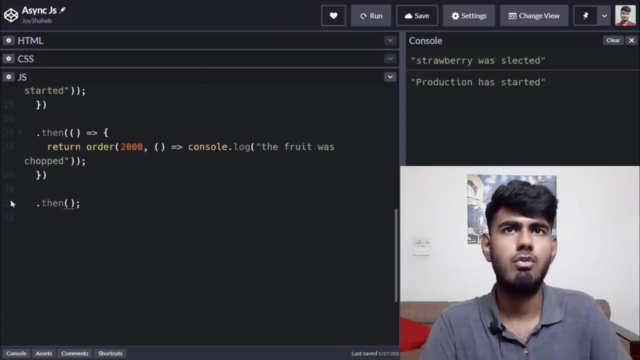 the fruit was chopped. sorry, control s. okay. there we go, following this chart. let's complete our process, okay. next is we have to add water and ice. let's go and do it so over here we're gonna follow the same process. let's actually um copy this code from here, okay, no, no, look, let's not copy the code, okay. 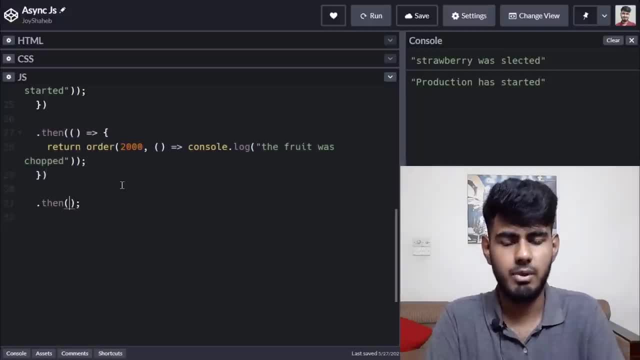 let's just do it manually so that you can learn it. okay, follow along with me. arrow function over here, okay. return, return order: um is gonna take how many seconds? one second, okay. one, one, two, three, okay. then this sign, which is um the arrow function, give a curly braces over here, okay, and inside over here. you know right. 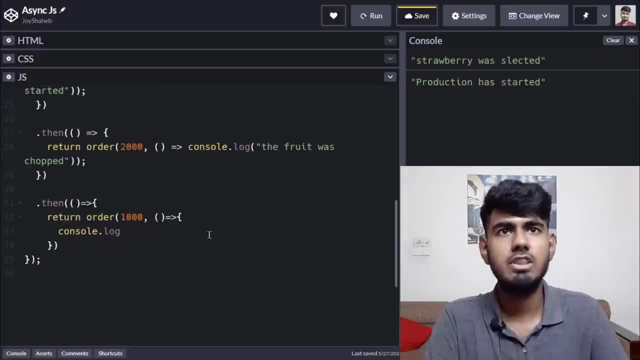 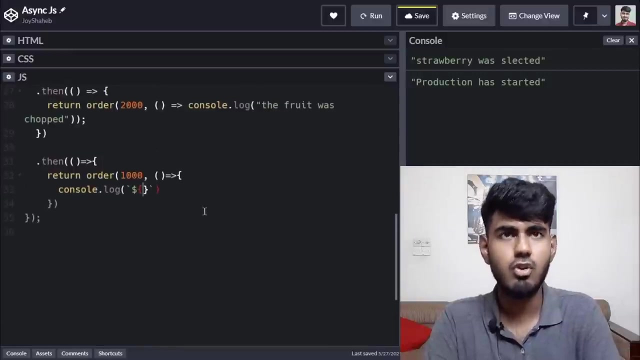 console dot log. um, what was it? backticks. okay, then dollar sign: curly braces. that is because we need to select what our liquid, which is water and ice. okay, stocks dot liquid. come at the very bottom over here. you write stocks dot liquid, like this, and then zero, in order to select what the water. 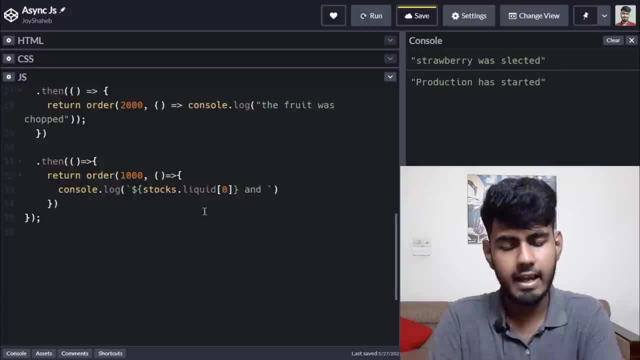 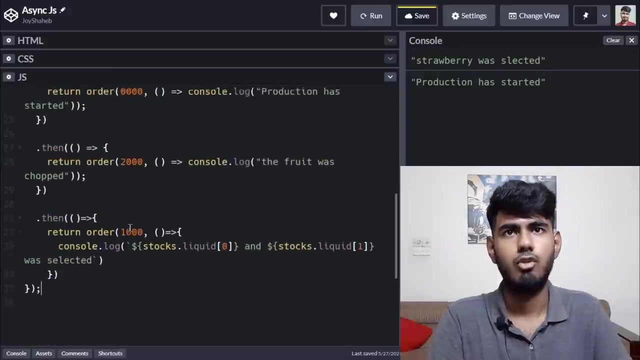 okay, and over here, right and a. again, you write dollar sign, curly, braces, stocks, dot, liquid, and then what was it? one? okay, so water and ice was selected like this. there we go and remember this. this is very crucial. you cannot have semicolons between tens. okay, remove this semicolon from here. i mistakenly wrote it. okay, space, and then. 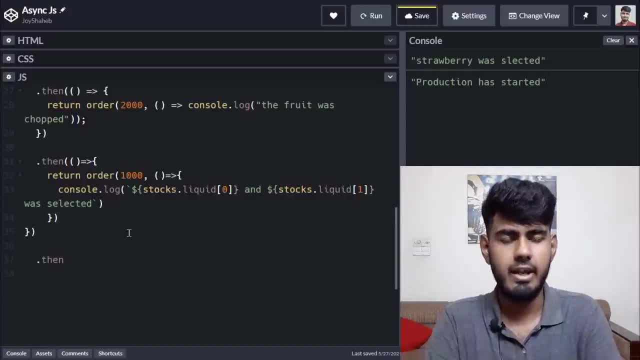 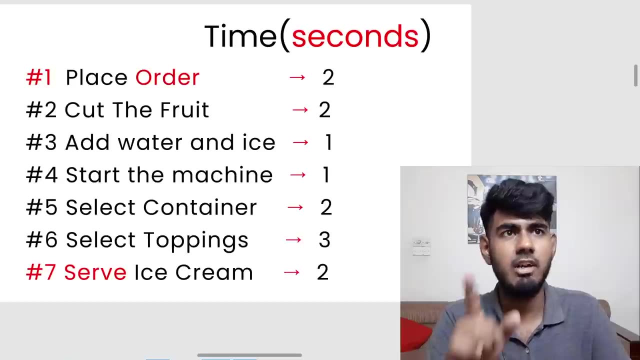 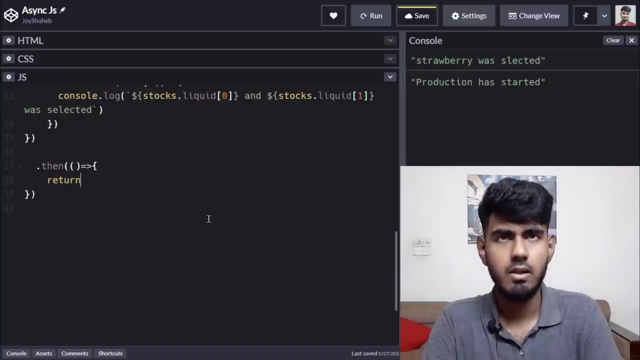 over here we're gonna write 10 brackets arrow sign like this: curly braces. what's the next step? let's see we need to start the machine in one second, okay, so write return, sorry, return, order, square brackets. then, um, first of all you need to write the time: okay, one seconds, like this arrow sign. 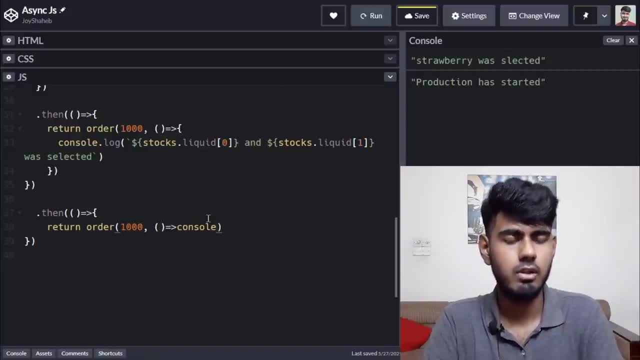 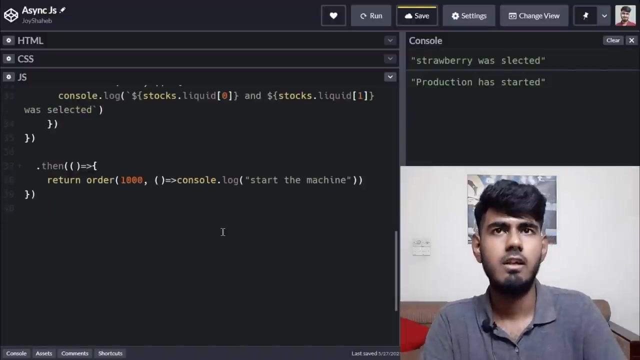 like this: console: dot log: um. start the machine. like this: next step is: we need to select the container. we're going to select the cone. okay, in order to do that, come here dot 10. okay, then arrow function like this: return order: it takes how many second, two seconds to select. 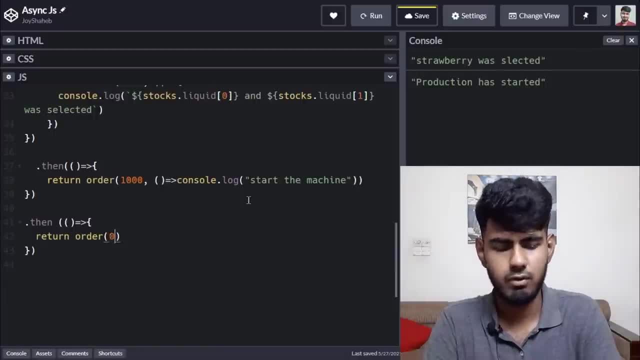 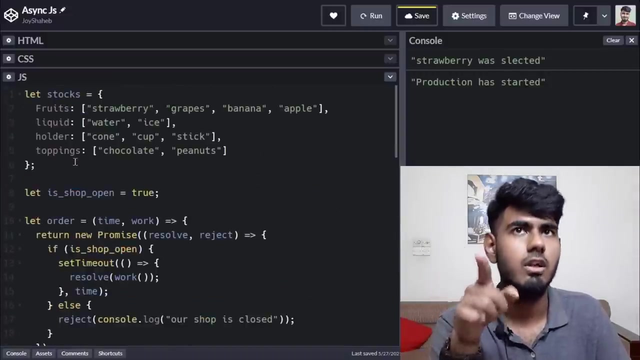 the comb. okay, sorry my bad, oh, ah. then the arrow function over here. curly braces. inside you're gonna write console, a log, um, what was it? um, back ticks. okay, then dollar sign. curly braces over here you're gonna write stocks dot, which was it? let's see top and a holder, holder, and then zero, because the cone is over here. okay. 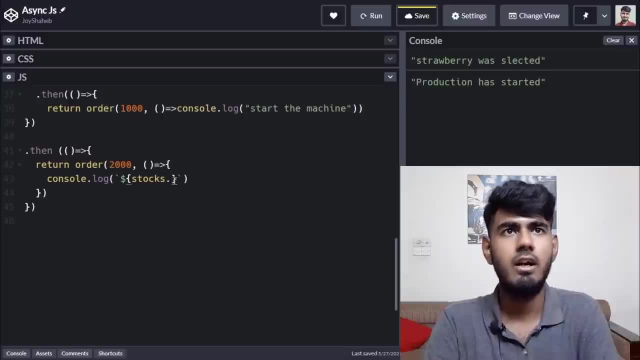 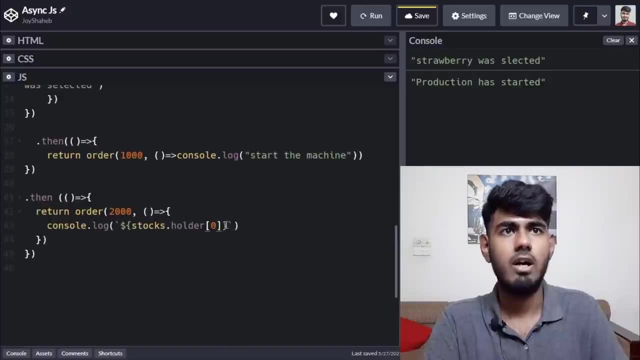 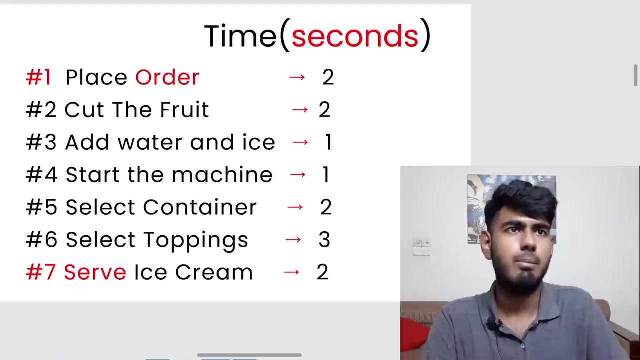 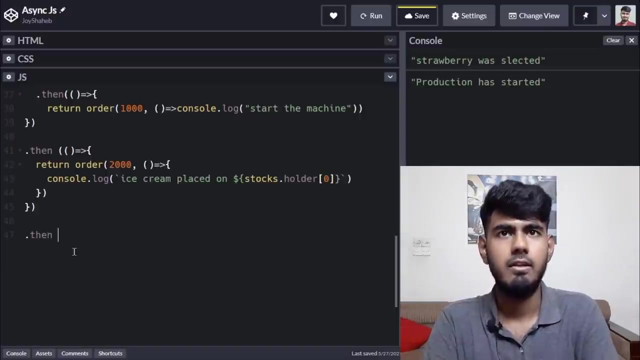 at the very bottom holder h-o-l-d-e-r, like this square brackets zero. okay, then you're gonna write: uh was ice cream was placed on this holder? okay, so ice cream placed on it translates to ice cream placed on comb. okay, so the next step is select toppings. we're gonna pick chocolate dot 10. okay, then this sign: 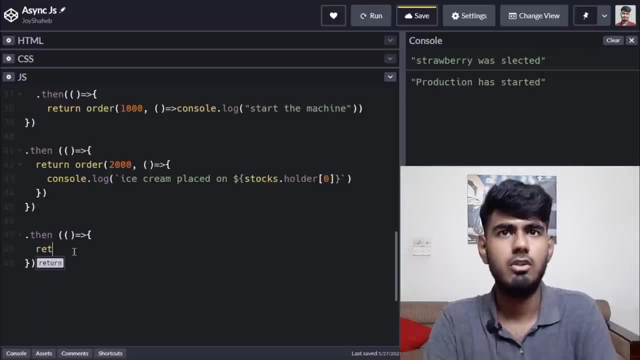 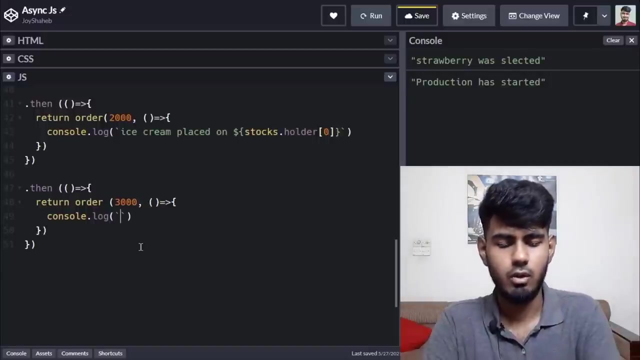 i mean the arrow function return, sorry, return order, uh, three seconds, because chocolate takes time to melt, right. so equal to uh. arrow function, then console the log, then inside over here back ticks. okay when you back ticks, okay, don't forget dollar sign. curly braces. over here you write stocks, dot toppings. 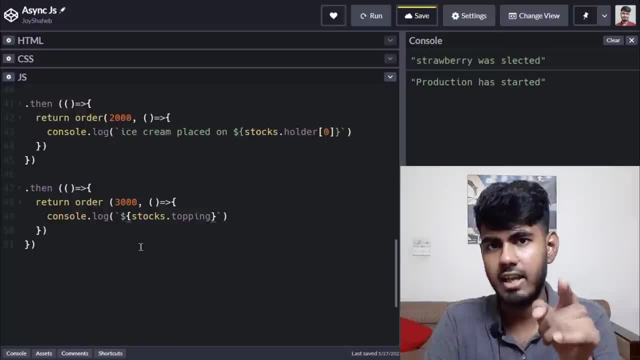 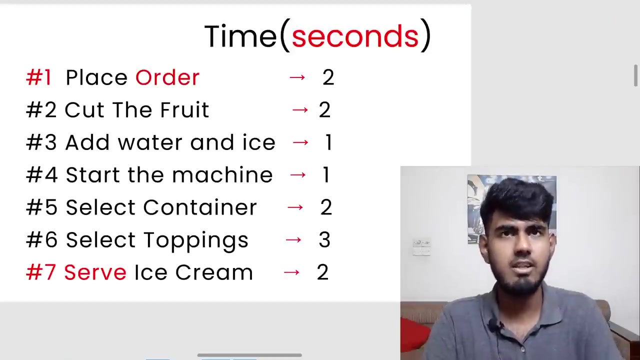 t-o-p-e-i-n-g-s, don't forget the last s top pins. and then square brackets. over here we're gonna write zero chocolate was selected like this, so we're almost done. then we're gonna serve the ice cream. serve ice cream. we're gonna write um dot 10: okay. 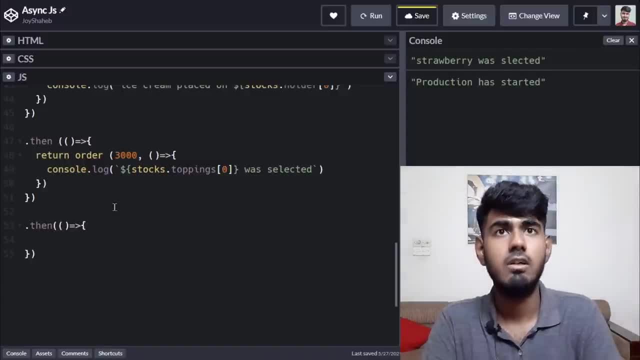 like this: um, return order. we're gonna write how many seconds it's gonna take. it's gonna take two seconds, okay, equal to curly braces. uh, we don't need curly braces, actually, we can write it directly: okay, one, two, three. like this: uh, like this: equal to this. sign the arrow function and then 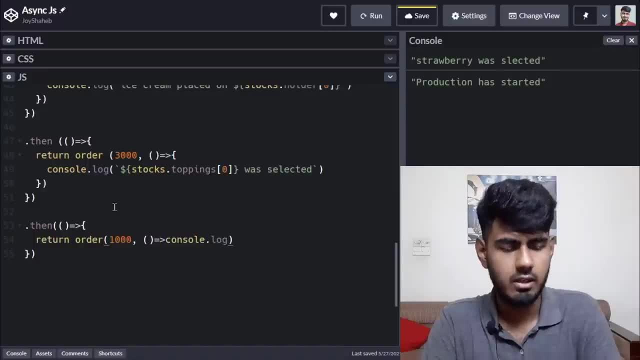 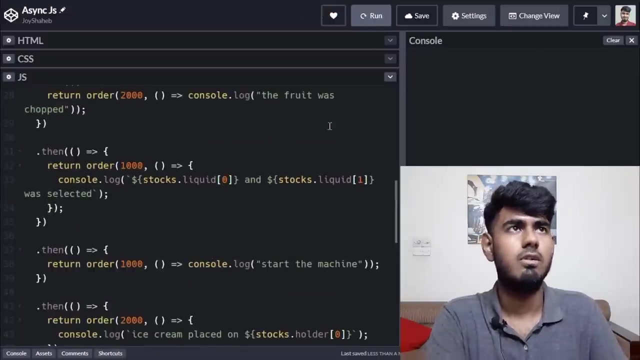 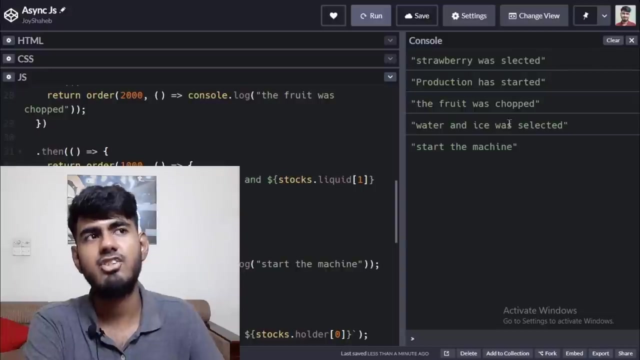 console dot log. okay, double quotes. ice cream was served, control s. there we go. we completed our process. now let's run our code. before that, clear this console, run it, let's go. strawberry was selected. production has started. the fruit was chopped, water and ice added: start the machine. ice cream plays on cone. 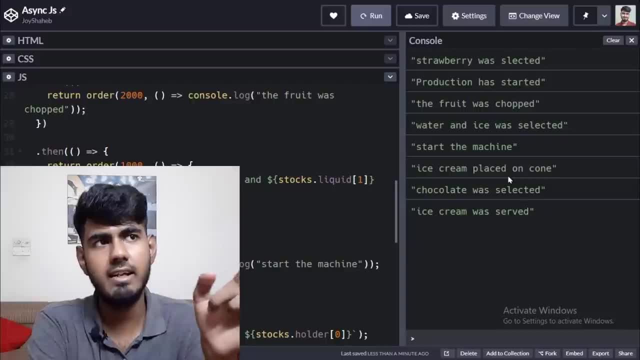 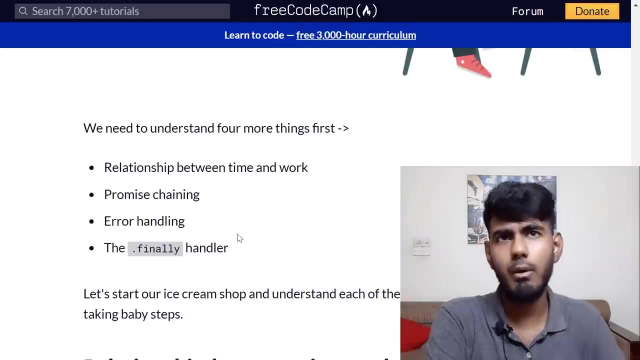 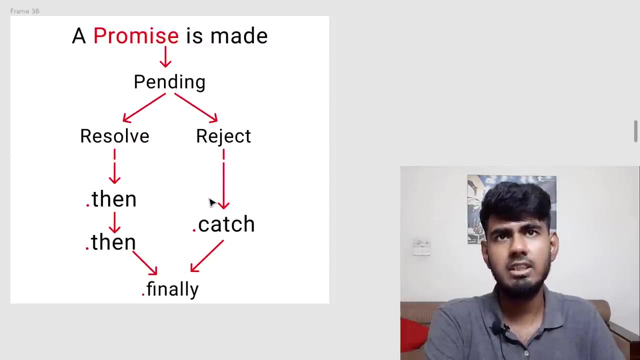 then, where is our chocolate? there is our chocolate. chocolate was selected, ice cream was served. give us the money and let us buy us the lambo. yay, now is now it's time to understand the error handling part. okay, which is this one over here, the catch handler. in order to understand the catch handler, 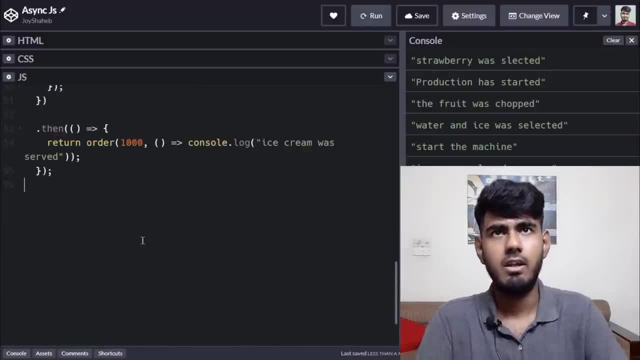 come at the very bottom over here, okay, and you write: uh, oh, don't forget to remove this semicolon form here, otherwise it's not gonna work. you write dot catch like this, okay. like this. then write an arrow function like this: okay, equal to curly braces, like this, and over here, right, consolelog. 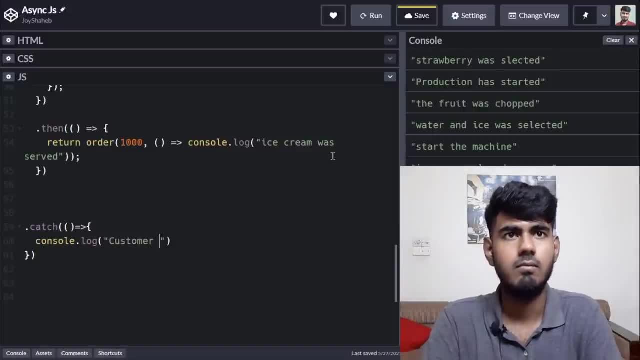 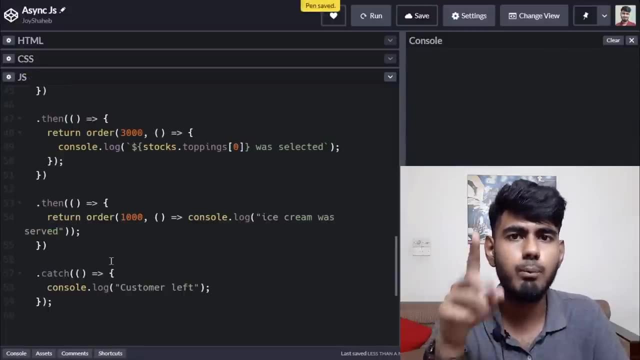 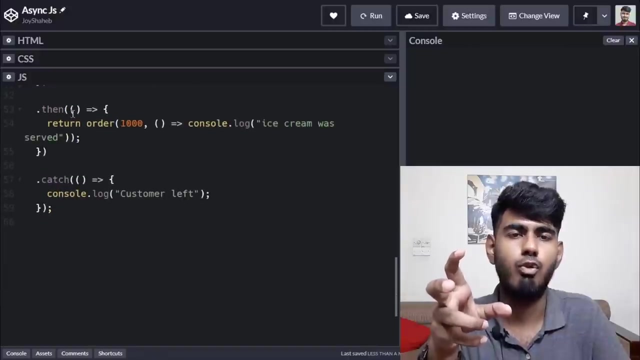 customer left, like this control s, and then clear the console. now, this catch will only work. when our promise is rejected, i mean, when we cannot serve ice cream to our customers, then this catch, then this catch will work. let me show you. okay, if you can read, if you can remember this variable at the: 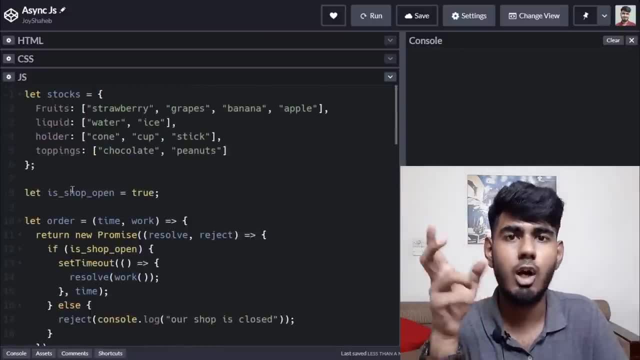 very top of the box, this value here. it just left the address not on active and if you can see here it's correct, it is not on active. it is not worked at all. see now what happens here: consideration to over here, below the stocks, which is is shop open. it is true. let's convert it to false and let's 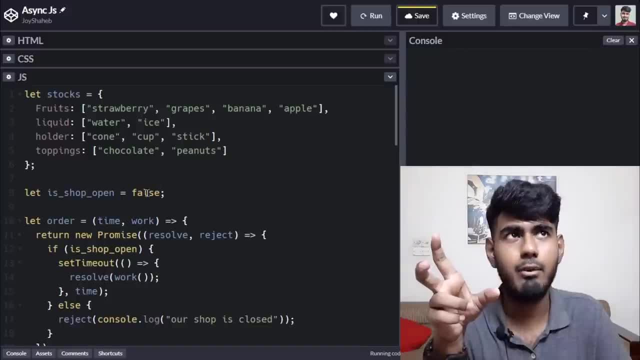 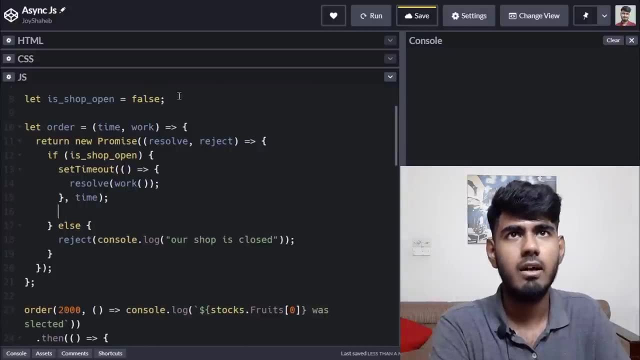 see what will happen theoretically, then we're gonna run this code. okay, let's see, we have this if statement over here, it will run when the variable is true, but it is false, which means our shop is closed. look at here else: reject, our shop is closed, so false. and then this: 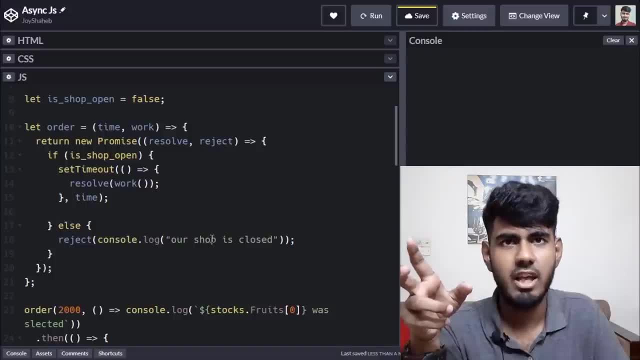 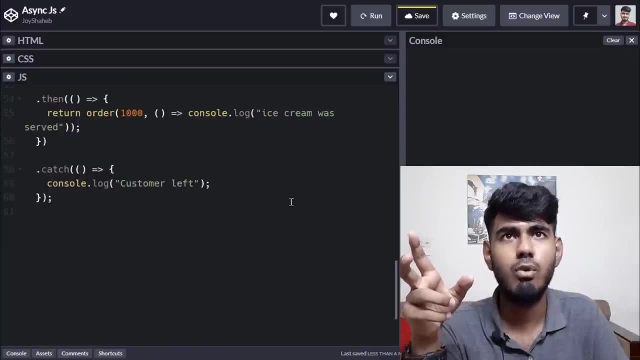 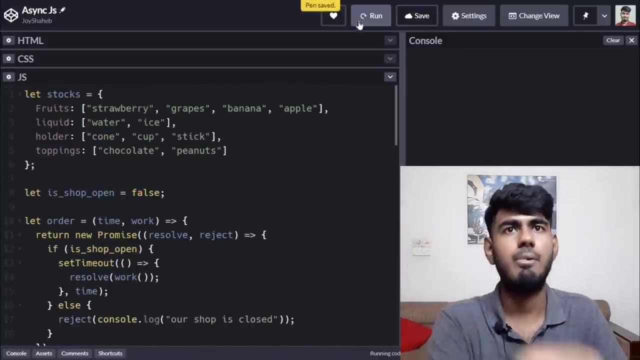 this code will be run first, and then at the very bottom we have this catch. then this line of code will run and these things will not run. this all then, then then it will not run. let's do a test, run it and let's see what happens. okay, so our shop is closed. the first thing we're gonna get. 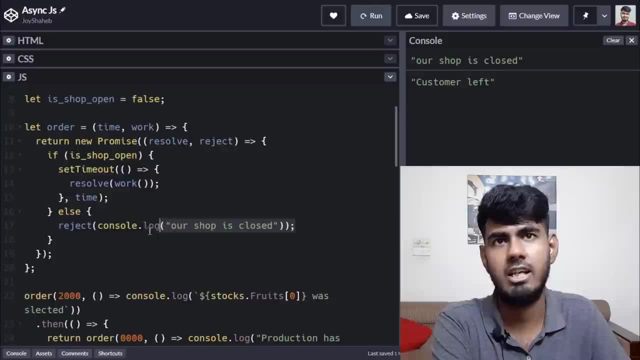 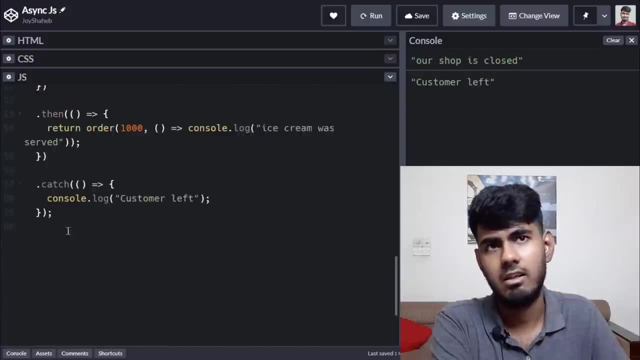 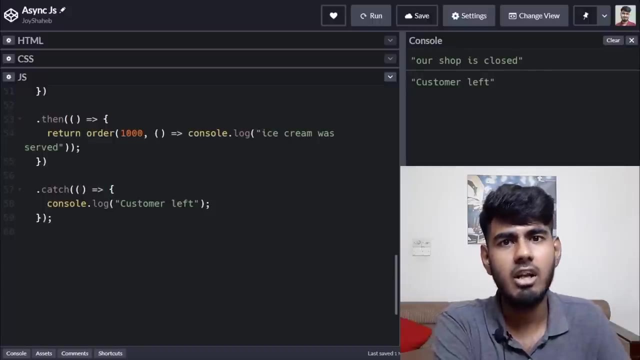 is: our shop is closed. look at this message over here inside this reject statement: look, our shop is closed. and then at the very bottom, look at this: this catch handler: customer left. we're very sorry, this left, they left us. look the customer left. we're not gonna make the money. we can't buy the lambo, we're very sorry. all right then, i hope you. 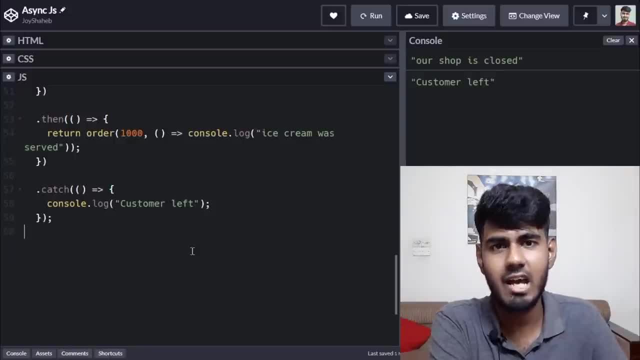 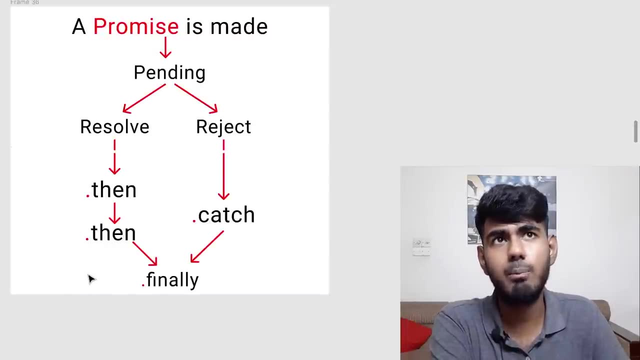 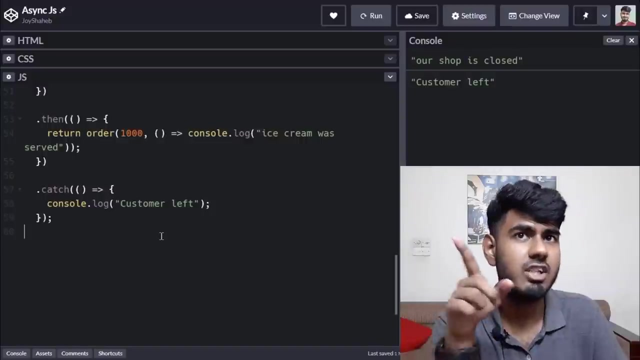 understood this catch. i mean the error handling part with the catch handler. let's understand this. finally, handler: i told you earlier that is, this will run whether our promise is resolved or rejected. it will run anyways. okay, now let's look at this example, but first remove this semicolon, otherwise it's not gonna work. okay, then dot finally, like: 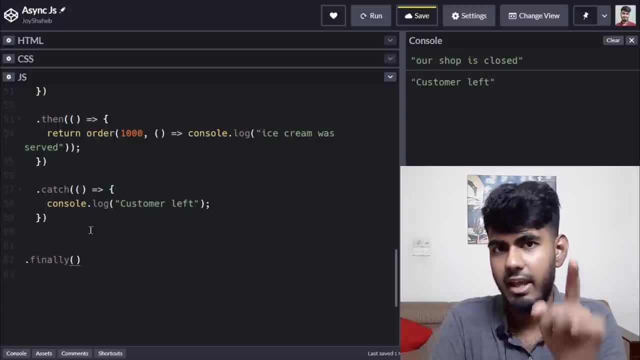 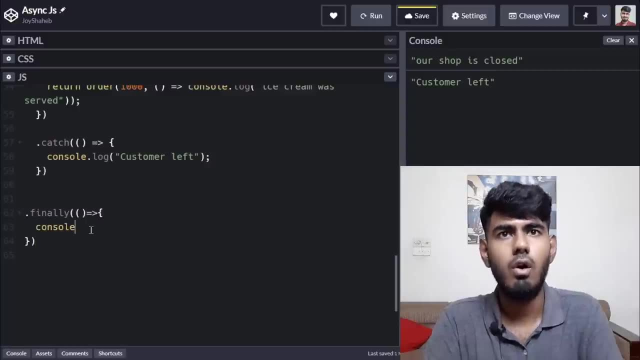 this, and inside over here we're gonna write: what tell me arrow function. okay. like this: equal to this sign: curly braces. like this, we're gonna write console dot log like this. and inside over here we're gonna write: our shop is closed. now let's write day ended. shop is closed, okay, day ended. 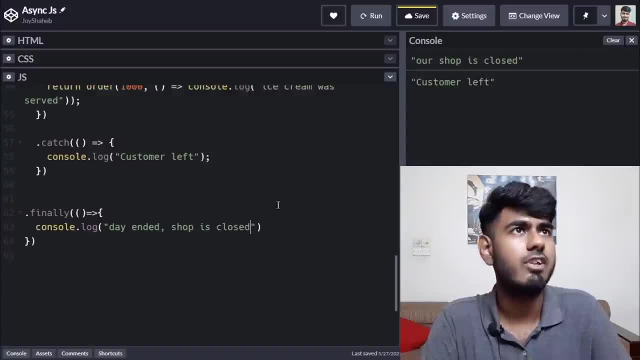 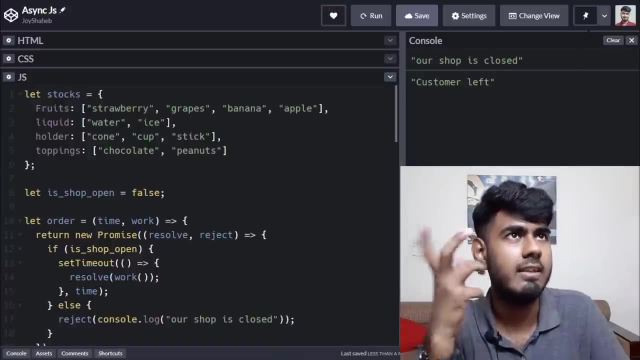 is closed like this. okay, let's save it. do you remember what state is it in? our shop is closed, which is false. okay, let's run it in this way. you can also run it in true. let's see, look, our shop is closed. this message is coming from this reject statement over here. customer left is coming from. 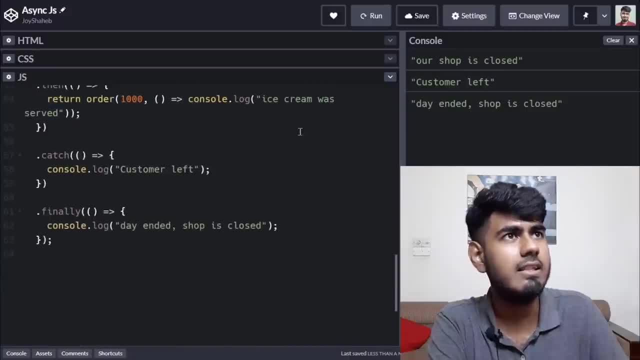 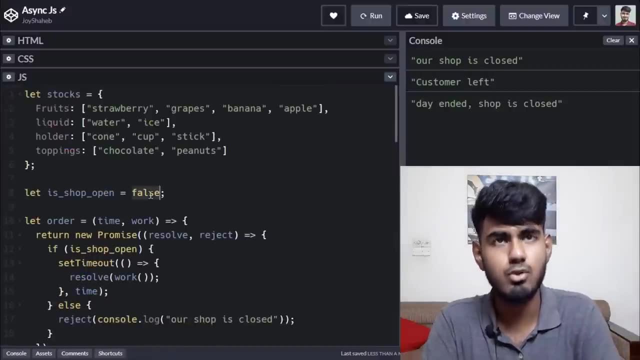 this statement over here. this catch handler okay and this day ended, shop is closed- is coming from this finally handler. let's set it to true and let's see what will actually happen with our finally handler. okay, control s run it. uh, clear the console and let's see what happens. okay, we got the statement then. 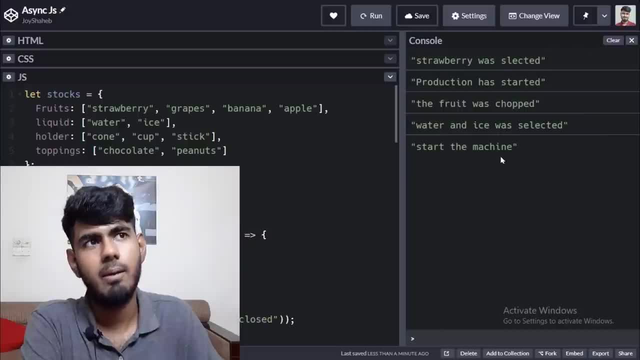 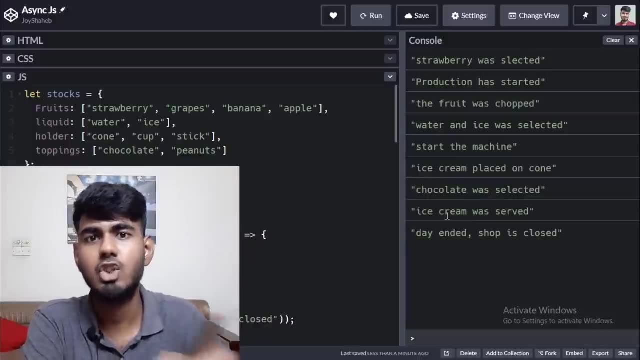 this, then water and ice added, then this: um, ice cream place in cone, then my favorite part is the chocolate, yay, and then ice cream was served. day ended. shop is closed. look at this. look look at the very end. day ended. shop is closed. it's coming from this, finally, handler. so what did you understand? 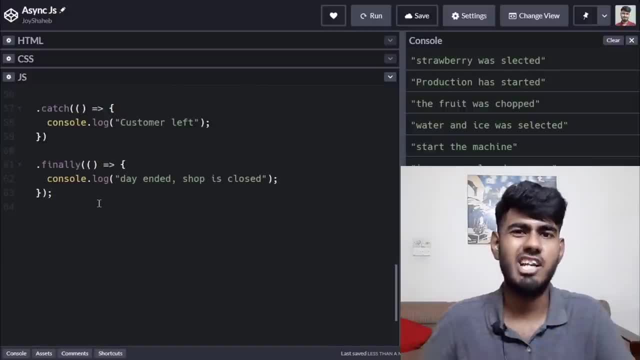 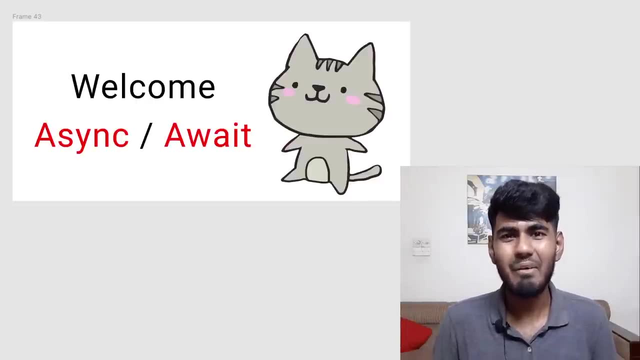 it will run whether our promise is resolved or rejected. and with that we finished our discussion. with promises, everyone, please welcome async await. yay, so this is actually proclaimed to be a better way to write promises. let's go and dissect async await, but first you take a break because you 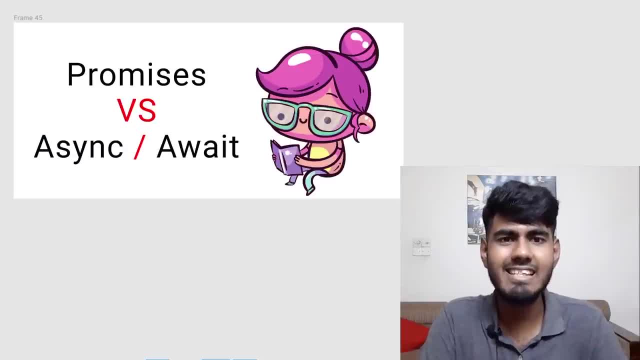 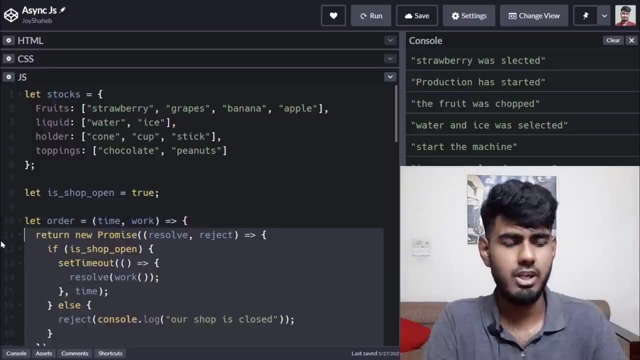 really deserve a break. in order to understand the async await, first of all you need to know the difference between the promises and the async await. let's look at an example. come back to vs code. i mean code pen. you delete everything except our um this part okay. keep the shop and the stocks okay. now in the promises part, how did we make? 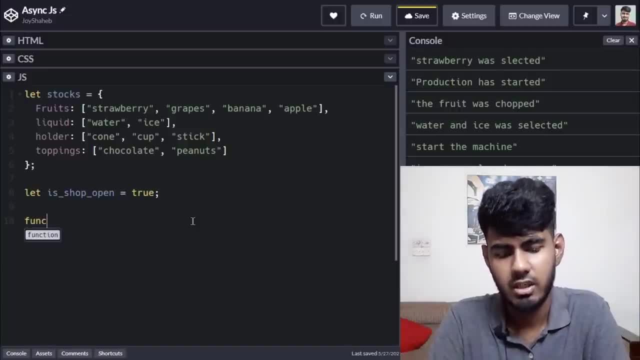 a promise like this: look, function. uh, let's name it: order okay. order like this okay. no, we actually didn't write it like this, my bad, we wrote it in the arrow way. function, i mean the arrow function. so let order equal to this, equal to um arrow sign, curly braces like this: and in order to make the 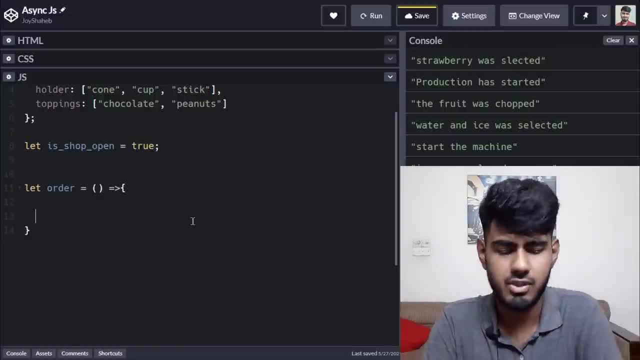 promise. we wrote what return new promise, return new, oh my bad, new capital letter: p r o m i s c promise, like this. and then inside these brackets we wrote another um arrow function like this: okay. and inside here we wrote resolve reject, like this: okay. and then inside over here, what we wrote: if statement okay, then this one, and. 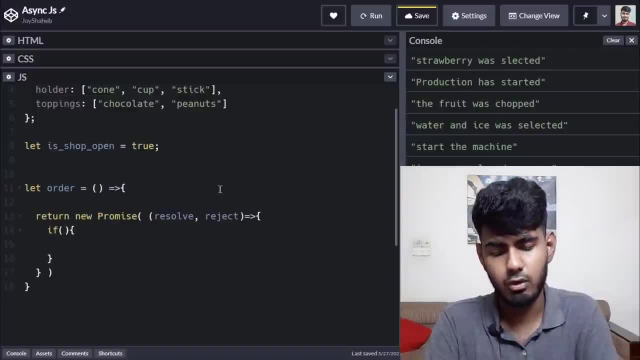 inside over here. what did we write? what did we write? we wrote the results like this: okay, look at this. and over the else statement, what did we write? okay, then we wrote the reject over here. my bad, we checked like this: okay, we wrote it like this: this was the promise, but how do we write it? 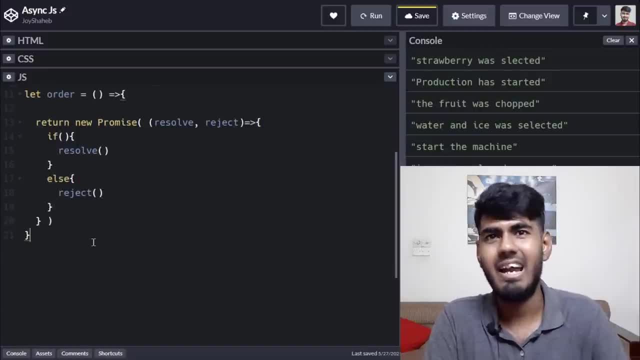 okay, so we have to write the async await. look at this, look, look. we write first of all the async keyword. what the async keyword? async- okay, you write the function order. okay, this, and then the curly braces, and there we go. we made ourselves a promise. how simple is that. but wait, the story. 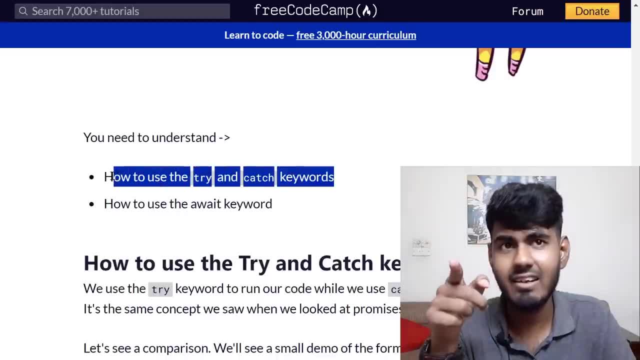 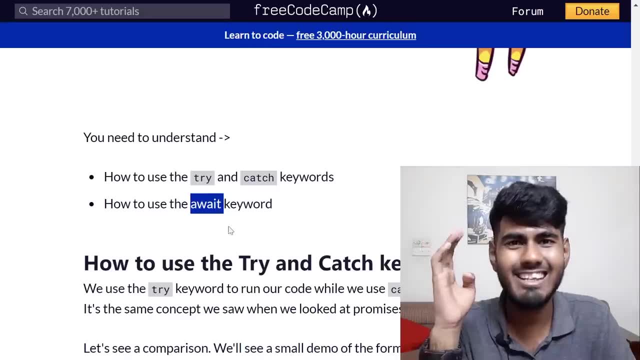 doesn't end here. we need to understand two more things: the try catch handler and how to use the await keyword. so this is the async keyword. we need to understand the await keyword. let's dive in now. let's come back to our code pen and understand the difference between the. 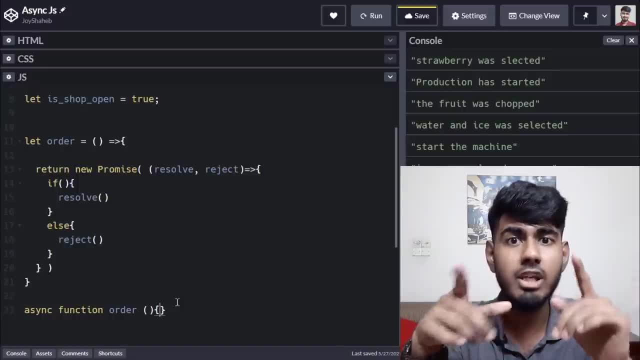 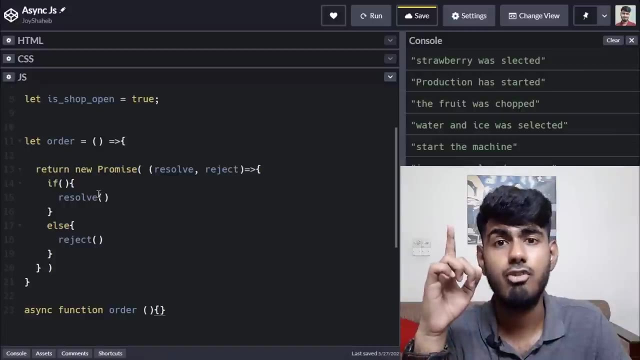 promise and our async await. only then we can understand the try catch. okay, come over here and see this if and else statement. what did we write? how did we make the promise? we made this promise like this: first of all, we wrote the function over here and then return new promise. then 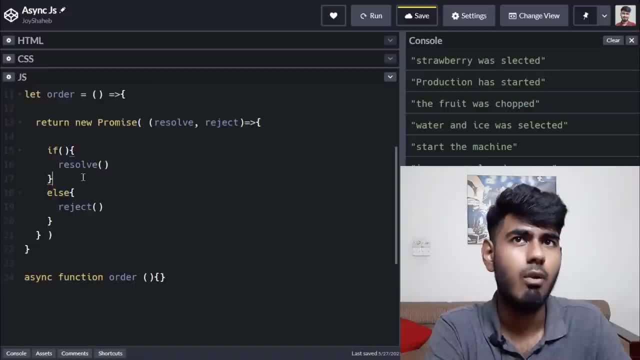 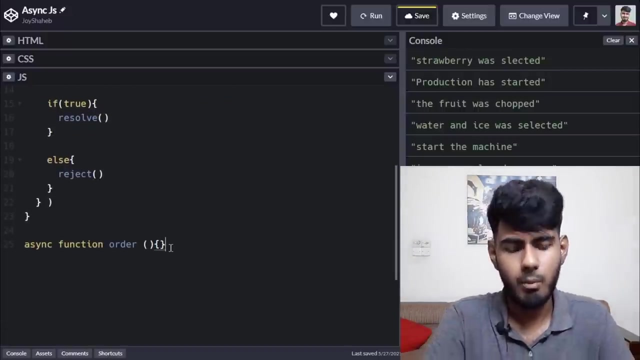 resolve, reject. and then we wrote the if statement, which is: if this is true, we wrote this, t-r-e-e true, okay, then it's gonna resolve it. if it is not true, then it's gonna reject it. like this: this is how we make the promise. and then what did we do? okay, we comment this like this. let me. 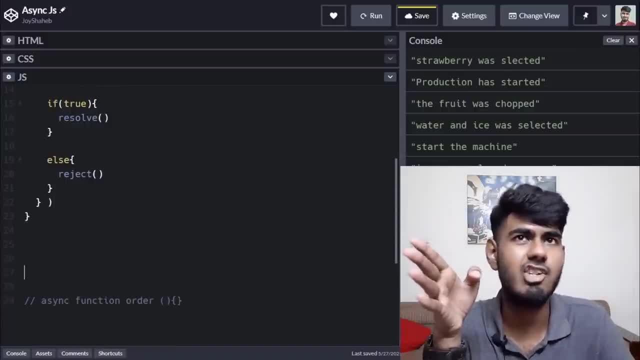 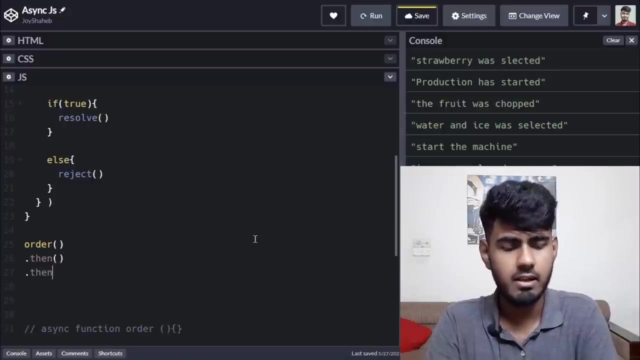 actually finish with the promise part, then we're gonna come to the async javascript part, i mean async await part. this is the order, right? how did we write it? order, okay, order. this is our first start. and then what did you write? dot? then okay, dot, then dot. then oh, sorry my bad. and then what? 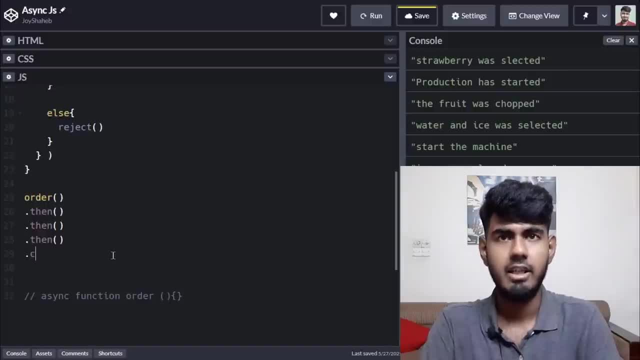 did you write? and then we wrote dot catch, catch t c, c a t c- oh, i forgot my bad. c a t c, h catch handler and then the dot finally handler. okay, so this will work when- what if our promise was resolved? this will work. when it is rejected, this will work. anyways, it's still gonna work, even it was. 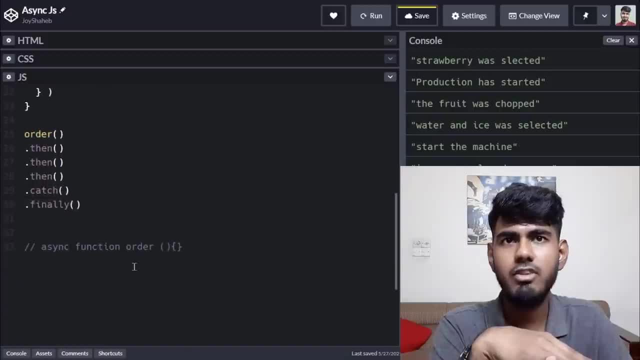 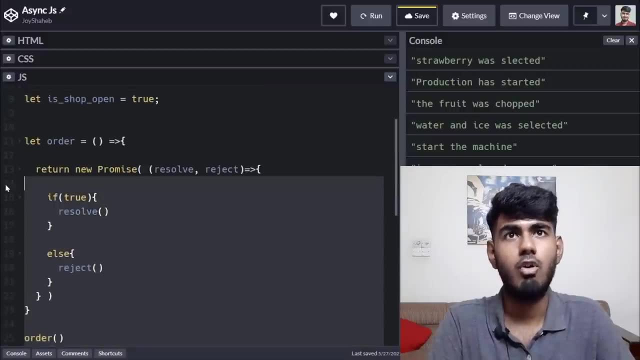 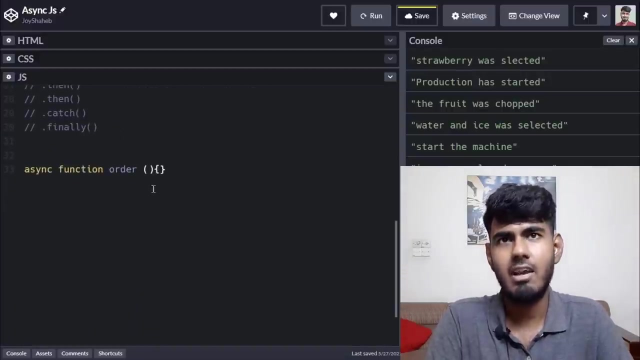 resolved or rejected. but in terms of this, um, async await. let's actually test it with this how this works. okay, don't worry about this one. let's comment this. we're gonna return over here. okay, don't worry, comment this like this and come over here. so first thing is you know if you want to declare. 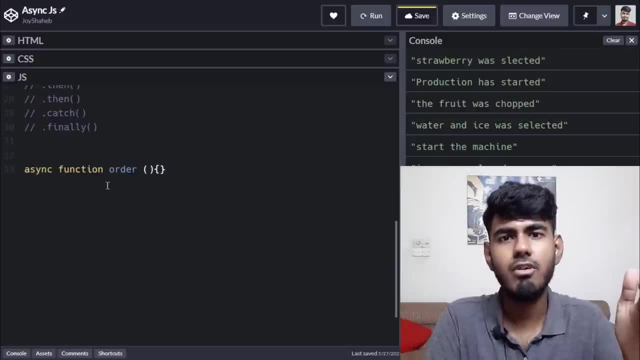 i mean, if you want to work with promises in the async await world, then what we have to do is we have to declare this async word before the function i showed you a little while ago, right, and then inside, over here, you have three options. i mean three things to write: try, catch and finally, what tell me, try catch. finally, over here, we wrote what. 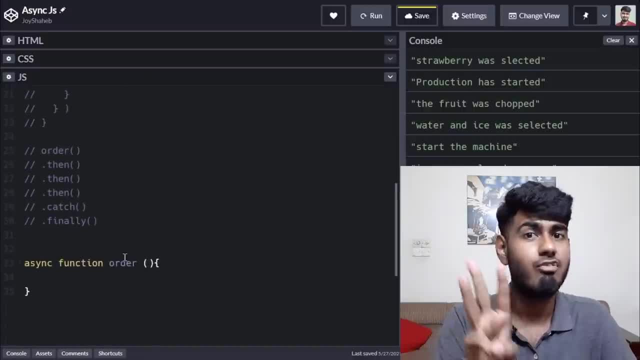 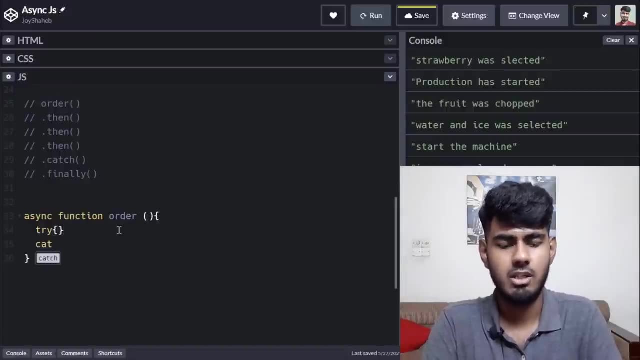 else statement. and over here we're gonna write try, catch, finally, follow me. you write try over here: okay, curly braces, like this. and then you're gonna write the catch, okay and brackets. over here you write error, okay, curly braces. and over here you write finally, like this: okay, then, curly braces. 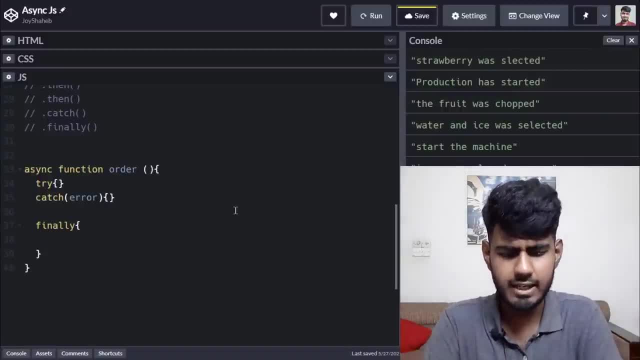 so what does this finally? does it? it runs code anyways. okay, let's write it. okay, don't worry, we're gonna test it. okay, consolelog, um, run code any way. okay, inside this catch handler. I mean, let's start with the try. okay, let's create a fake problem. what problem? fake problem over here we're. 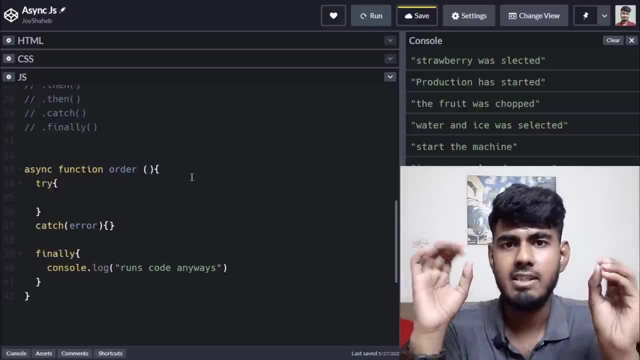 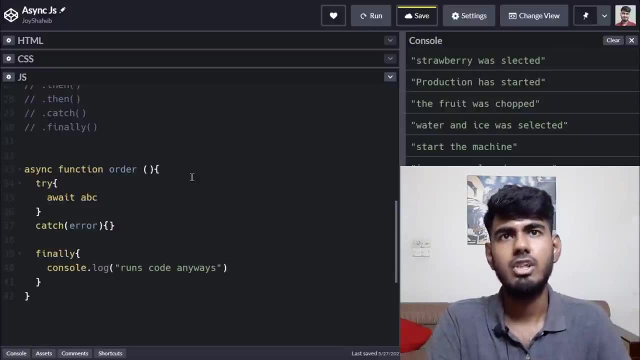 gonna write away. don't worry about the await keyword. I'm gonna discuss in detail about this await keyword. okay, it's coming. wait, you write away ABC. so this ABC is actually pointing out to a function which doesn't exist, and I still wrote it because it's a fake function. what function? fake function, okay, so 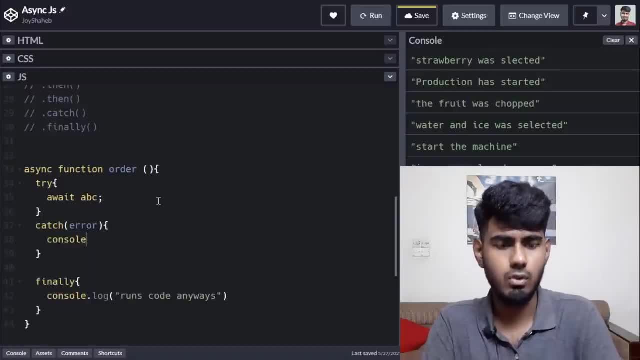 inside this catch handler. what we're gonna write is console the log like this, and over here we're gonna write: ABC doesn't exist, exist. okay, and this error is actually written like this: comma error. okay, for now we don't need this error part, but we're just keeping it over here as it is. we just want to work. 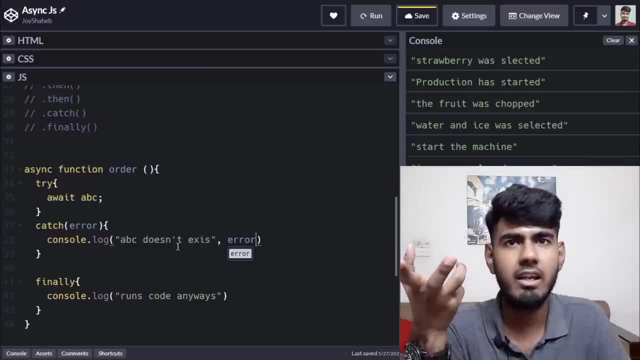 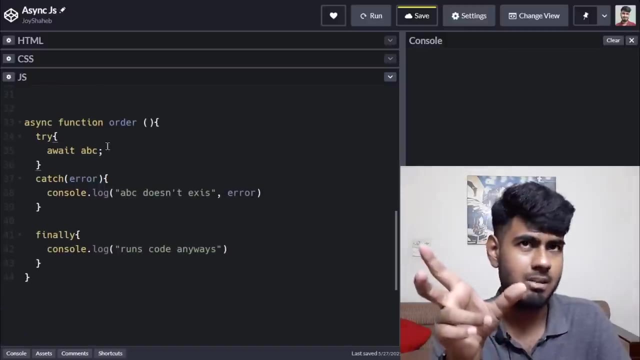 with our try, catch this console log and this finally, and this finally, handler, in order to understand the main theory of the async await. okay, so you clear the console here. as I told you earlier, this await ABC. I mean this ABC part doesn't exist. look at the entire code field. nothing exists which is named ABC, right? 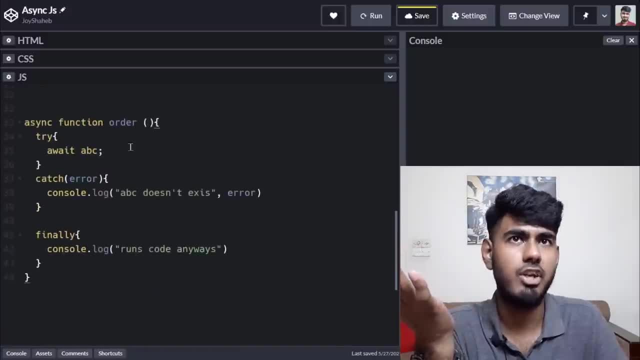 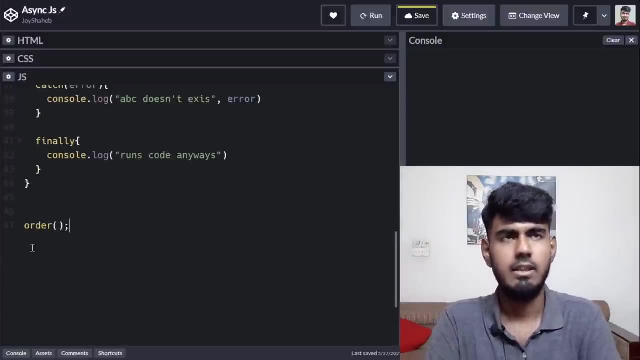 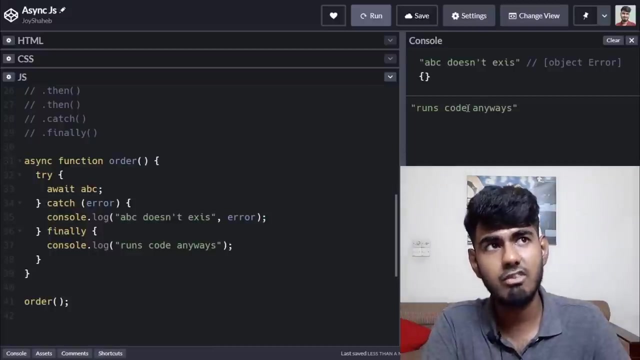 so, in order to run this, first of all you need to provoke it, like by saying order, and the very bottom over here, right, order, okay, my bad, sorry, like this control s and let's run it and let's see what happens. there we go, we got the message. first of all, ABC doesn't. 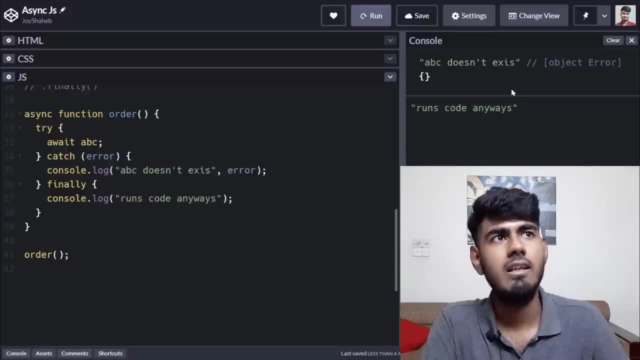 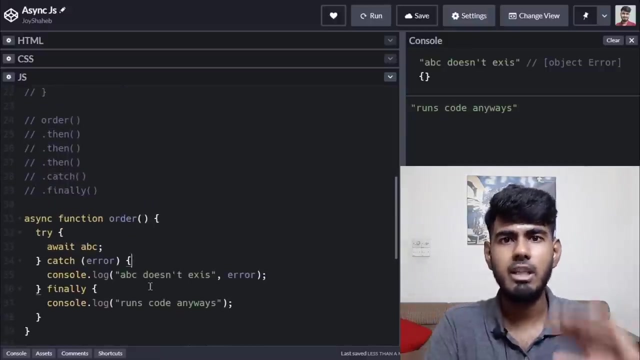 exist because we don't have anything named ABC, then um it, then we have runs code anyways. look at this, the finally handler. do you remember this? finally, from the promises, this is over here. it will run code anyways. by the way, do you remember this? handlers, this. then catch finally handlers. you can. 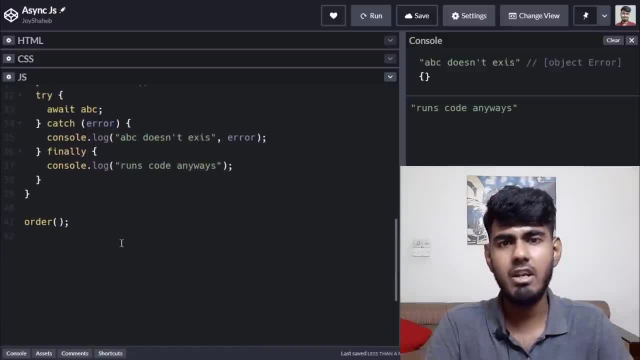 also use them inside. I mean outside the async await system as well. let me show you a demo. okay, you write at the bottom of the order, after removing that semicolon dot, then like this: okay, brackets, then create a arrow function like this, and over here you write console. 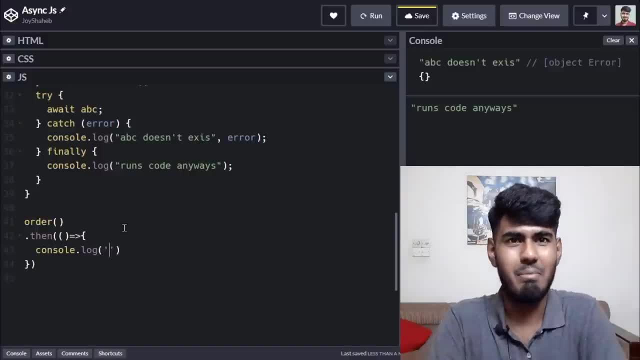 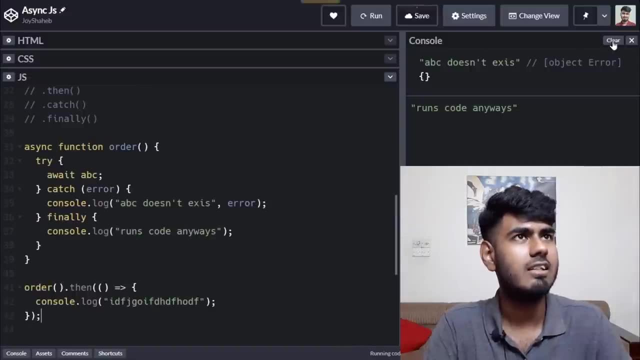 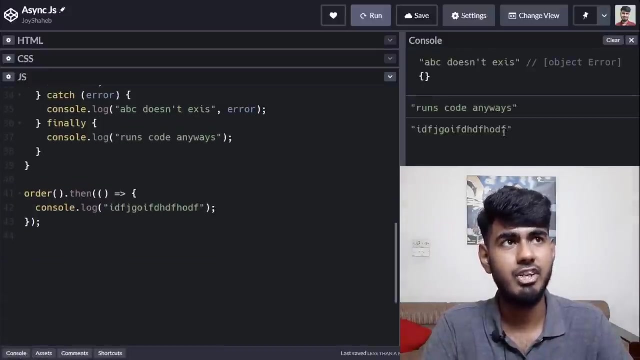 dot log then write anything you wished. I'm gonna write my bad. i don't. i cannot think anything of good right now. ctrl s clear this: run it like this. ah, there we go. we have got that. then, handler, it is printing over here. okay, first of all, we got that. 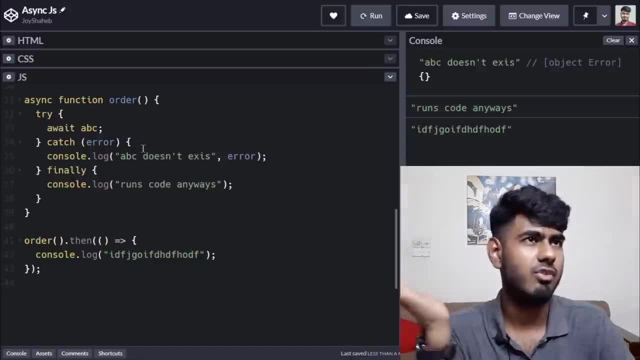 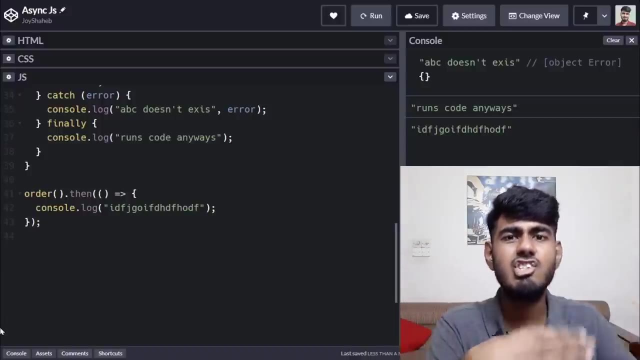 error. and then the finally, it's gonna run anyways. okay, so that is over here. and then the then what will happen after our promise is resolved? it's gonna do this part over here and you can also use those. then cats, finally, etc. after here, it is the chaining part. okay, i hope you understood. 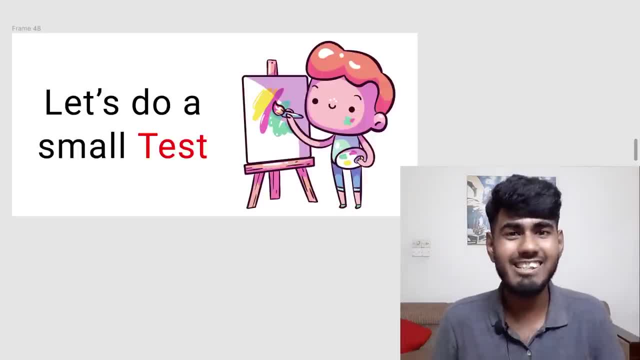 this far. now let's do a small test and understand the await keyword. let's say that i am the chef of the restaurant. okay, just look at me. i am the chef of the restaurant. okay, i make an ice cream. i took the order from the customer and i'm making ice cream. okay, my bad, sorry. okay, so i'm making ice. 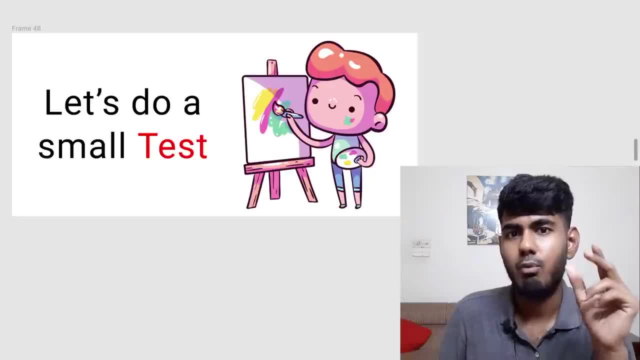 cream over here. but i've then realized that my customer didn't tell me which stopping work he like. so i have to go outside the kitchen, ask the customer: sir, which topping topping would you like? chocolate or peanut? then he's gonna give me the order. give me chocolate, and then i have. 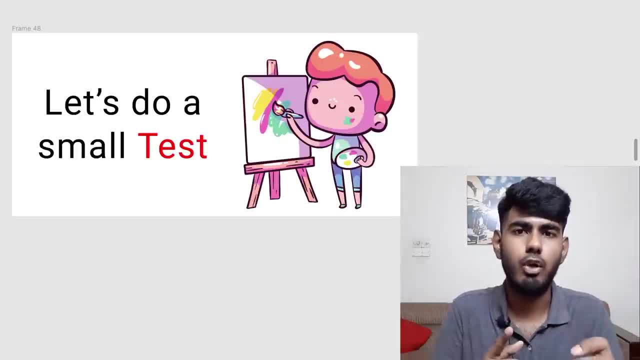 to return to the kitchen and start working. look how the process is working. i am going outside, which means that the kitchen is being stopped completely. without the chef, the kitchen doesn't work. but realize this: that there are other employees at the restaurant. who is working? who is? 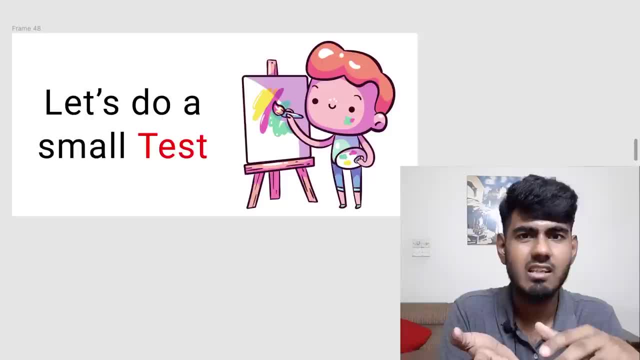 cleaning the tables, cleaning the dishes, taking orders, etc. everything else except the kitchen is working. this is where we use the await keyword. let's do a test and understand about this await keyword in details. let's start now. come back to code pen. now come back to code pen and remove. 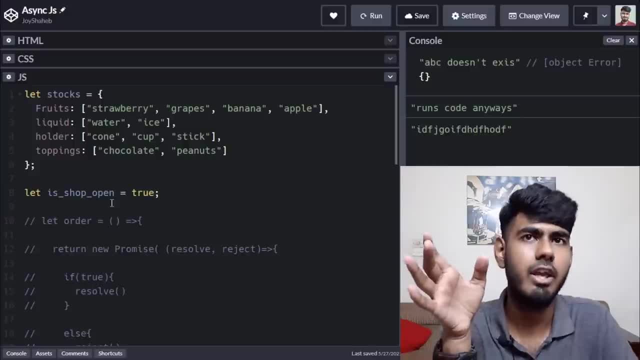 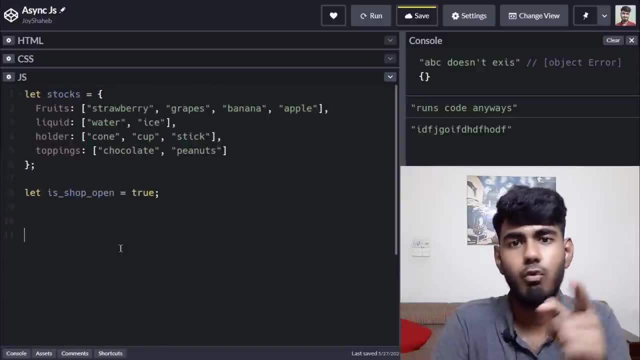 everything except the stocks and the east shop open. okay, remove everything like this. goodbye forever. okay. now what we're gonna do is we're gonna create a function. what a function. which one arrow function. okay, let let's write toppings choice, okay. which will ask the customer cell: which topping would you love? okay, equal to my bad. equal to. 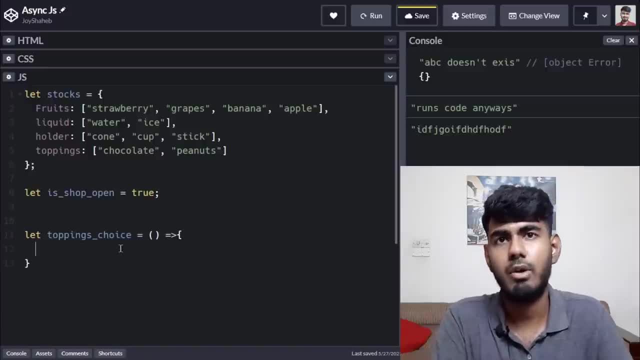 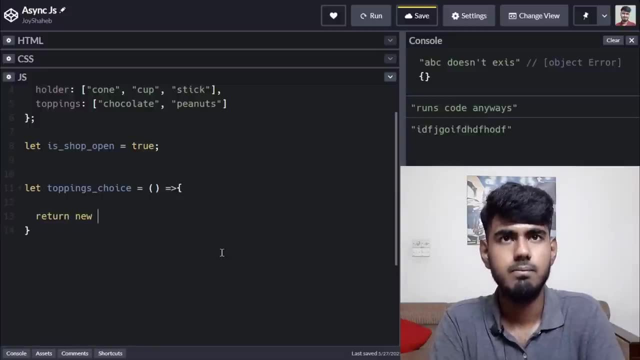 brackets this sign, which is the arrow sign, and inside, over here, we're gonna make an arrow sign, and inside, over here, we're gonna make an arrow sign, and inside, over here, we're gonna make an new promise. what new promise? okay, so return new promise like this, and over here we're gonna write. 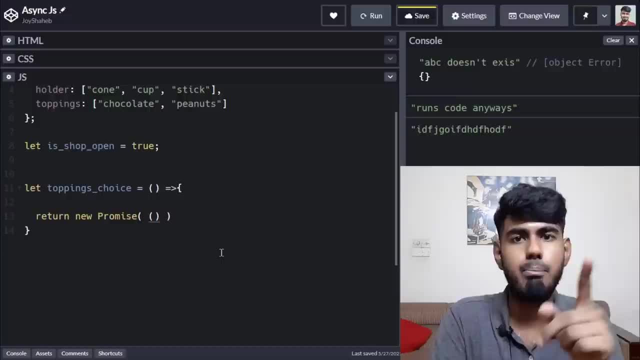 resolve, reject. don't worry, i'm coming on, the async await part. okay, so equal to arrow sign, curly braces and over here what we're gonna write. come on, tell me: resolve, reject, resolve, my bad, we check like this. okay, now over here, what are we gonna do? 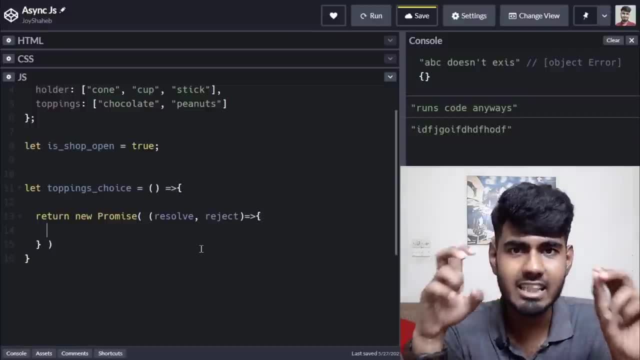 okay, now over here, what are we gonna do? we're gonna create a set timeout. let's say that the we're gonna create a set timeout. let's say that the we're gonna create a set timeout. let's say that the asking process takes how many seconds? three: 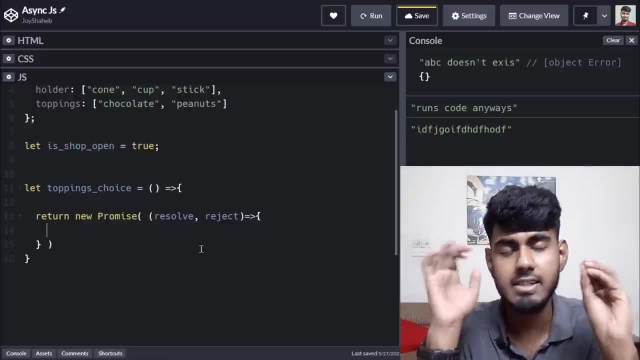 asking process takes how many seconds. three asking process takes how many seconds three seconds. how many three seconds. okay, in order seconds. how many three seconds. okay, in order seconds. how many three seconds. okay, in order to do that, we're gonna write set timeout. to do that, we're gonna write set timeout. 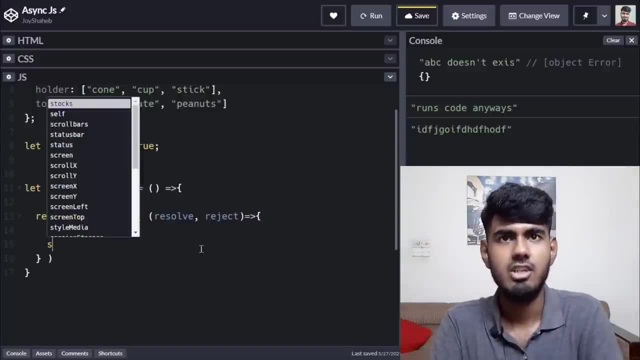 to do that. we're gonna write set timeout: okay for three seconds. so write set time: okay for three seconds. so write set timeout okay for three seconds. so write set timeout like this: okay, and then what we have to. like this: okay, and then what we have to. 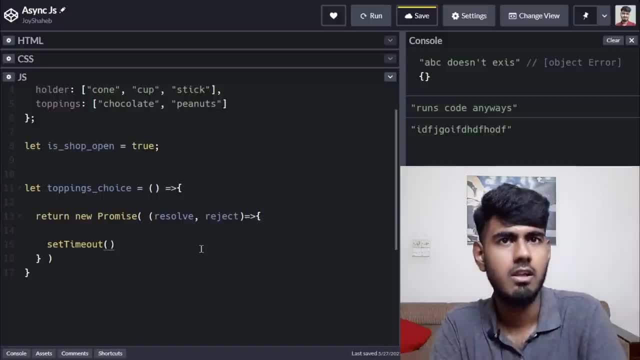 like this: okay, and then what we have to write is: come on, tell me arrow function. write is: come on, tell me arrow function. okay, like this. and then we're gonna set the time. how many seconds? three seconds, three, one, two, three, all right now, inside, over here, we're gonna write consolelog, consolelog. over here, we're gonna. 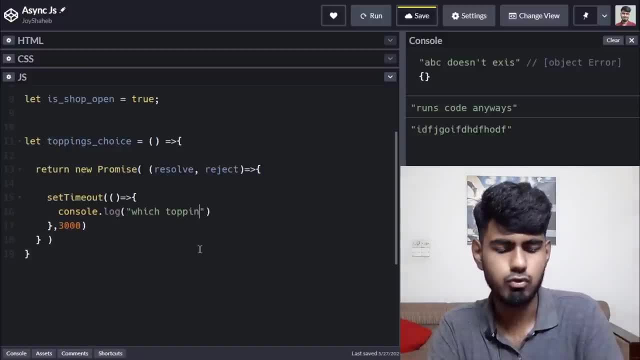 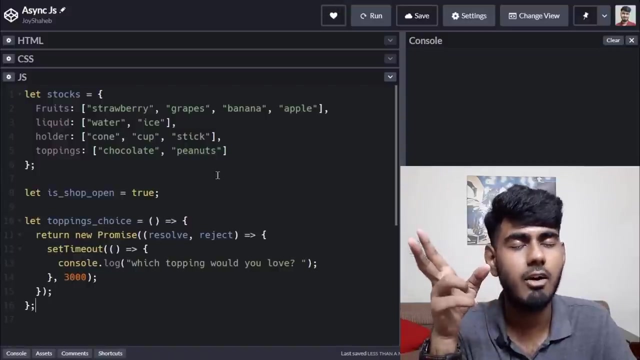 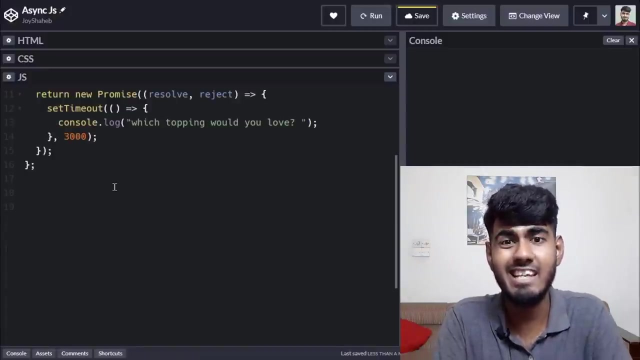 write: which topping would you love? oh, my bad, like this. remove this console from here. clear, okay, control s now. we made a small promise that we have to go outside the kitchen ask our customer what would he love to have as a topping? now, at the very bottom, what we're gonna create is is function async. 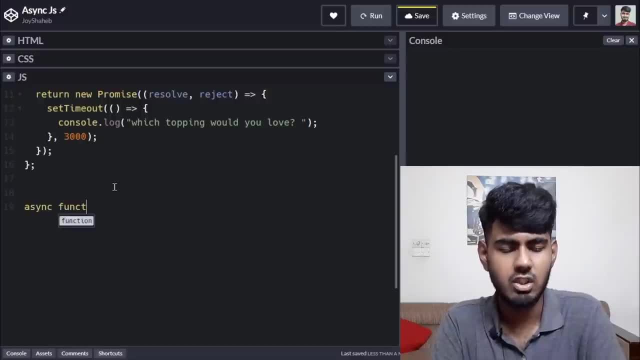 function. async function. um, we're gonna write what brackets? oh, we also have to give it a name. we're gonna name it kitchen k-i-t-c-h-e-n. kitchen over here, and then curly braces over here, like this: now follow along with me. we're gonna write consolelog five times: a, b, c, d, e, like this. okay, consolelog. okay, like this: 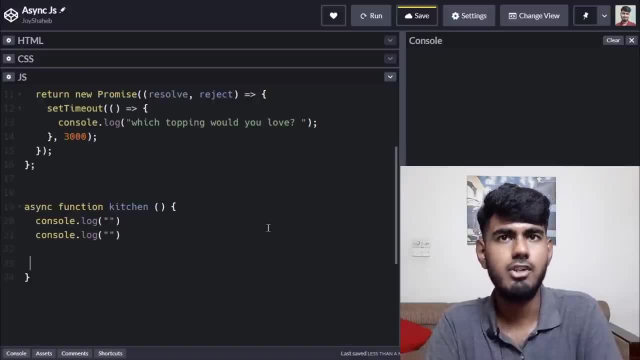 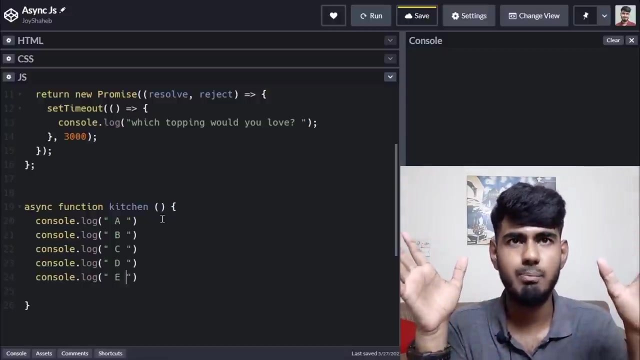 control c one, oh my bad. two, three, four, five. okay, now we're gonna write over here a, don't worry, i'm gonna explain that why i wrote a, b, c, d of my bad, b. okay, can c, b. okay, we're gonna write c, a and d, then c and d s, which are ug t. 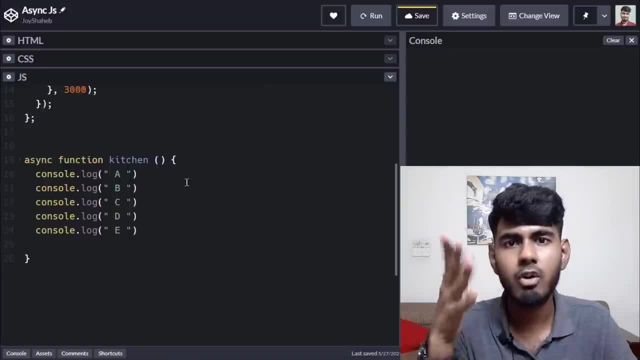 okay, now in the hdb, command again: rii, rii, e. okay, now what we are gonna do is: oh, let me actually explain why i wrote this: a, b, c, d, e and all this part. okay, the thing is, these are the steps. we're working the k— mean we are working at the kitchen. okay, we're making ice cream. we are following the steps one, two, three, four and the very middle. we just realized which topping would our customer love? okay, so we have to go outside the kitchen. outside the kitchen, ask him, sir, what do you love in the kitchen? what? ask him? what? ask him, sir, what do you love in the kitchen? why? 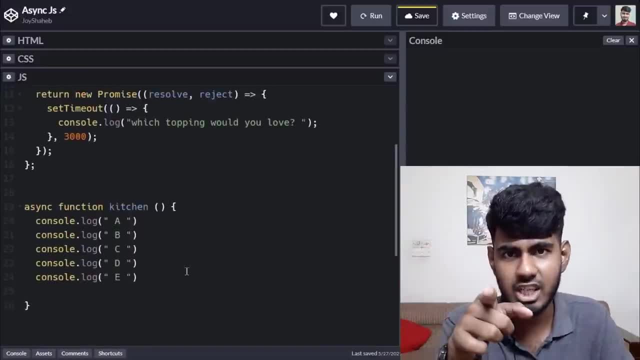 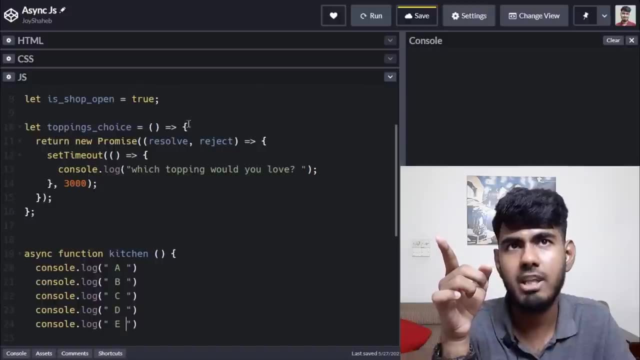 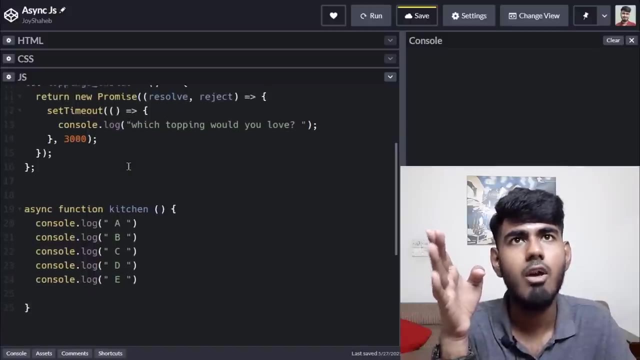 which you love to have. so this is our kitchen. we're inside, over here where, where we're inside this kitchen, we're working. now we need to go outside and come to this toppings choice, which is the where the customer is sitting. ask him: so what would you love to have? and then, once we have, 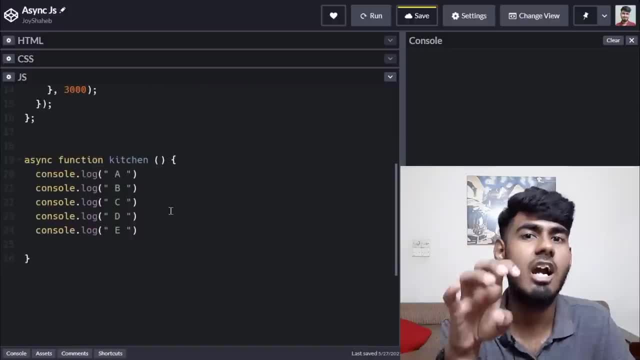 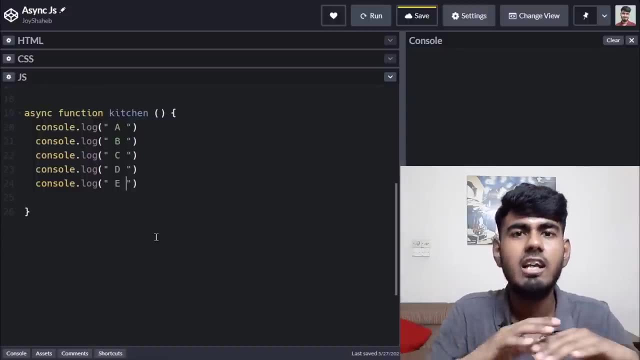 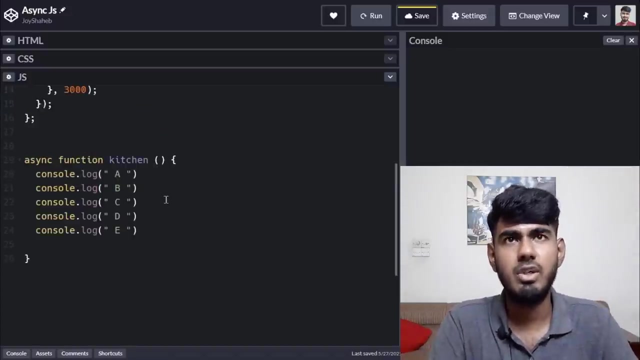 got the data, we're gonna come back to our kitchen, start working and then serve him. in the meantime, what will happen? others other works, like cleaning the dishes, cleaning the table, taking other customers orders will keep running. don't worry, i'm coming to that part. okay, now what you're. 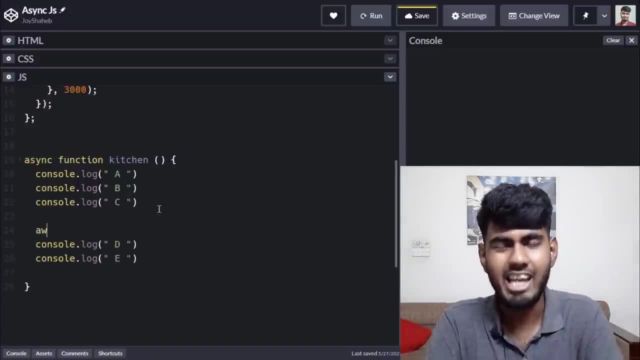 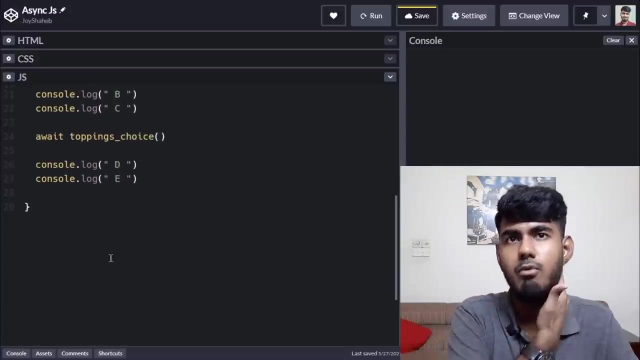 going to write is at the very middle over here. you're going to write: a wait, then what the name of this function? what is this? toppings choice: ctrl c, that one, ctrl v and then brackets- close it. and then what you're going to do is, in order to provoke this function we're going to come over at 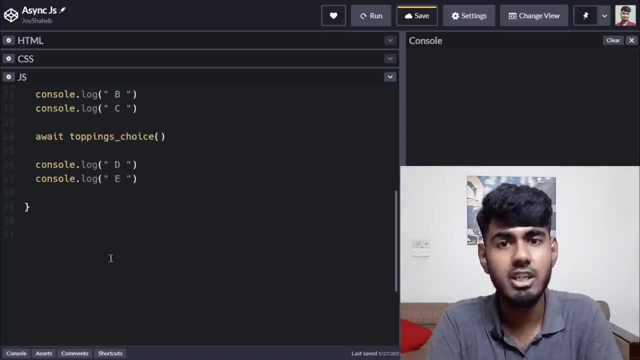 the very middle of this function, and then we're going to write a wait, and then we're going to come over at the very bottom, over here, you're going to write kitchen, what kitchen? kitchen, like this: okay, and then we're going to define other task which is happening except myself. i'm the 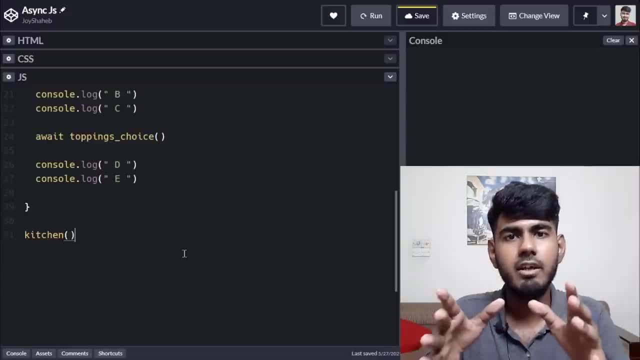 what i'm the chef, okay. other works are what cooking, i mean sorry, cleaning the dishes, cleaning the table, taking other orders, let's write them okay. console the log: um, cleaning my bad, cleaning the dishes. console the log like this control, i mean this one: ctrl c, ctrl c. then what? 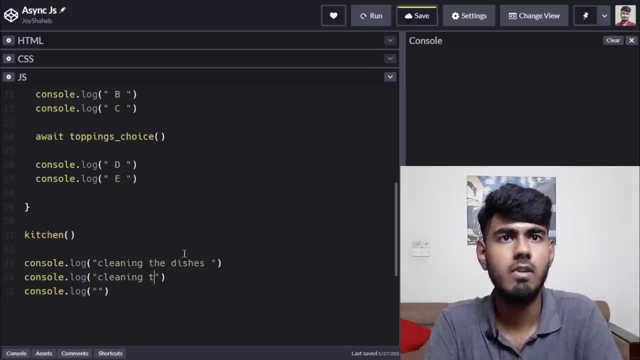 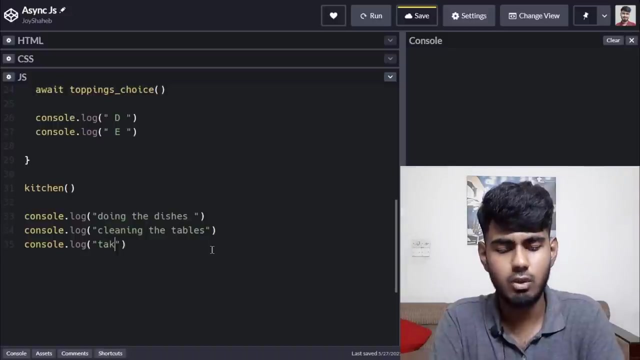 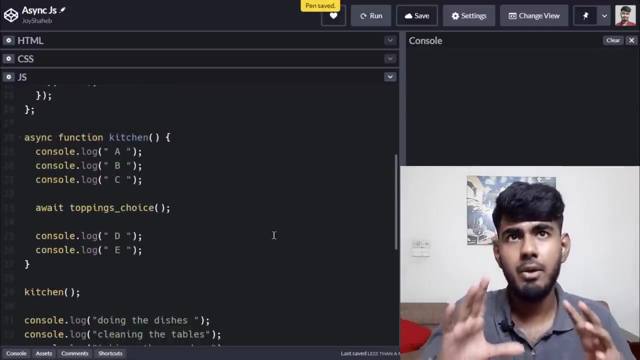 cleaning the tables. actually you write doing the dishes. it sounds good, i guess: doing the dishes, dishes, cleaning the table. and then at the bottom we're going to write taking others order. but ask question here also. okay, so here is the picture. so i'm here and i'm doing the picture in a quite stylish way, so you're not offering though on a big block. 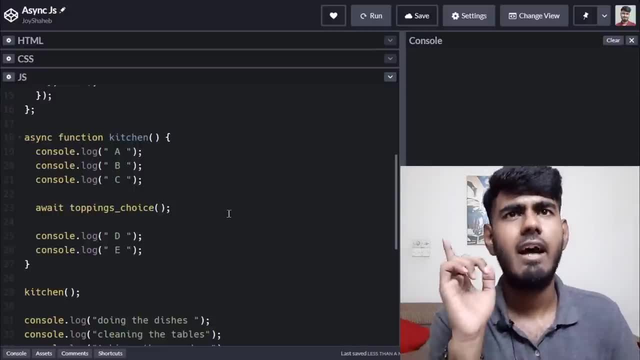 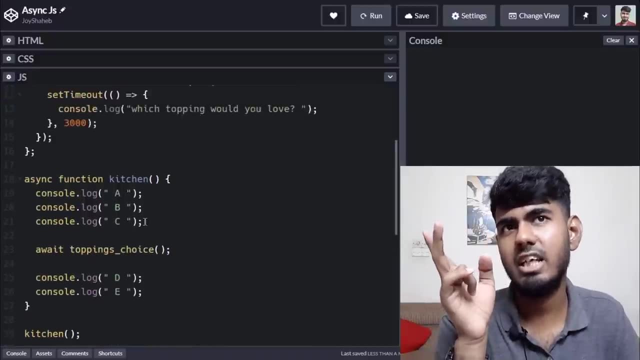 there's your phone number, there's your product, and if the answer is yes, let's go for the one more question again. yeah, let me give you a while, okay. ah, our автомобile cost? we're going to have the difference. ah, if we compare it with the 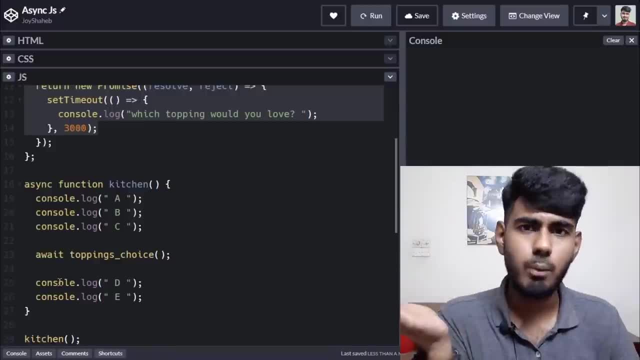 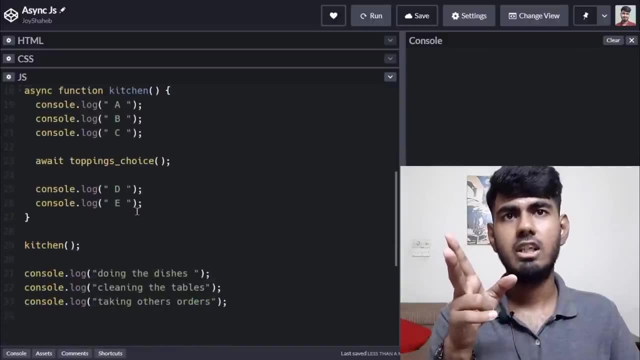 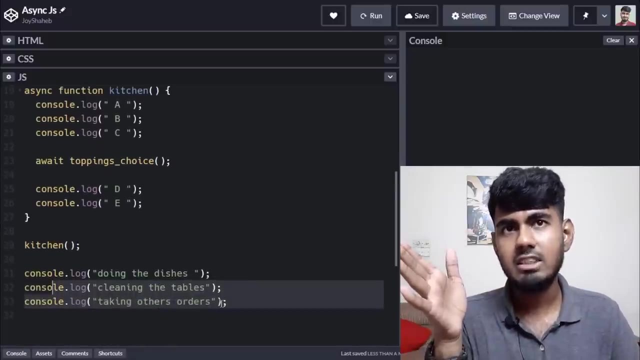 touristcole performance we're going to have a very nice将- is stopped, nothing is happening because the chef is outside and in the meantime, other work like this one will still happen, like doing the dishes, cleaning the table, taking others orders and, once I return to the kitchen, this to work D. 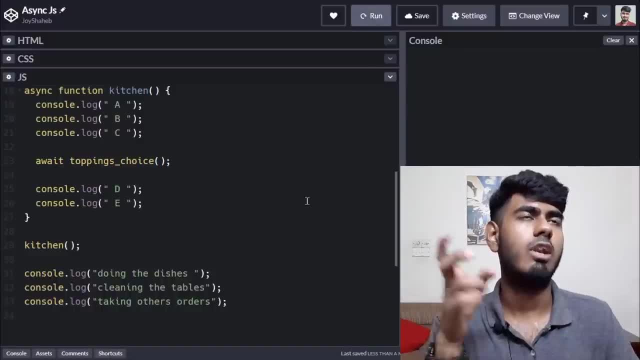 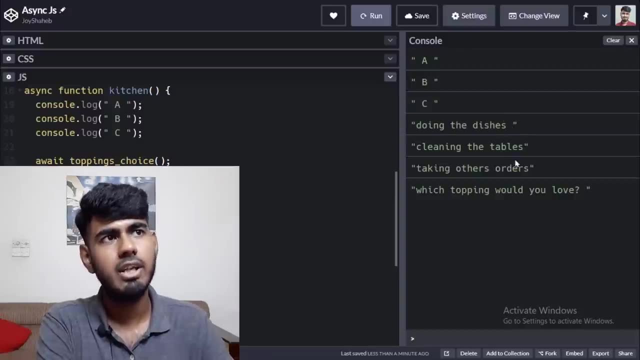 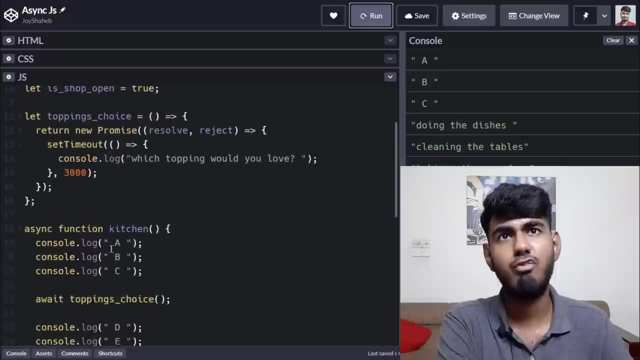 and E will work. let's run it and let's test what will happen. okay, look, a, B, C doing the dishes, cleaning the table, taking others orders. which topping would you love? oh, we didn't actually get the D and E. that's because I actually forgot something. I forgot to write the resolve over here and without writing the 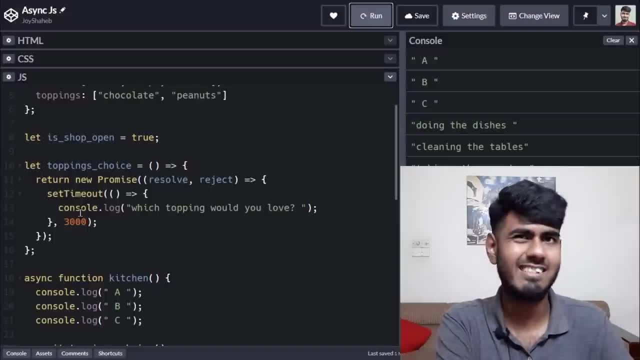 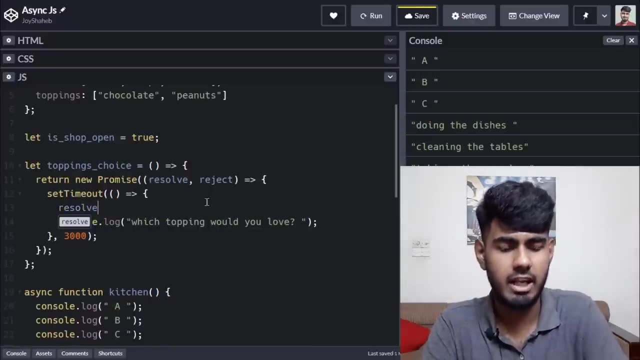 resolve. it's not gonna return our other tasks, okay, so come over here on the toppings choice, okay. or, and inside, over here, you're gonna write: we resolve, like this bracket, and inside the brackets, we're gonna play the game and we're gonna play the game, and we're gonna play the game, and. 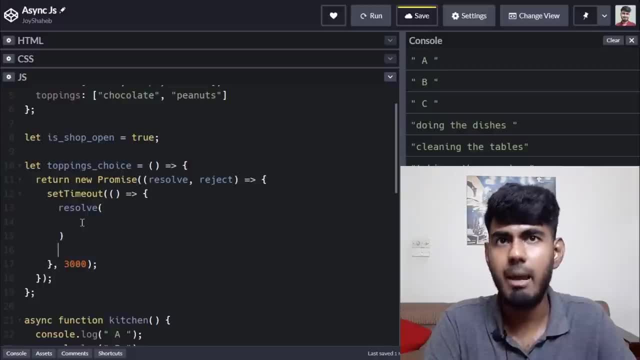 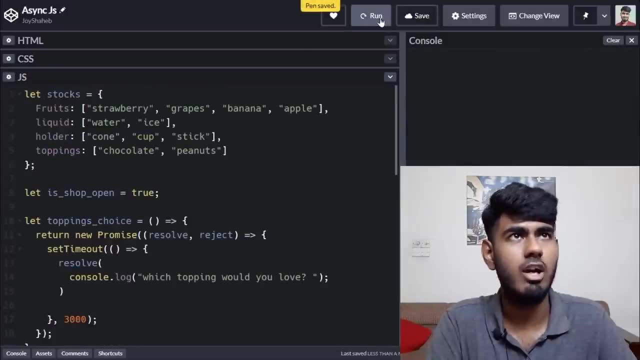 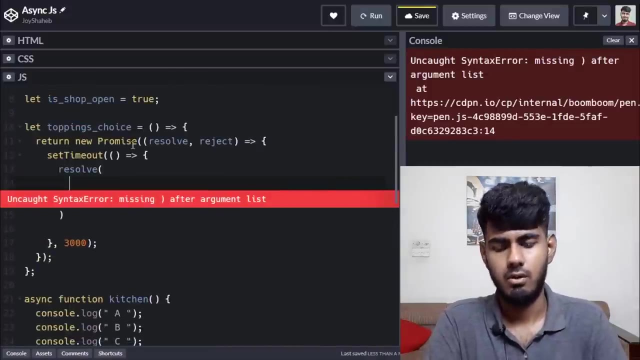 this console over here. okay, control X. my apologies, I actually forgot to write that part and control s. okay, now clear this and run the code and let's see what actually happens. okay, oh, I actually have an error. I don't know why, but let's check it out, okay. console log: which topping do my bad. 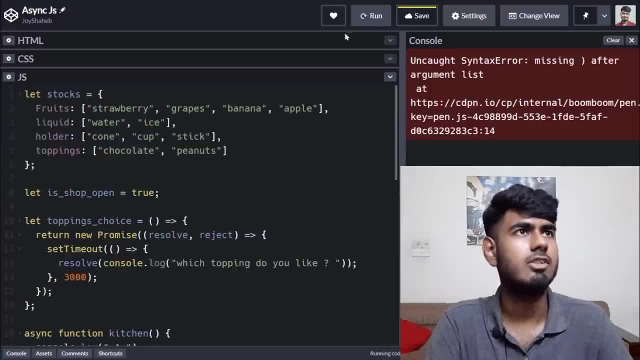 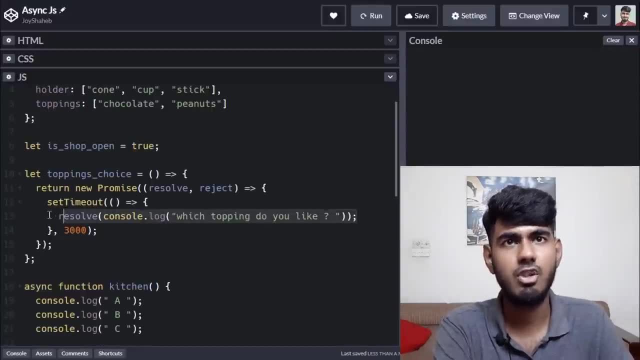 like: okay, like this control s. let's see what happens right now. clear the console like this: now you can see that we have fixed our error over here, we have written the resolve over here and we have to replace the console log inside this line over here. now it's gonna work perfectly fine. let's run the code and see what. 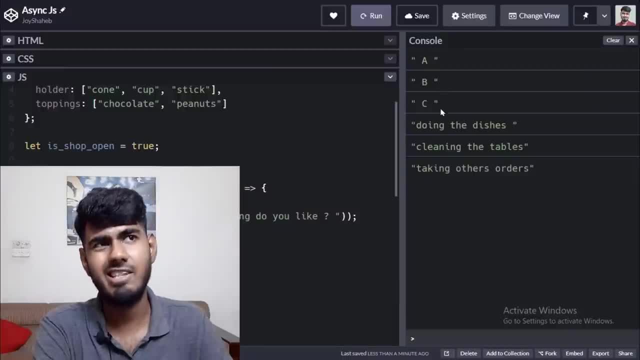 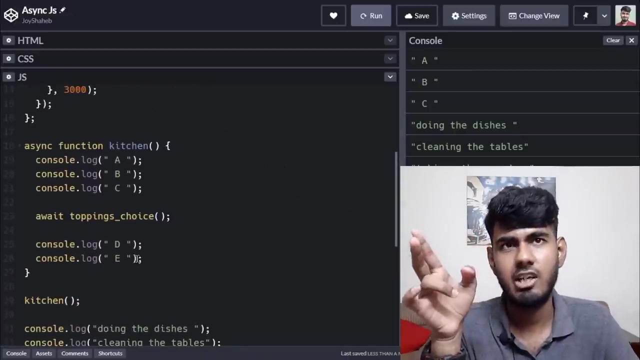 happens. there we go, we have ABC doing the dishes, killing the tables, taking others orders- which topping do you like? and then we have other works. what is happening? let me explain again. so what is happening? look here in the kitchen. I am working in the kitchen. where am I working in the kitchen? so these three 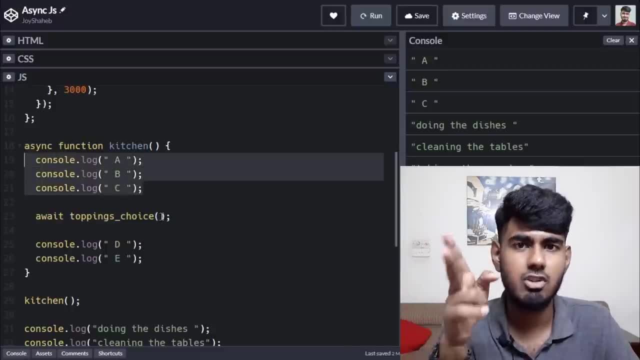 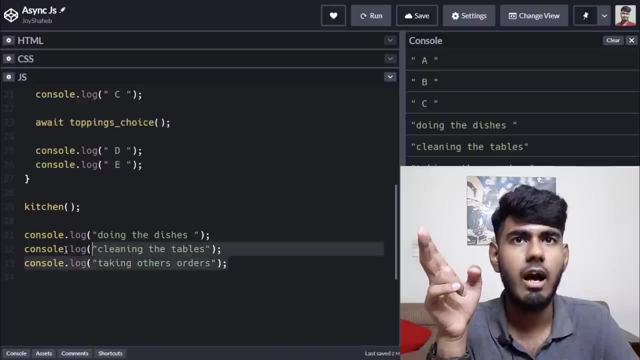 tasks are done, then I remember what topping does my customer likes. so I am going outside and asking him. in the meantime, others are working. look, other people are working over here. if there was hundred tasks they would have, they would have been working on those tasks. okay, so once this tax are done in the 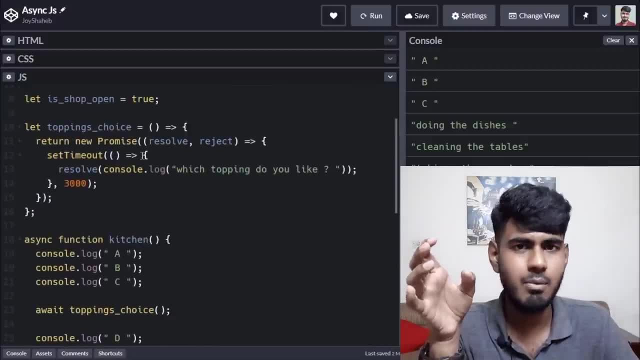 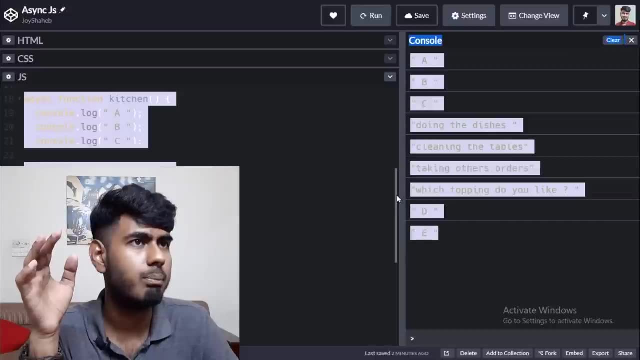 meantime, what I'm going to do is I'm going to go outside and I'm going to the kitchen and I started working. then D and E is completed on this bottom over here. you can see that. I hope you understood the await keyword. I hope you understood the resolve keyword. let's reopen our shop and welcome customers. 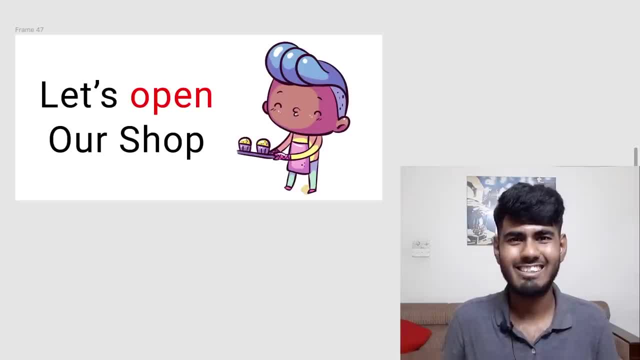 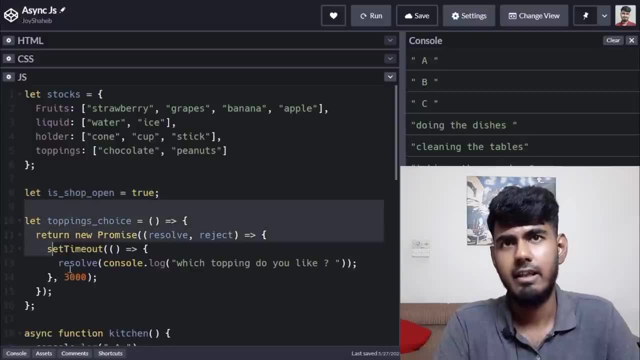